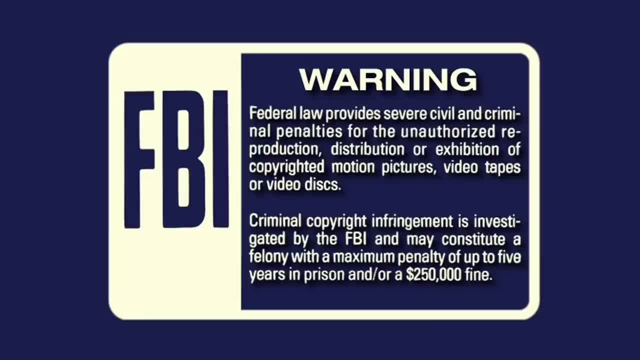 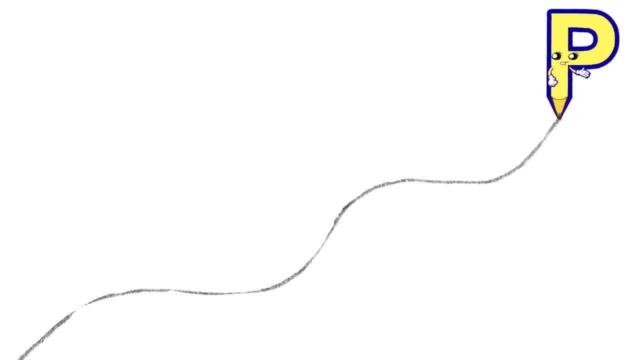 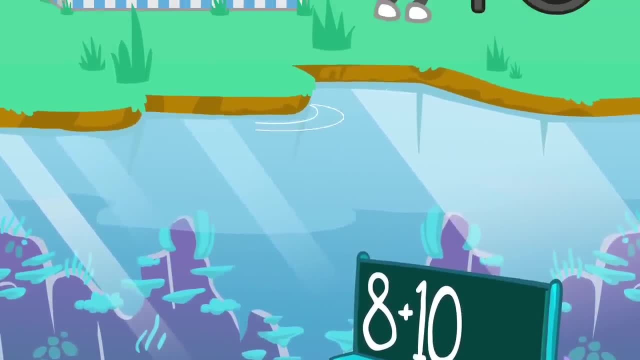 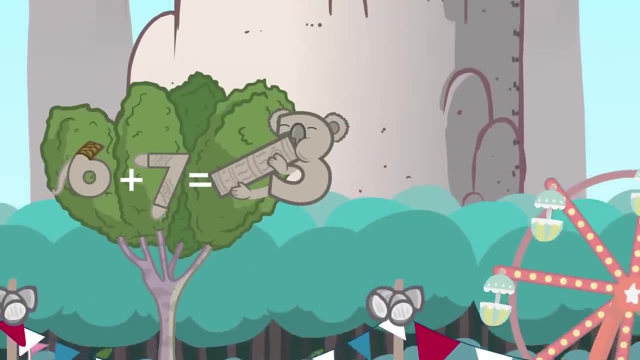 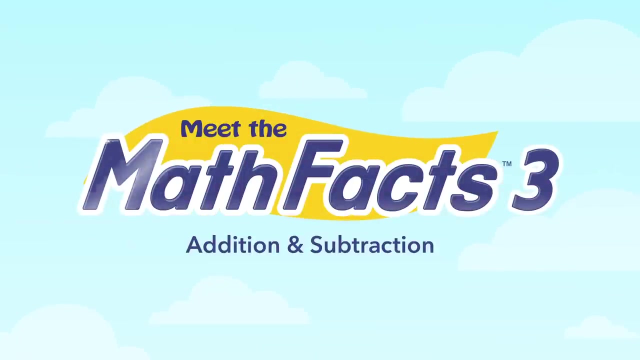 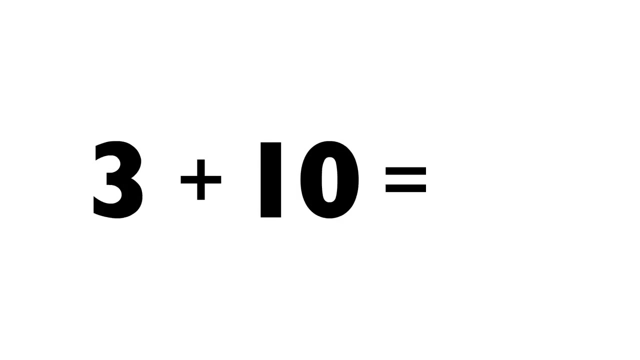 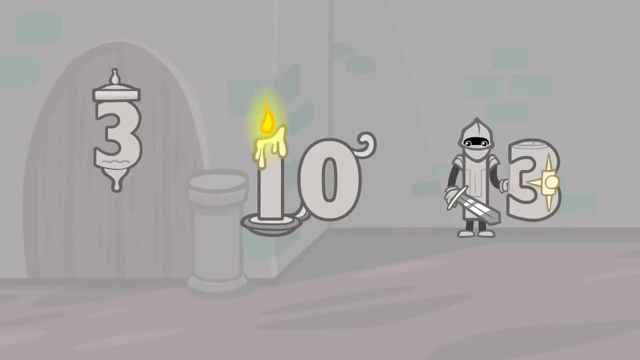 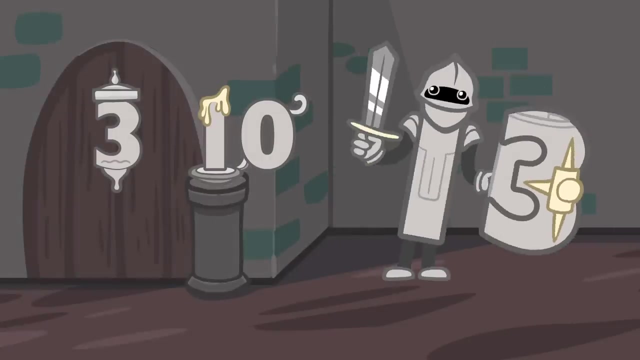 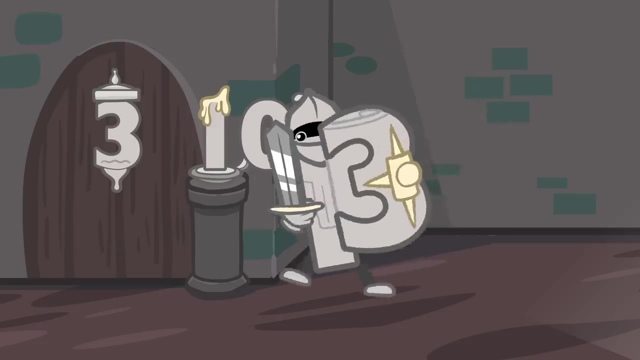 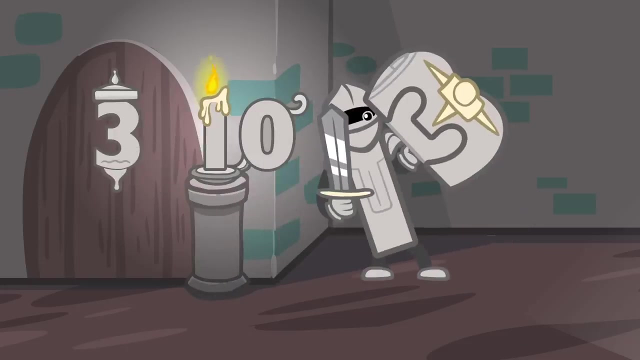 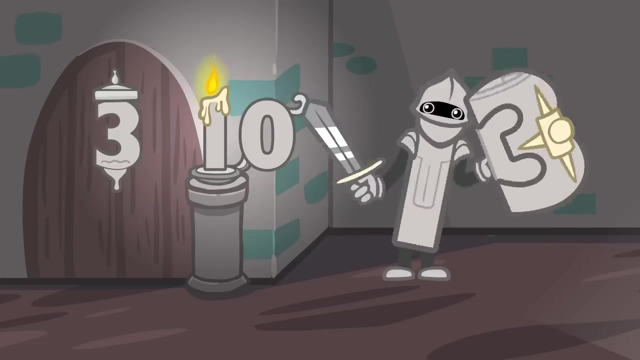 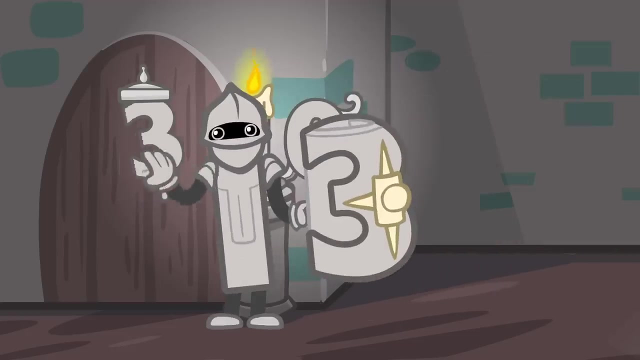 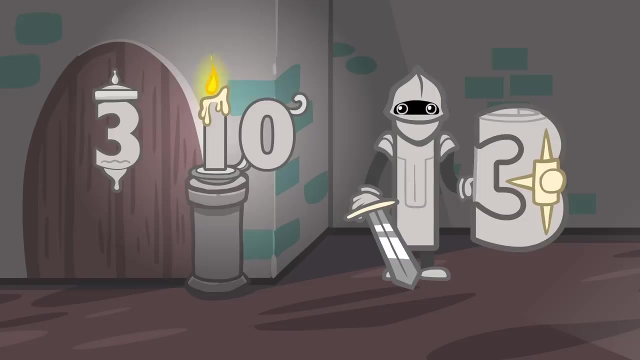 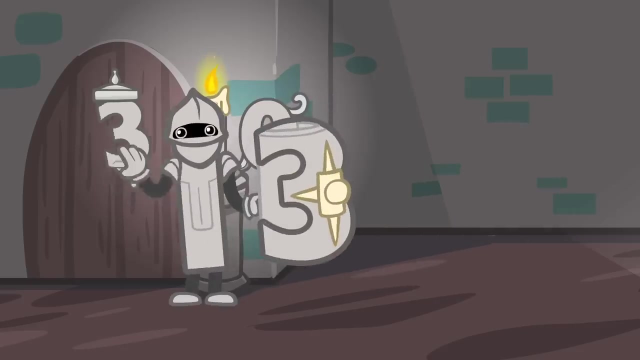 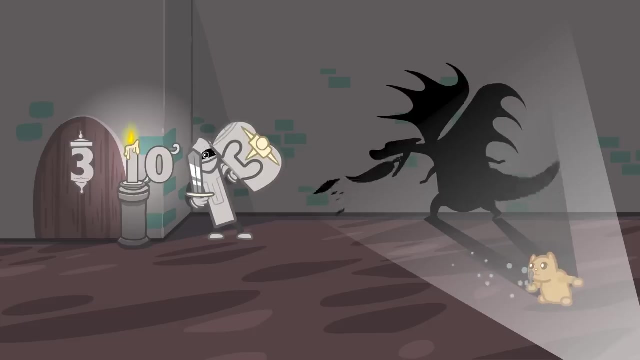 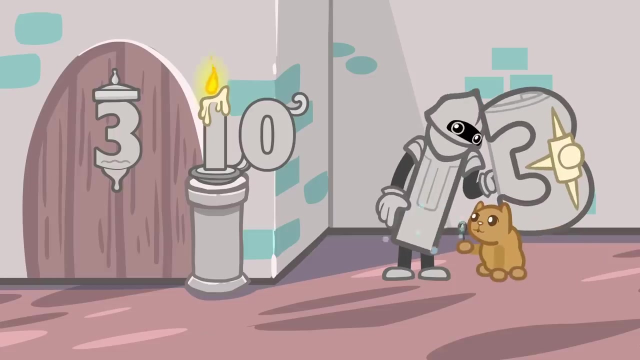 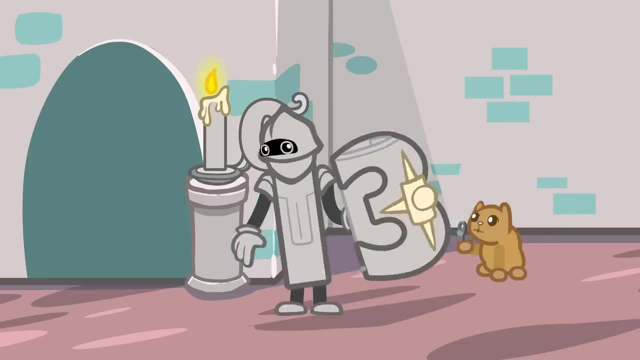 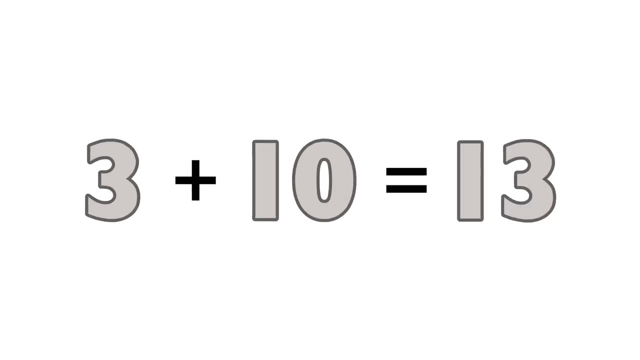 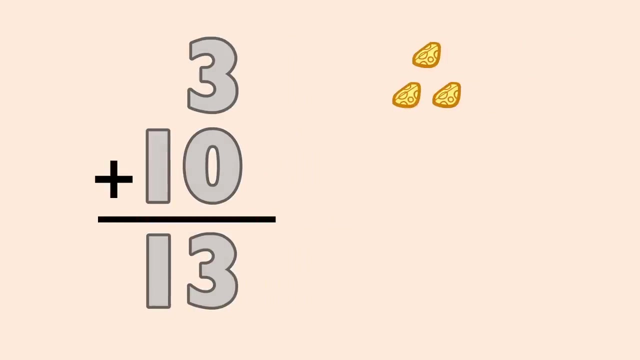 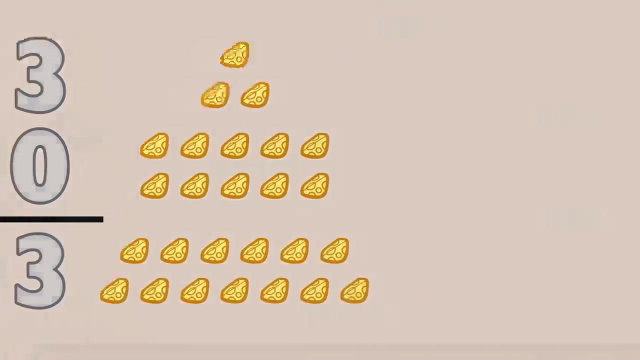 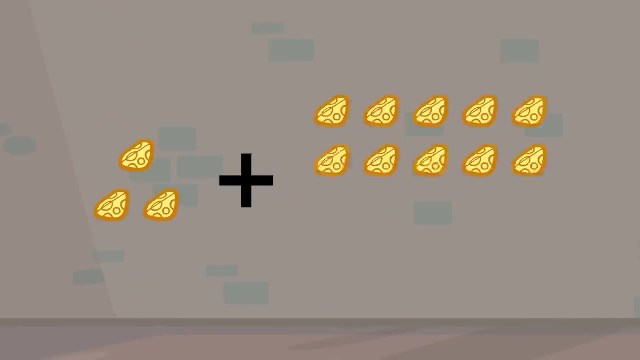 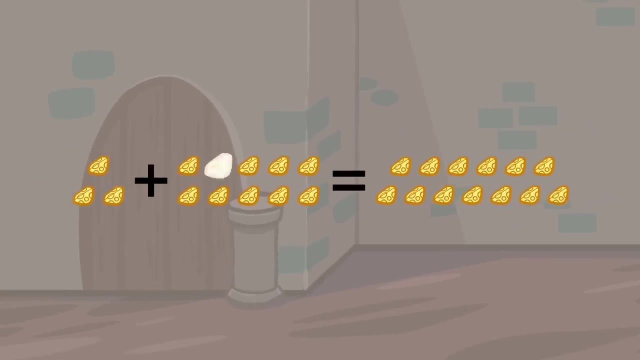 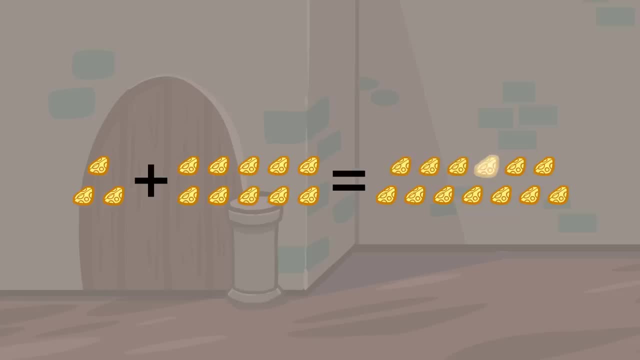 Equals: 1,, 2,, 3,, 4,, 5,, 6,, 7,, 8,, 9,, 10,, 11, 12, 13: 2,, 3,, 4,, 5,, 6,, 7,, 8,, 9,, 10,, 11,, 12, 13. 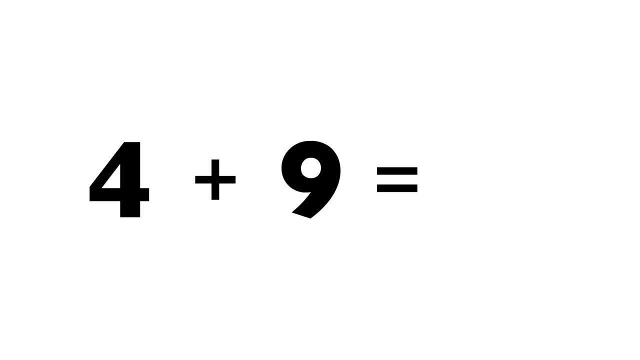 4 Plus 9 Equals. 4 Plus 9 Equals 14 1,, 2,, 3,, 5,, 6,, 7,, 8,, 9,, 10,, 11,, 12,, 13, 4 Plus 9 Equals. 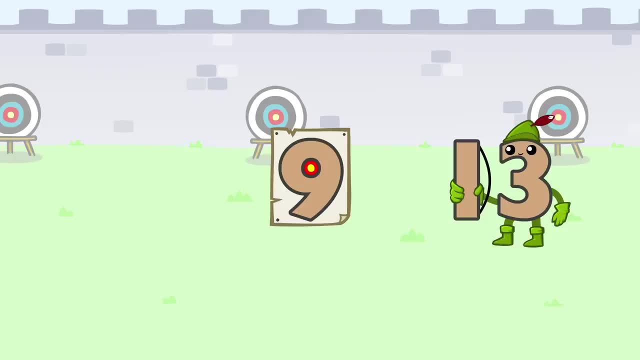 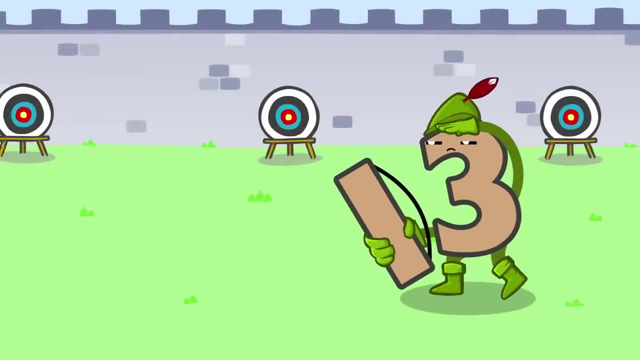 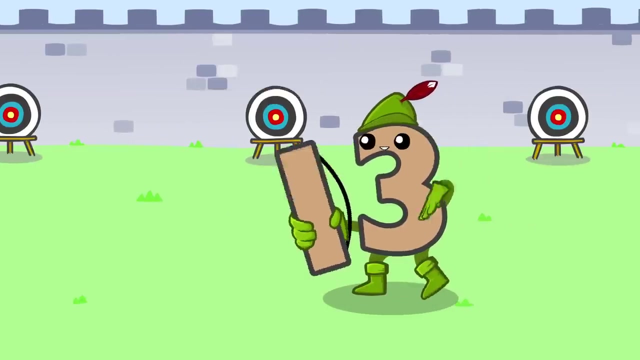 3 Plus 10 Equals 12: 13. 1,, 2,, 3,, 4,, 5,, 6,, 7,, 8,, 9,, 10,, 11,, 12,, 13. 4 plus 9 equals 13.. 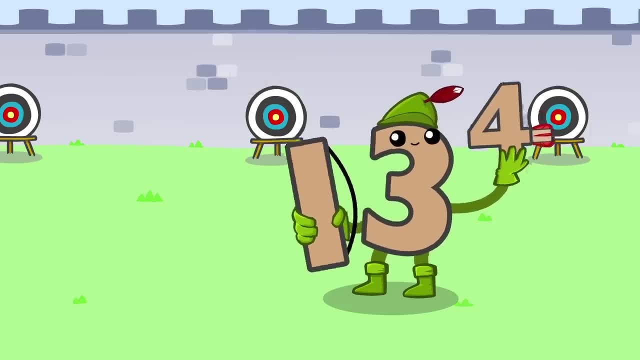 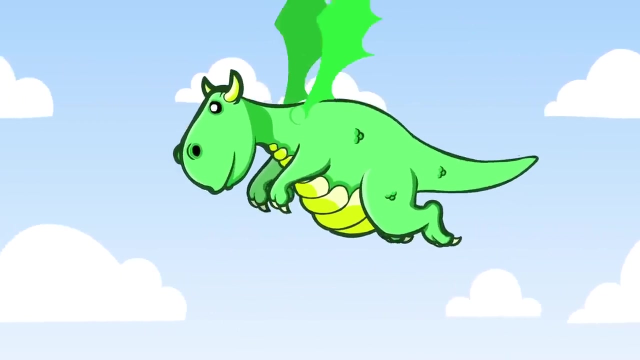 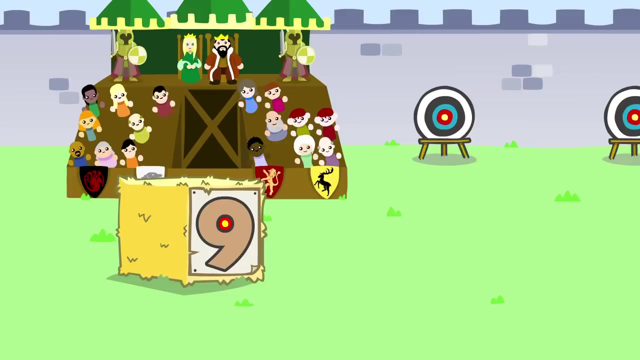 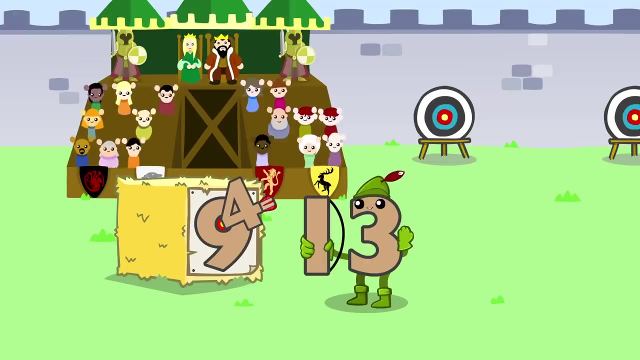 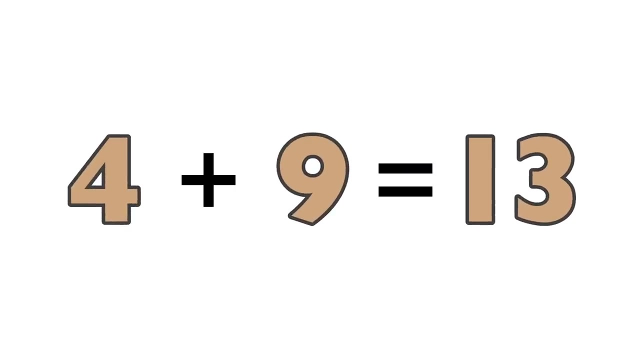 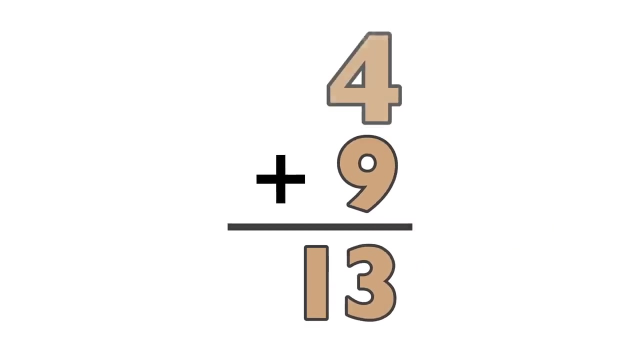 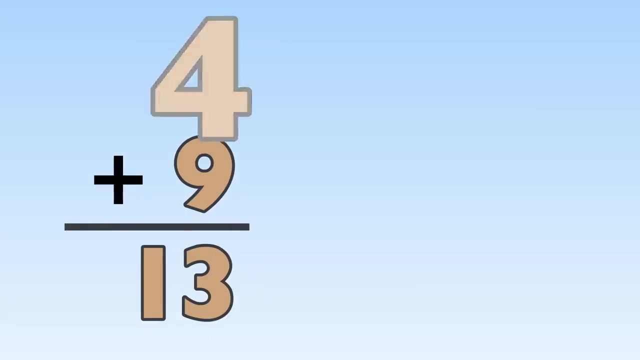 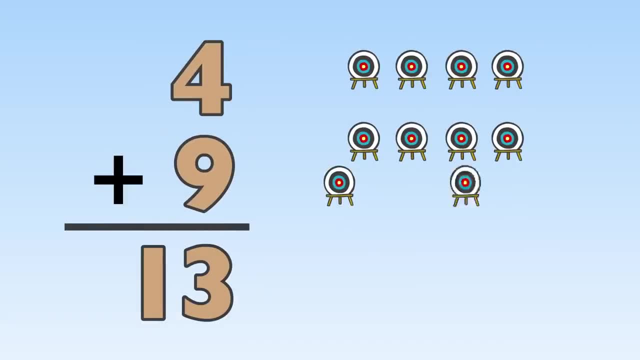 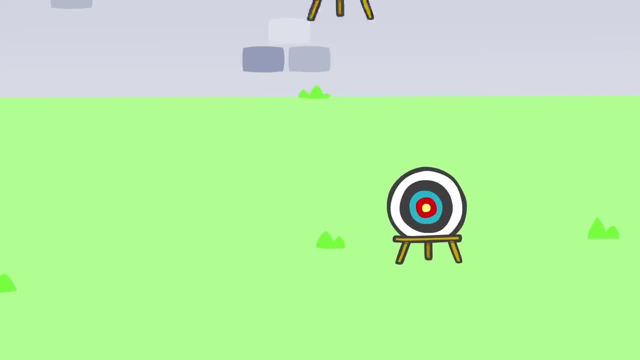 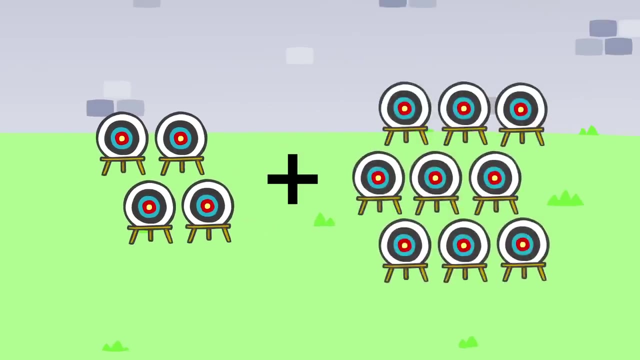 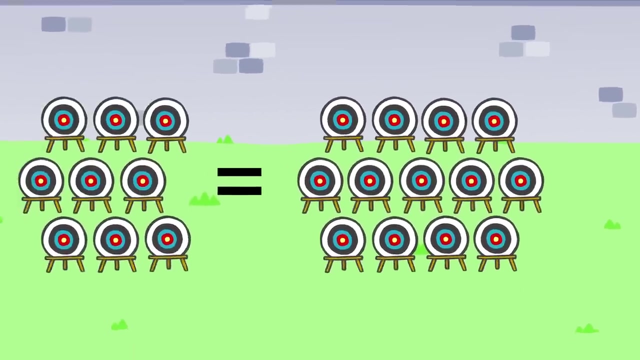 4 plus 9 equals 13.. 4 plus 9 equals 13.. 1,, 2,, 3,, 4,, 5,, 6,, 7,, 8,, 9,, 10,, 11,, 12, 13.. 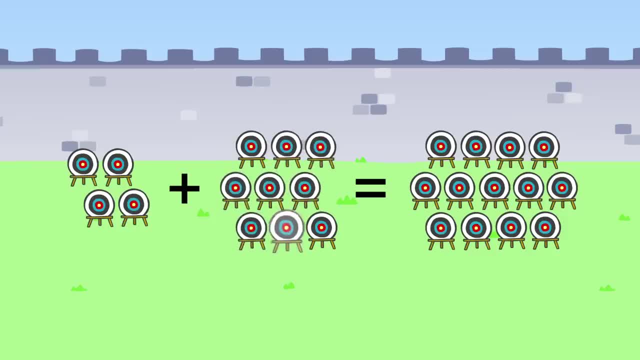 1,, 2,, 3,, 4,, 5,, 6,, 7,, 8,, 9,, 10,, 11,, 12, 13.. Equals: 1,, 2,, 3,, 4,, 5,, 6,, 7,, 8,, 9,, 10,, 11,, 12,, 13.. 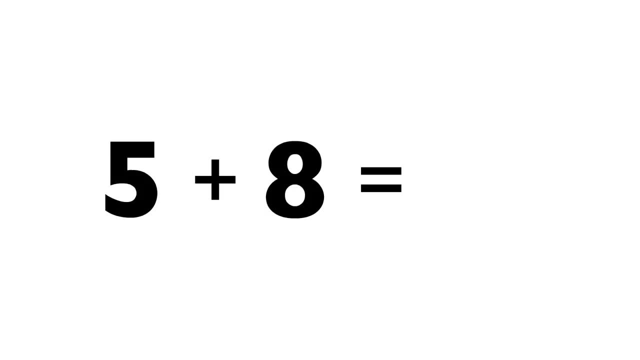 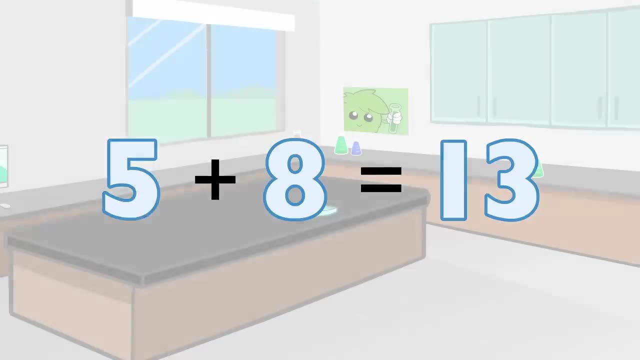 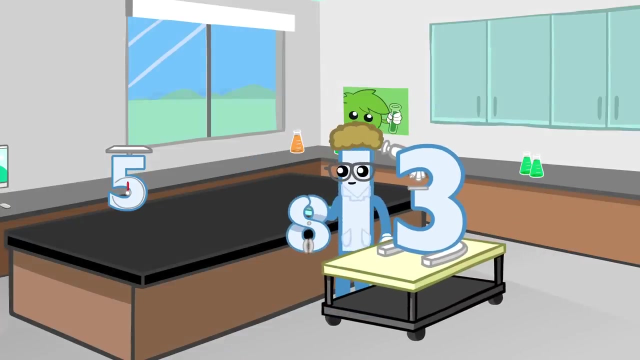 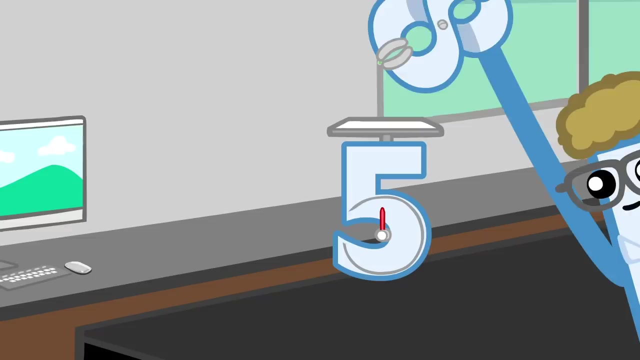 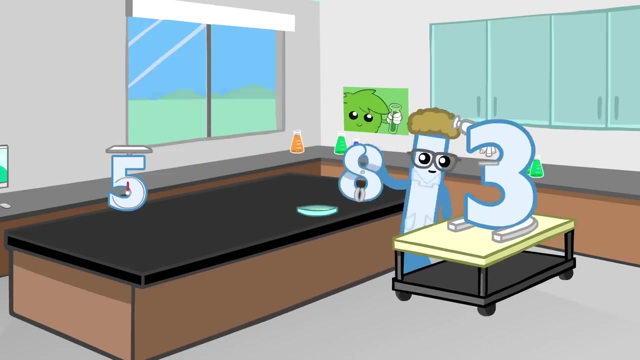 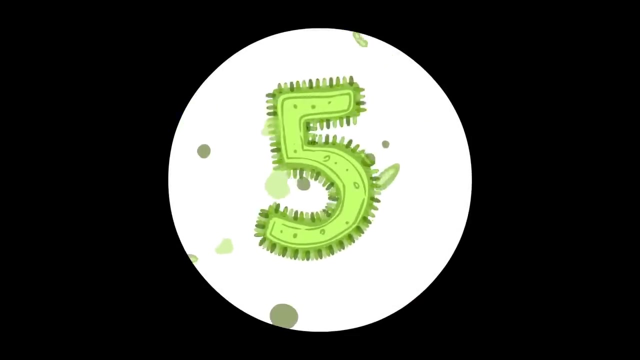 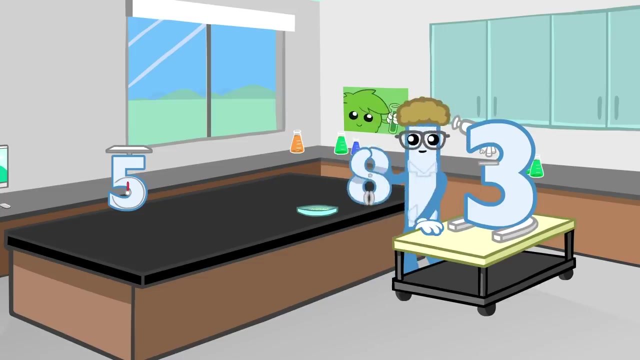 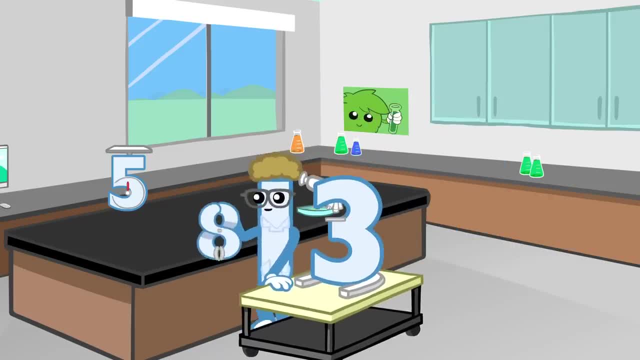 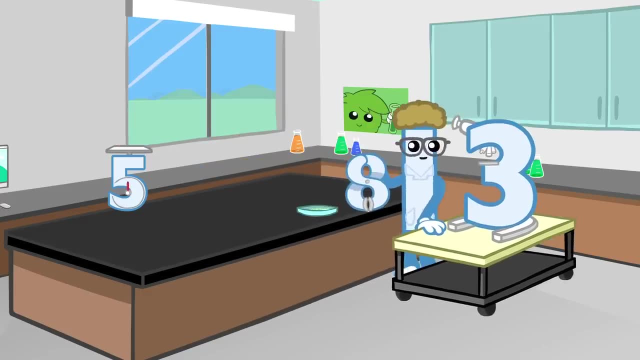 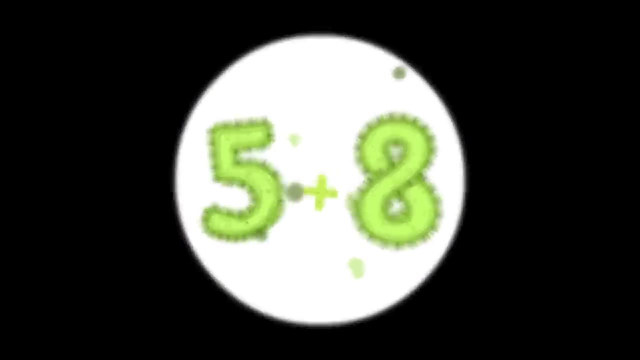 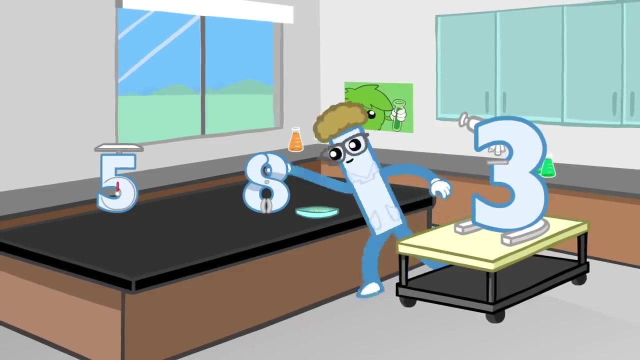 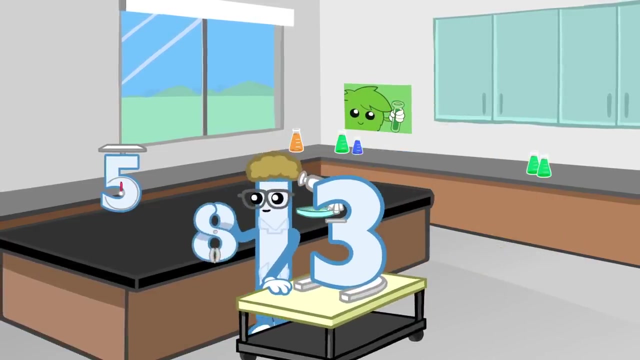 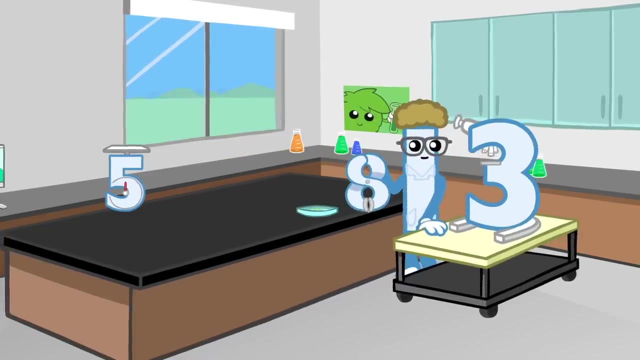 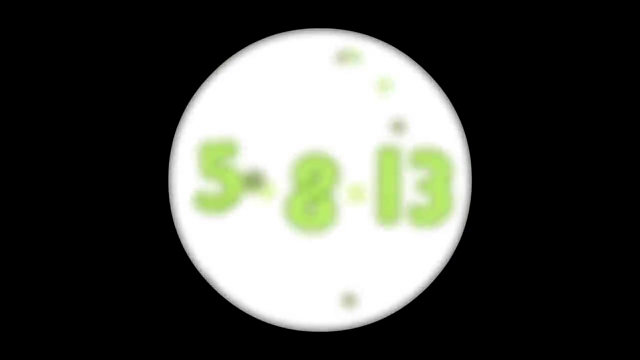 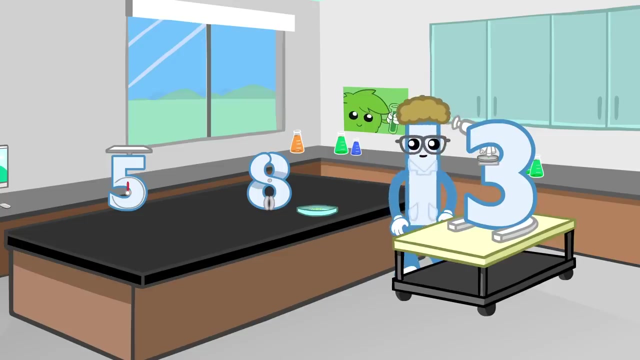 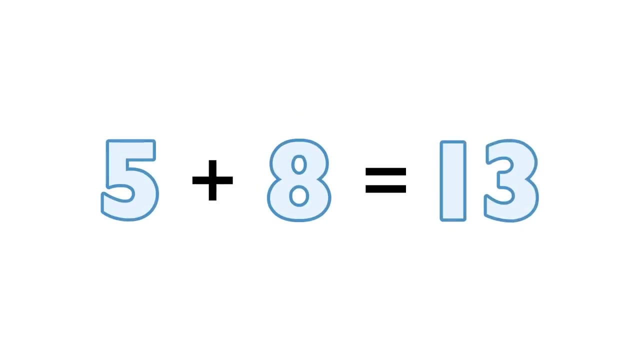 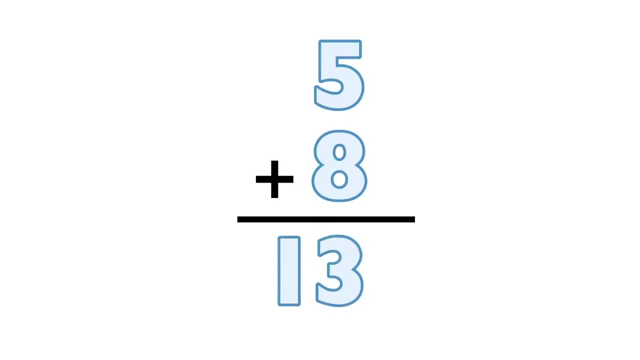 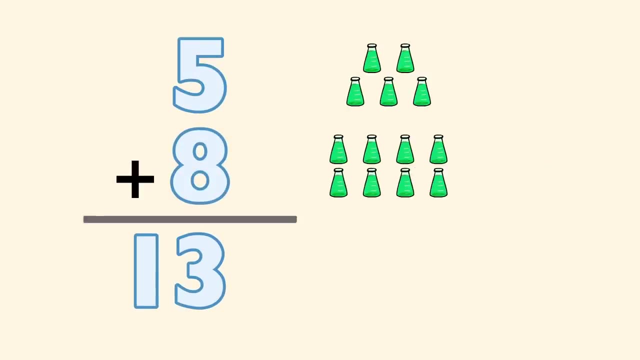 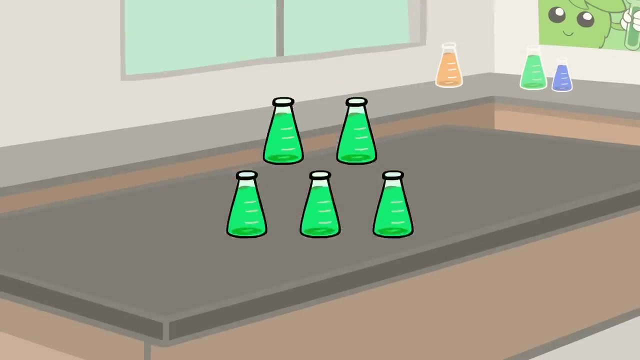 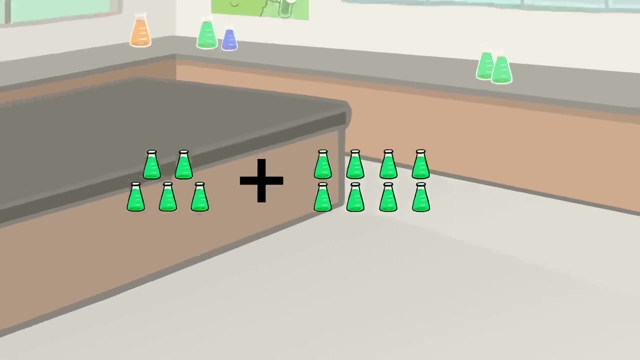 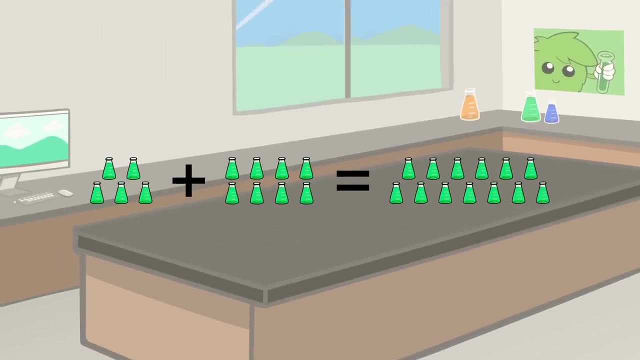 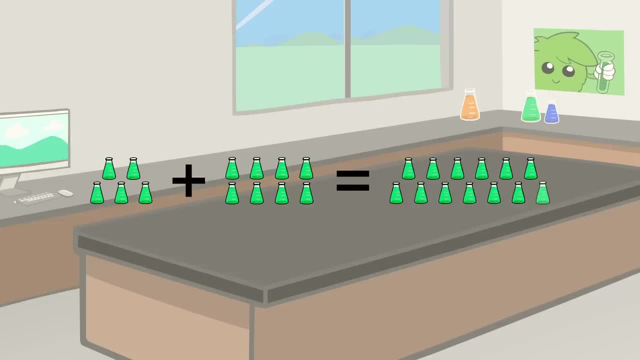 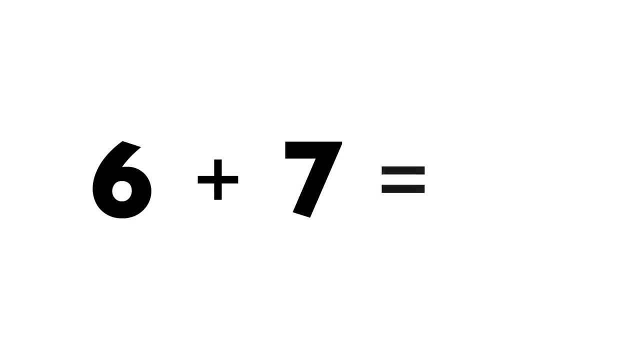 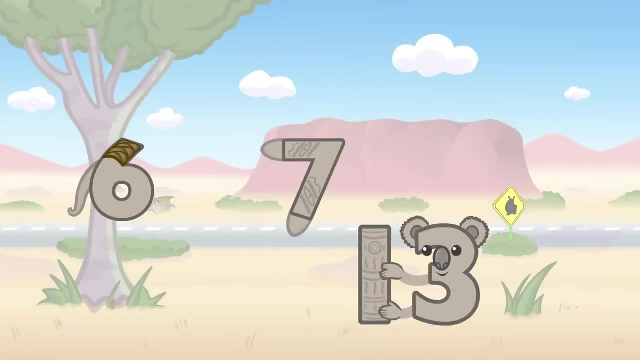 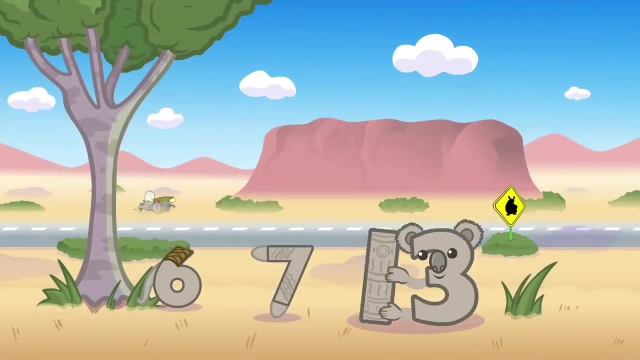 single one: two, three, four, five, six, seven, eight, nine, ten, eleven, twelve. thirteen equals Six plus seven equals Six plus seven equals Thirteen. Six plus seven equals Thirteen. 6 plus 7 equals 13.. 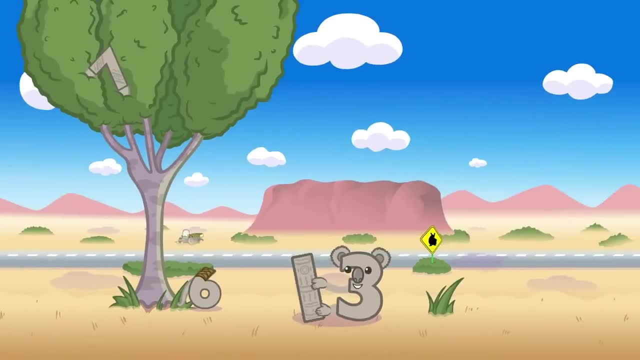 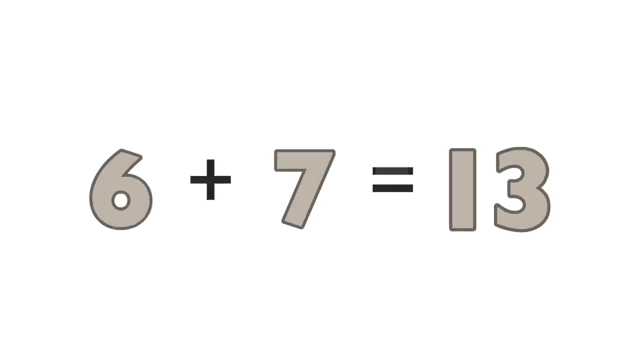 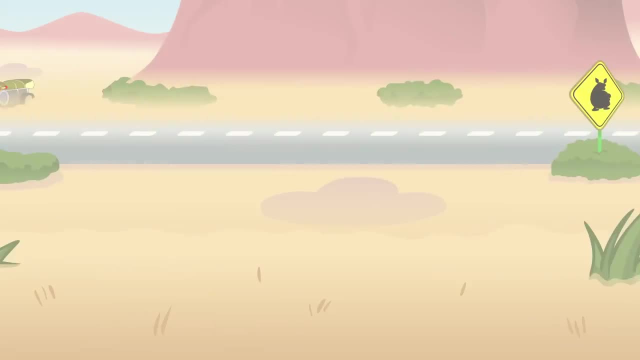 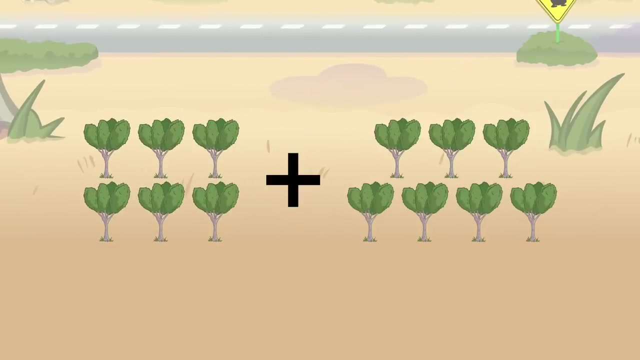 5, 4, 5, 6 plus 7 equals 13.. 1, 10, 10, 2, 3, 3, 6, 2, 3, 1, 2,. 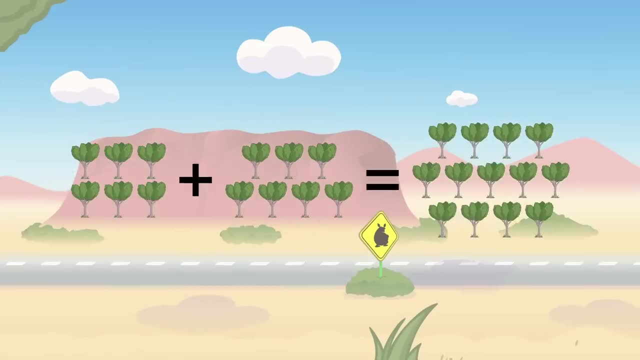 3,, 4,, 4, 3, 4,, 1,, 7,, 1,, 2,, 3,, 4,, 5,, 6,, 7,, 8,, 9,, 10,, 11,, 12, 13 equals 1,, 2,, 3,, 4,, 5,, 6,, 7,, 8,, 9,, 10,, 11,, 12, 13.. 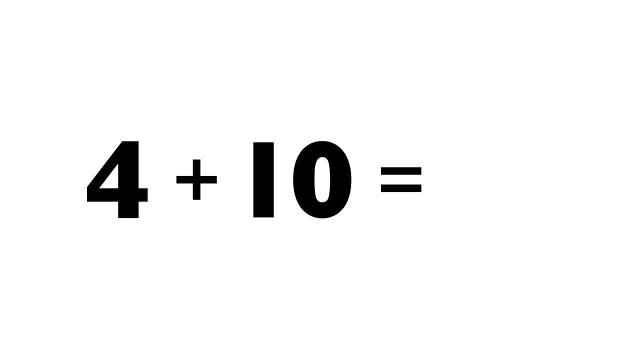 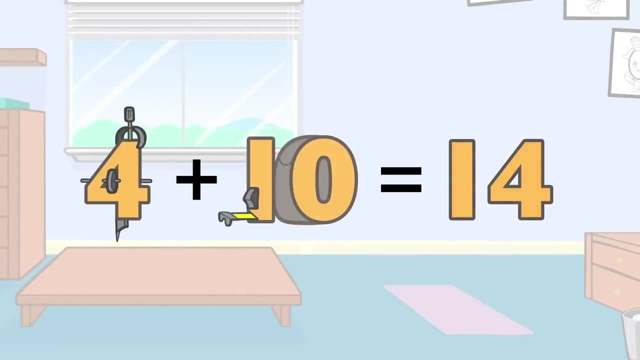 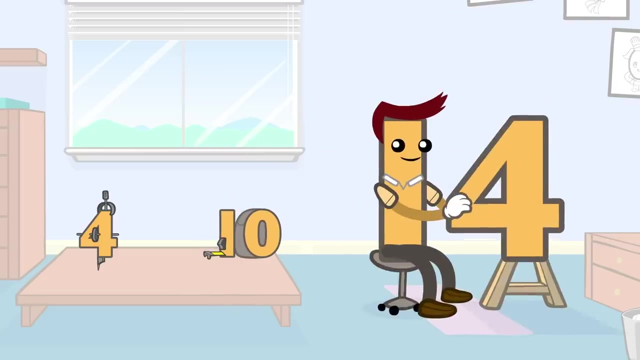 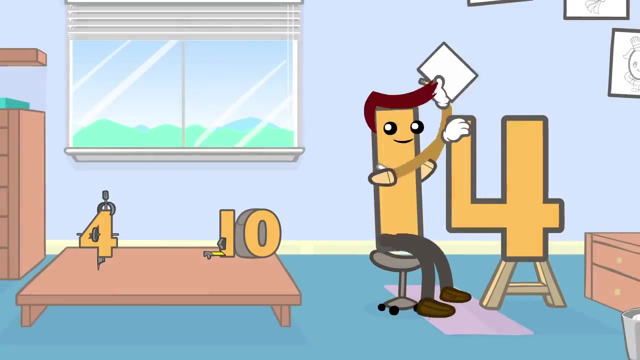 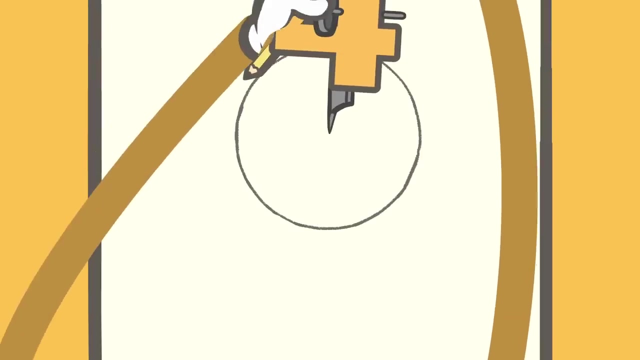 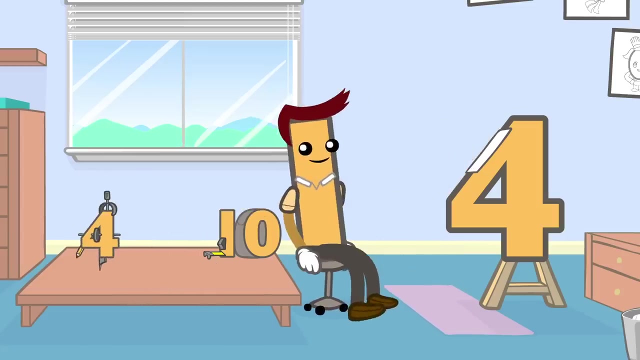 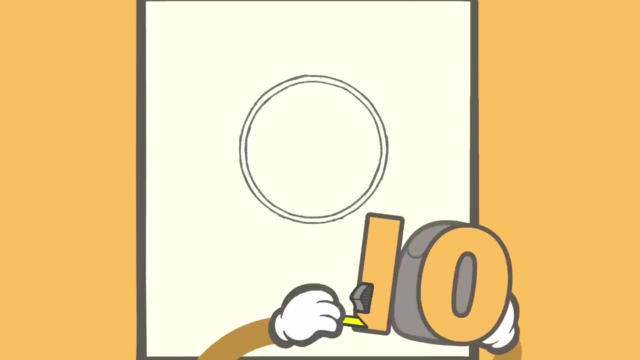 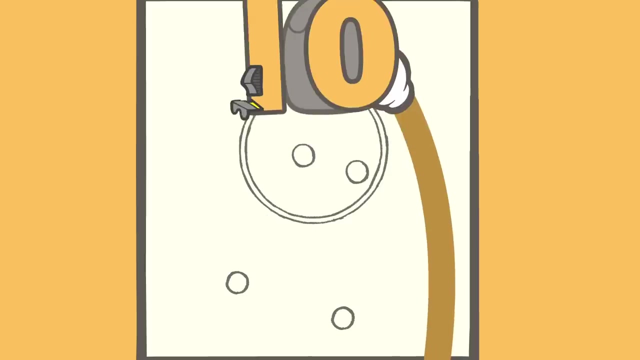 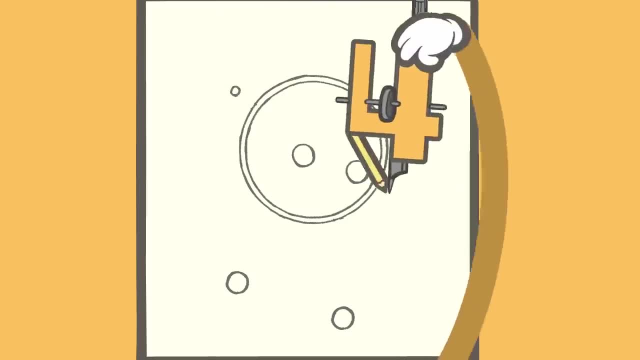 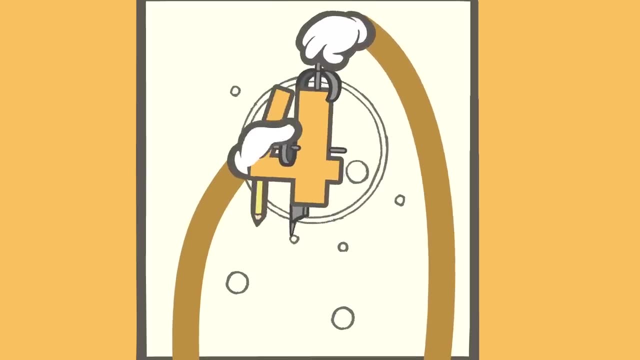 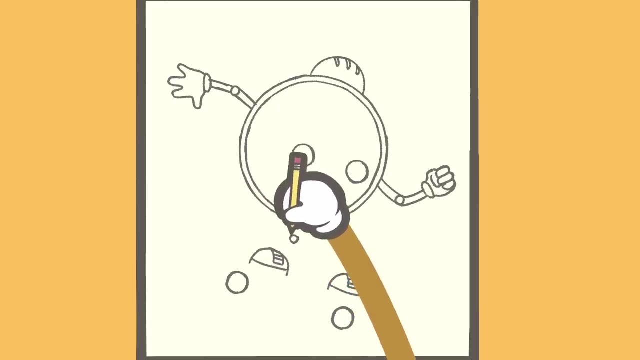 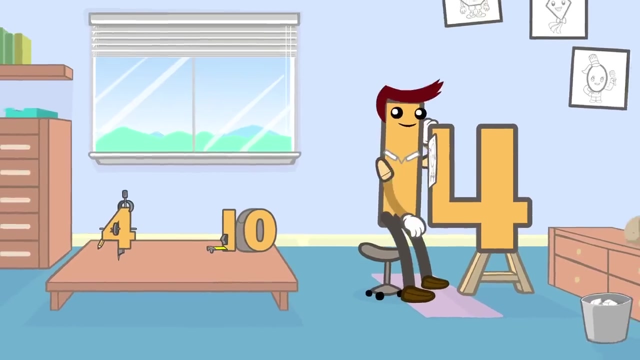 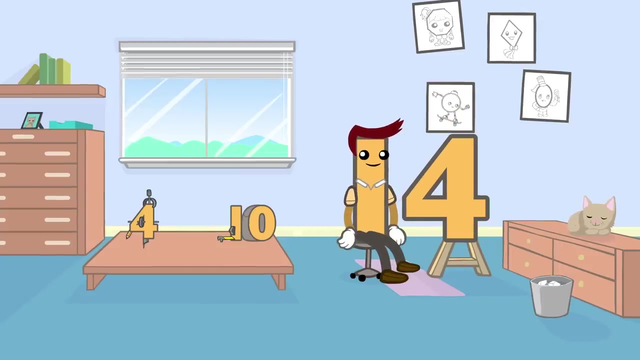 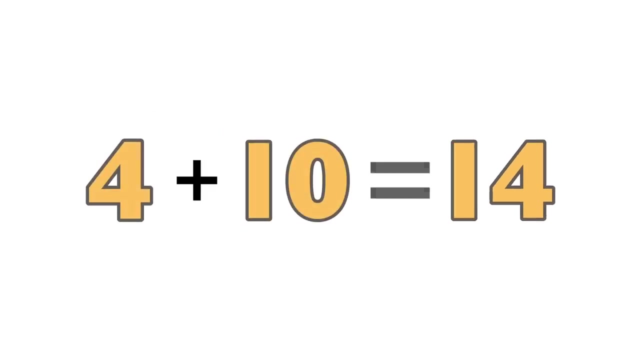 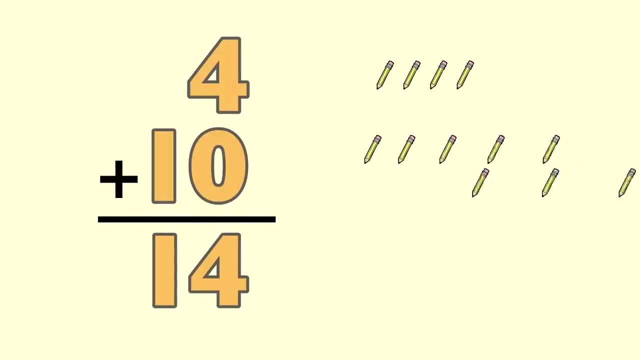 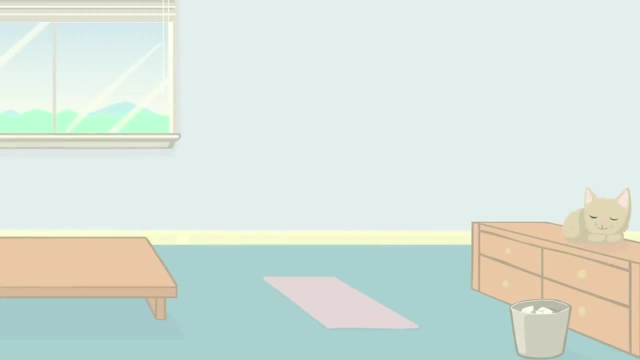 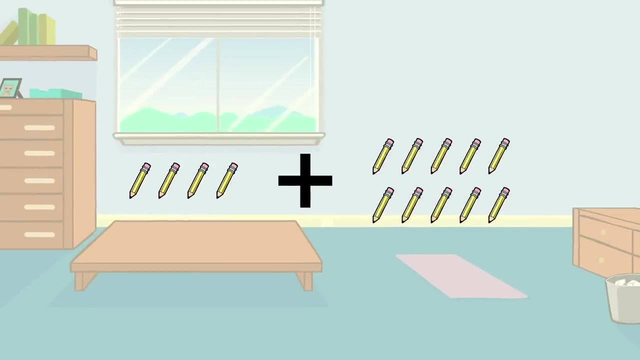 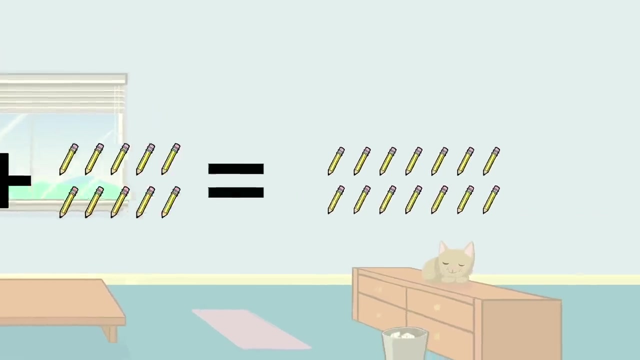 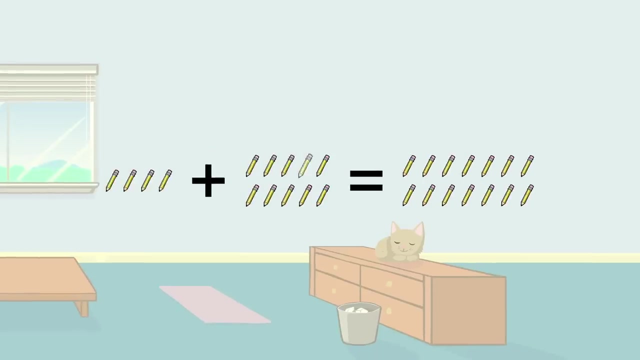 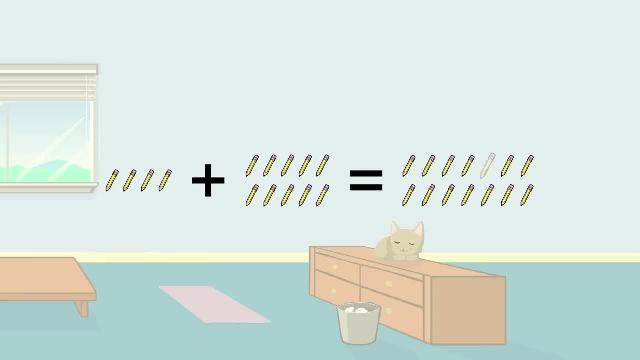 1,, 2,, 3,, 4,, 5,, 6,, 7,, 8,, 9,, 10,, 11,, 12,, 13,, 14.. 1,, 2,, 3,, 4,, 5,, 6,, 7,, 8,, 9,, 10,, 11,, 12,, 13,, 14.. 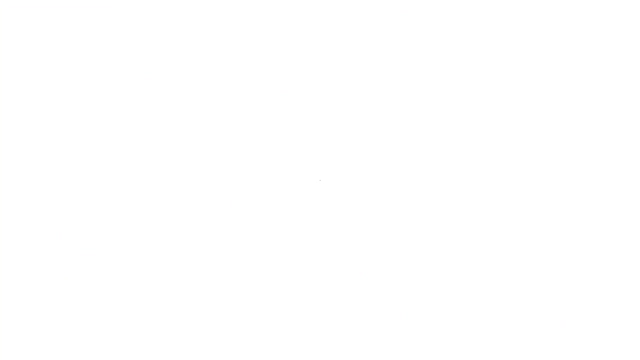 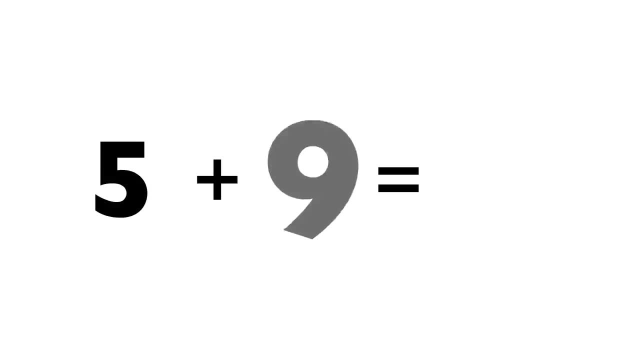 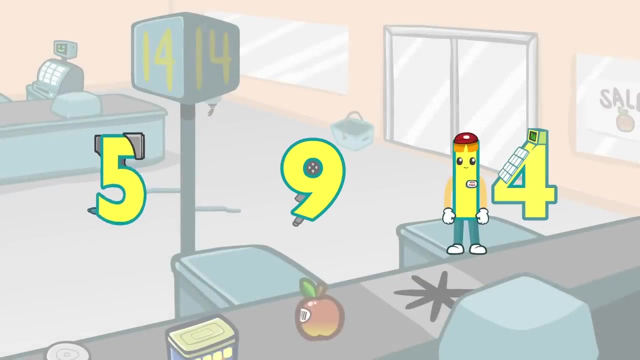 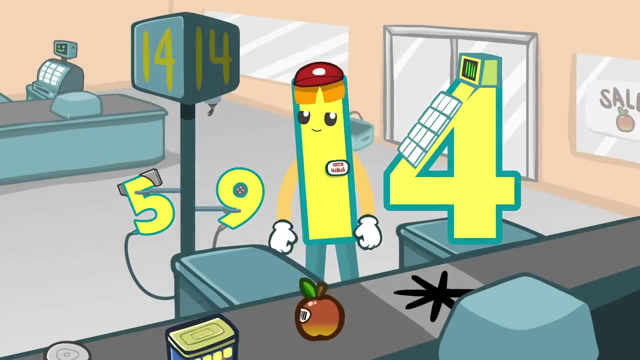 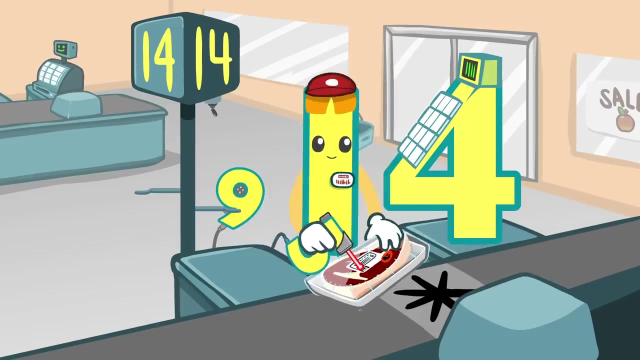 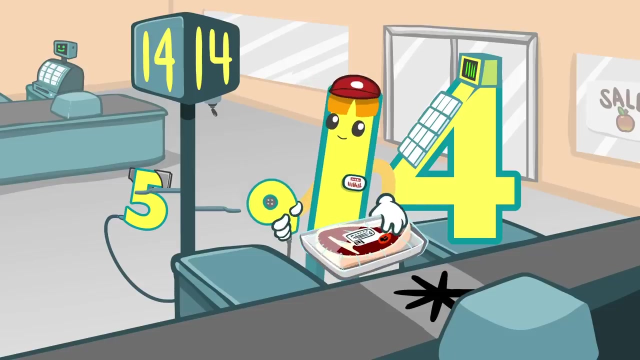 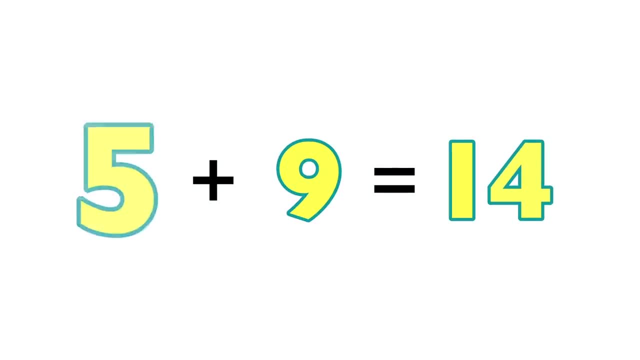 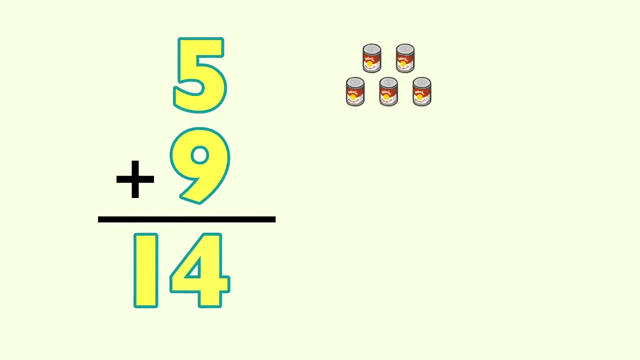 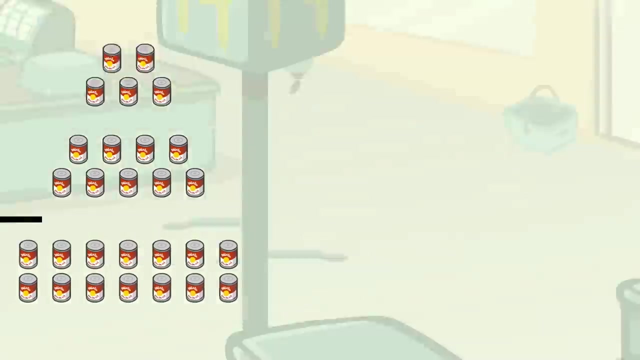 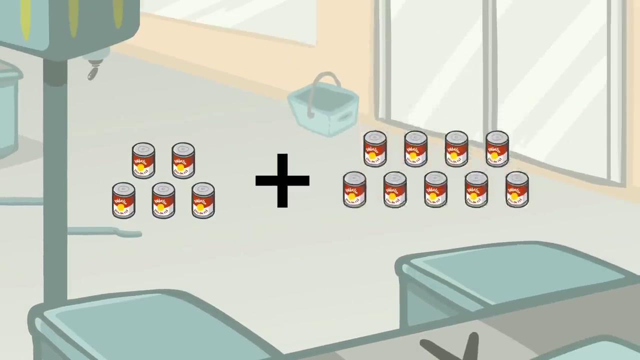 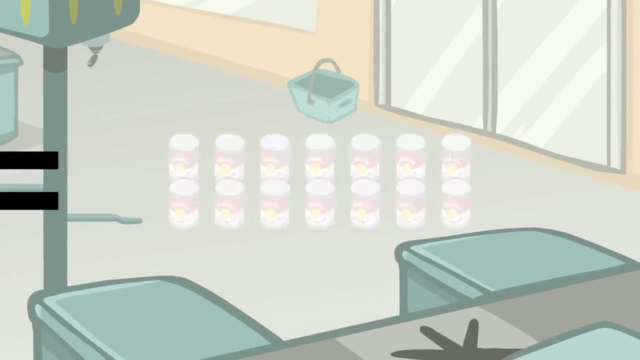 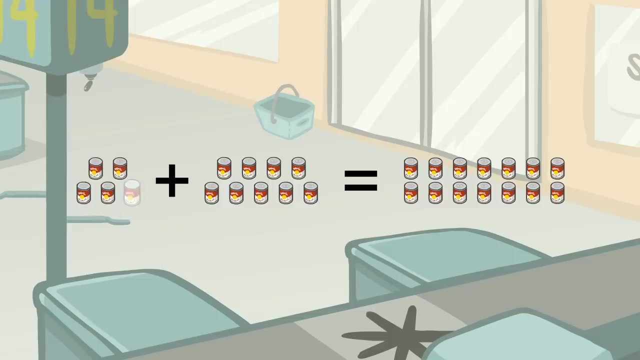 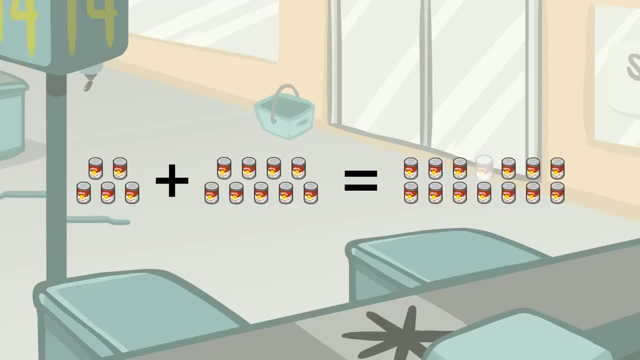 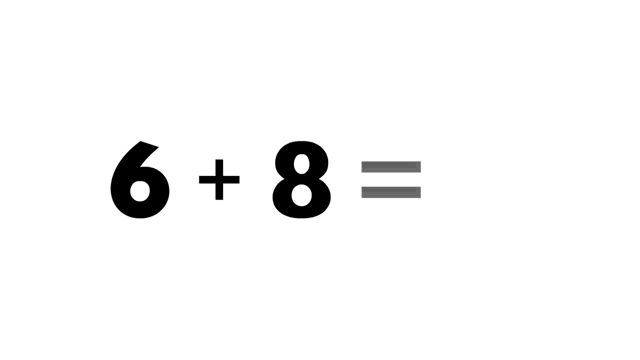 Equals: 1,, 2,, 3,, 4,, 5,, 6,, 7,, 8,, 9,, 10,, 11,, 12,, 13, 14.. 6 plus 8 equals. 6 plus 8 equals. 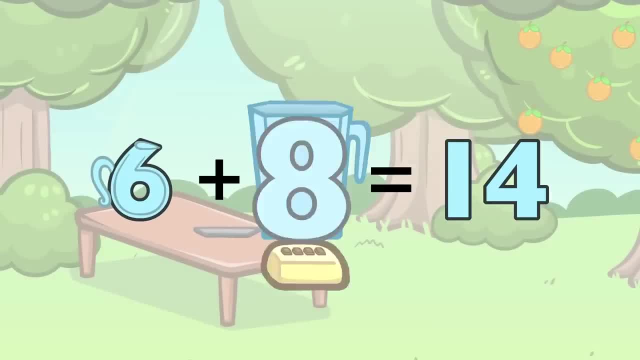 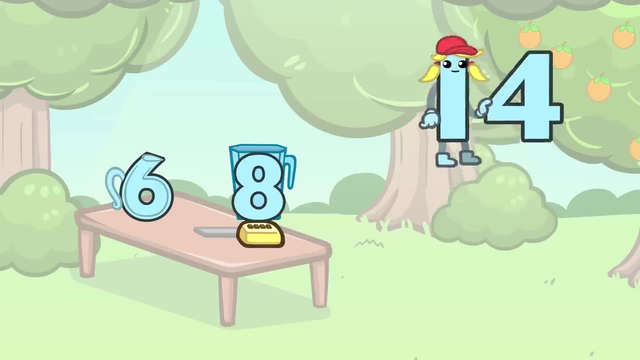 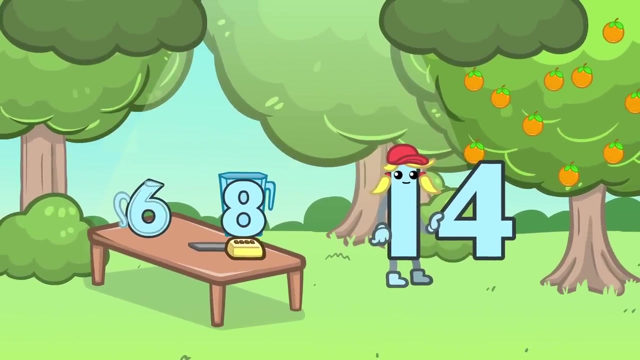 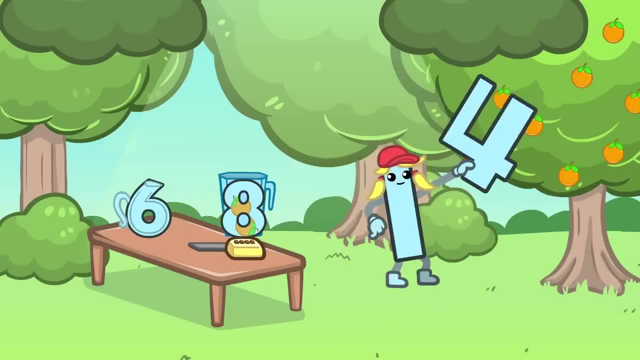 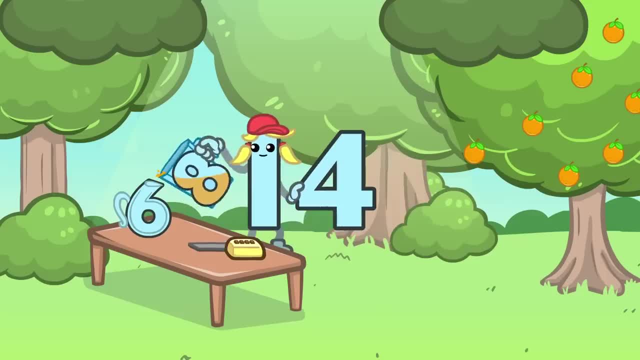 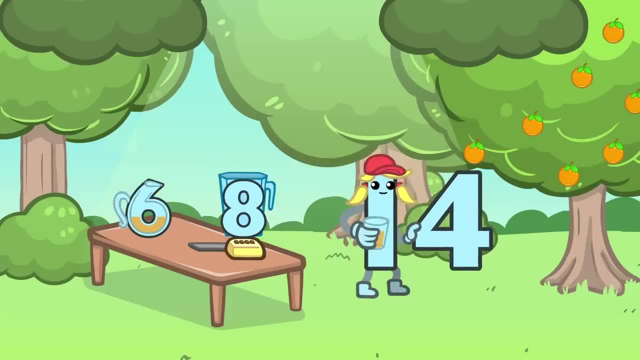 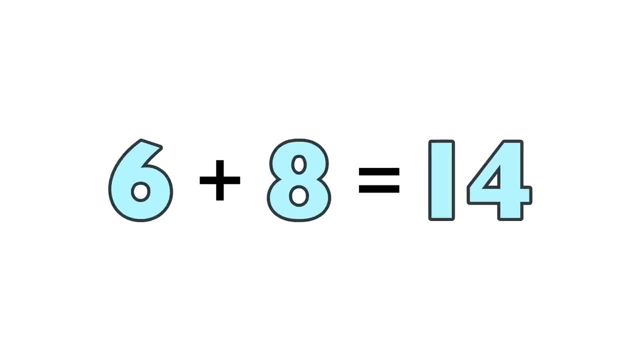 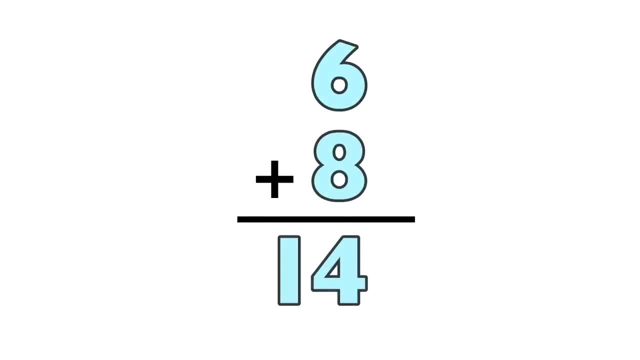 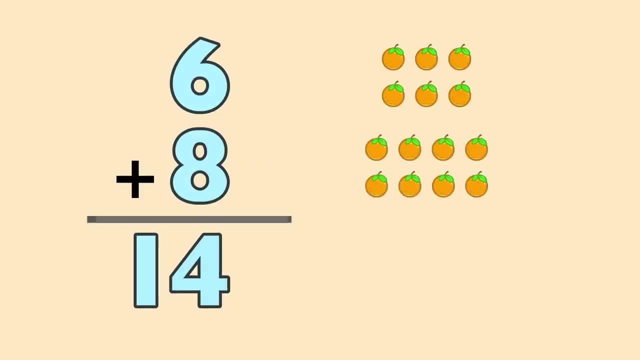 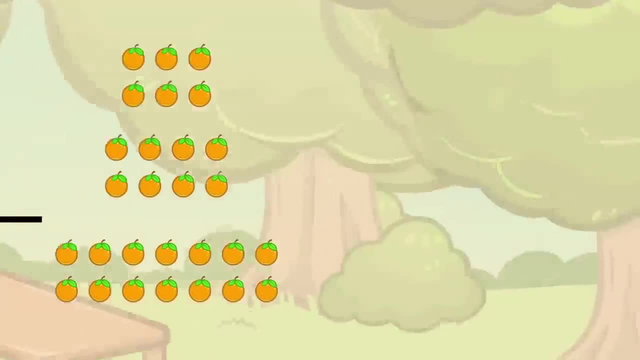 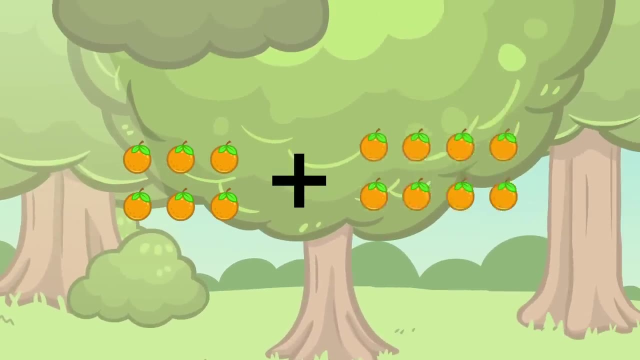 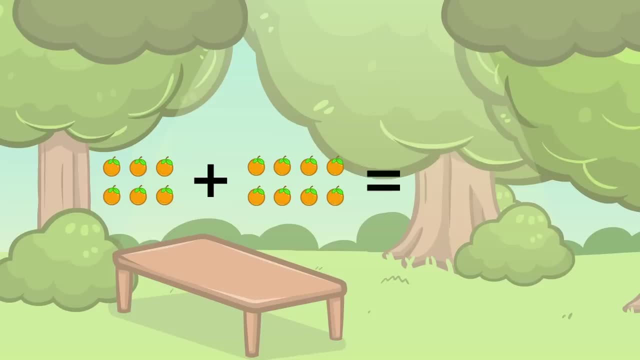 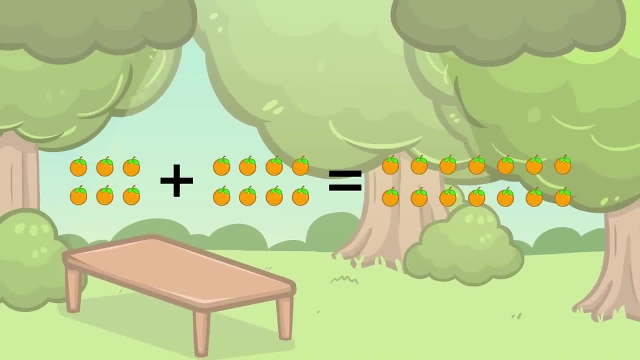 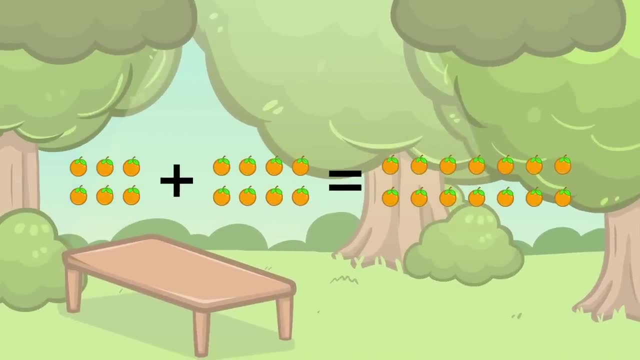 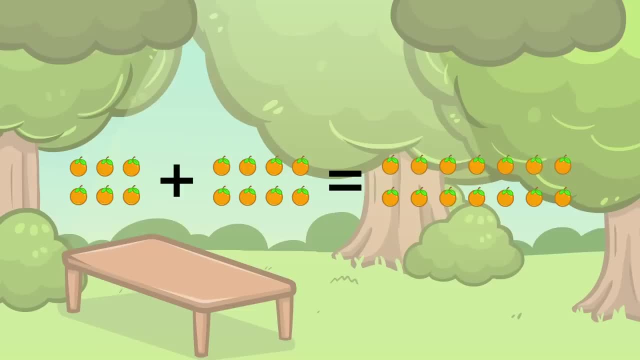 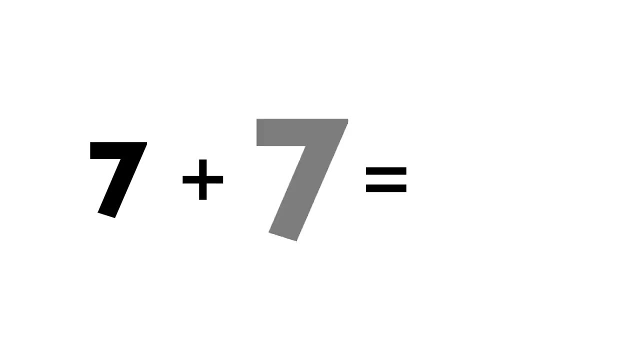 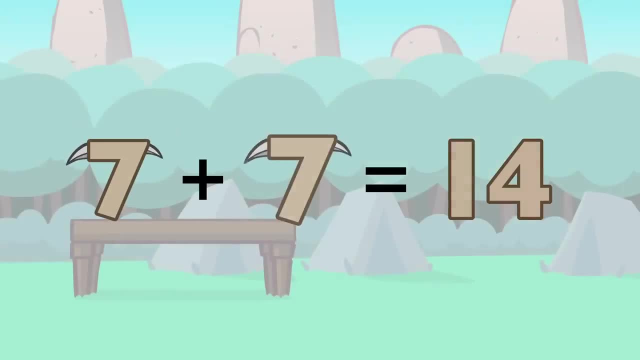 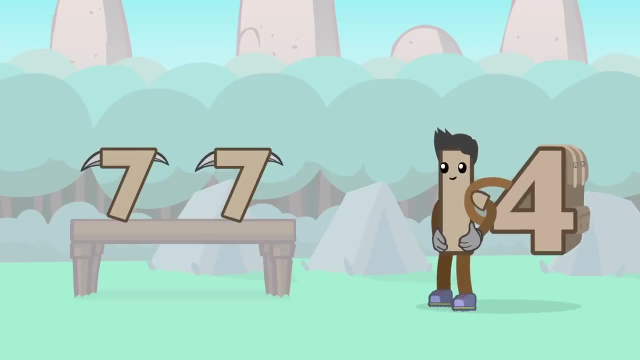 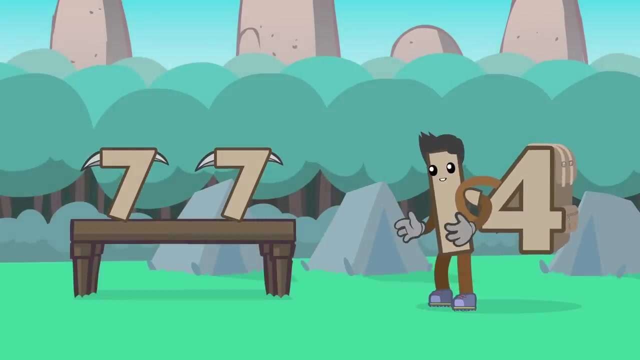 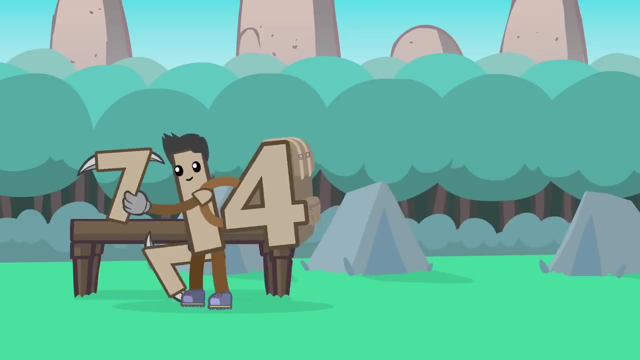 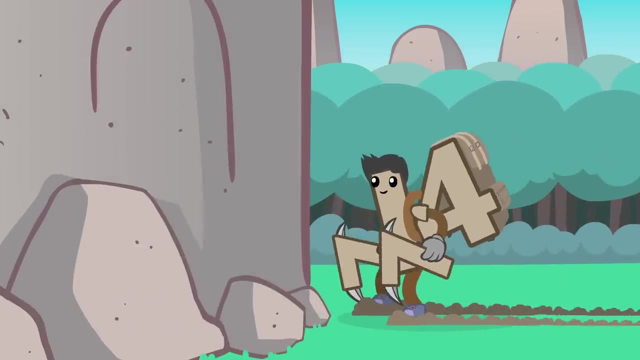 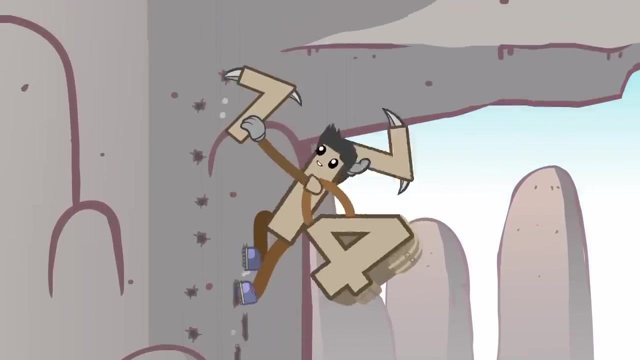 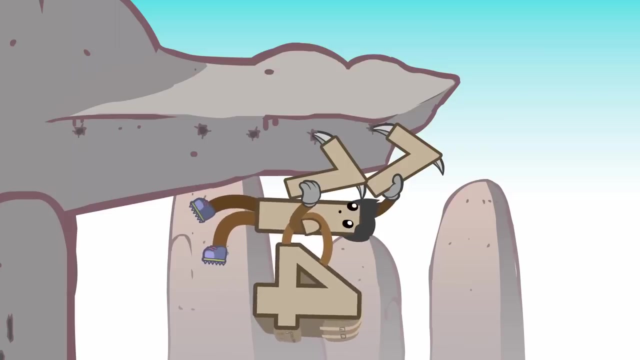 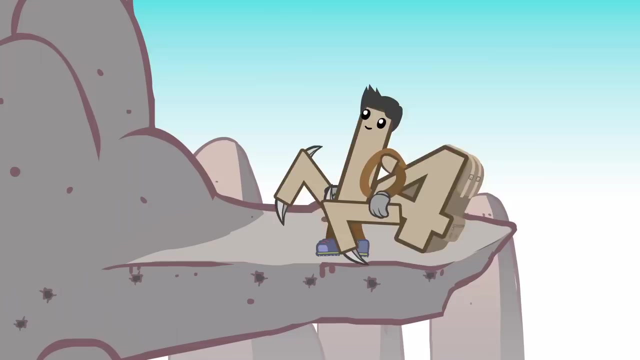 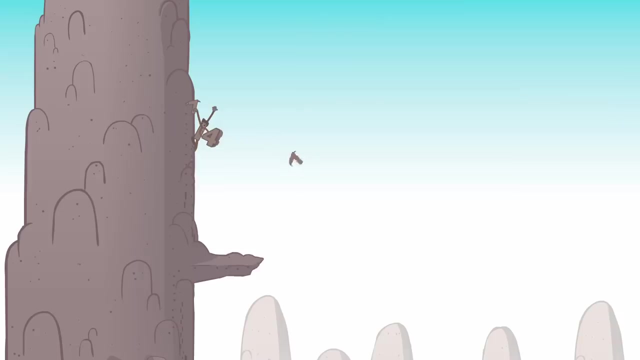 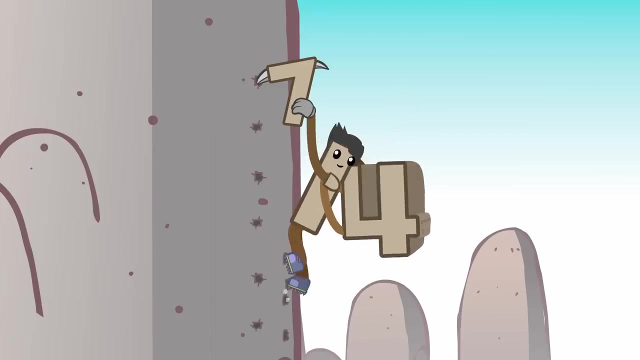 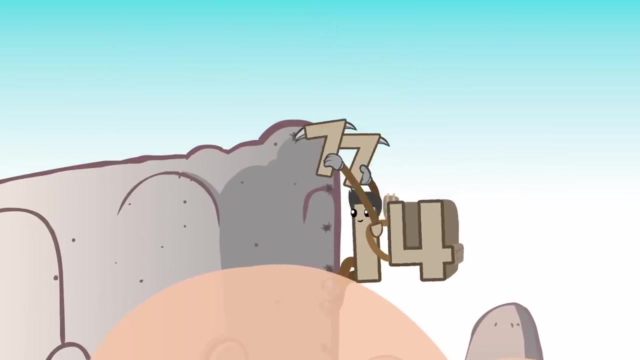 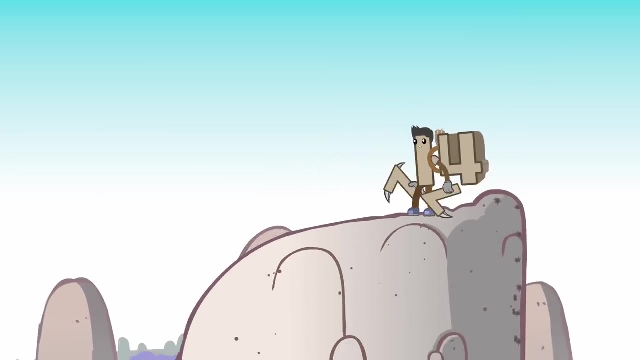 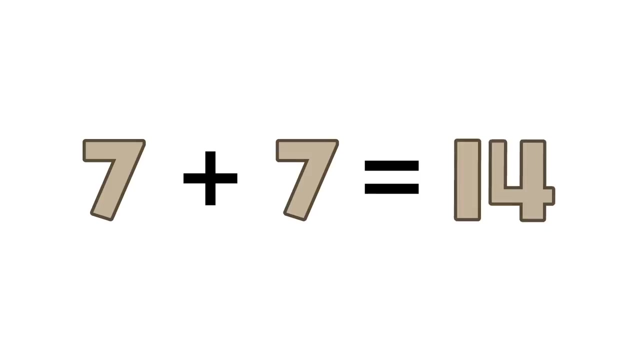 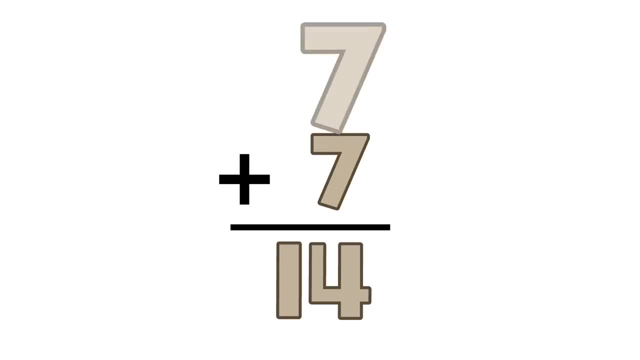 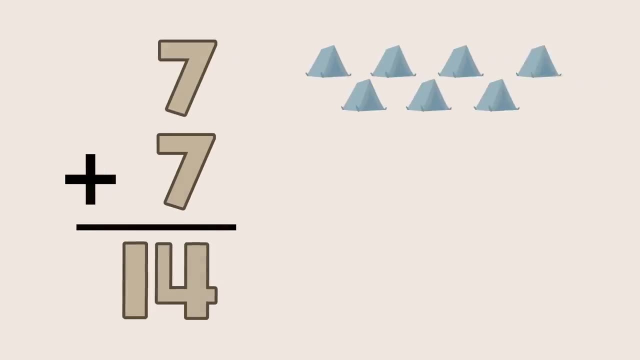 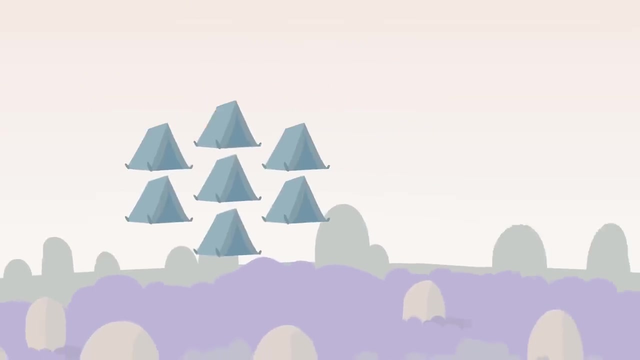 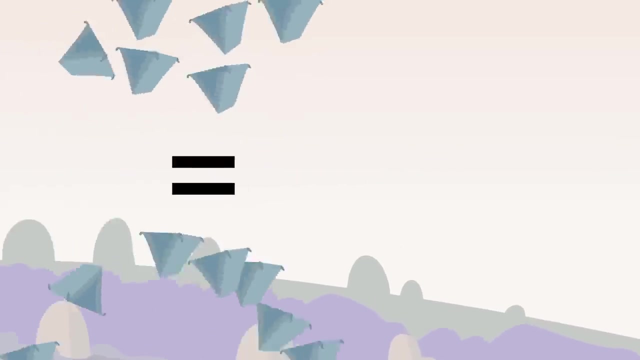 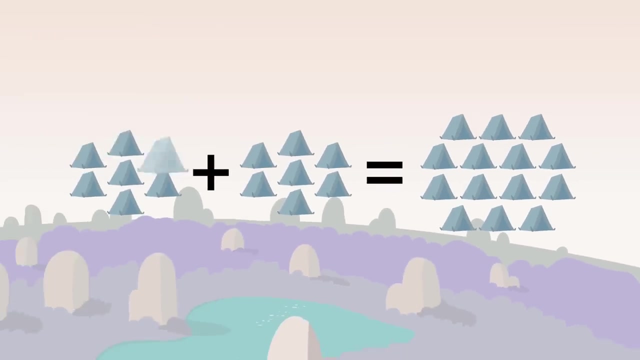 7 plus 7 equals 14.. 7 plus 7 equals 14.. 7 plus 7 equals 14.. 1,, 2,, 3,, 4,, 5,, 6,, 7,, 8,, 9,, 10,, 11,, 12,, 13,, 14 equals. 1,, 2,, 3,, 4,, 5,, 6,, 7,, 8,, 9,, 10,, 11,, 12,, 13, 14 equals. 1,, 2,, 3,, 4,, 5,, 6,, 7,, 8,, 9,, 10,, 11,, 12,, 13,, 14 equals. 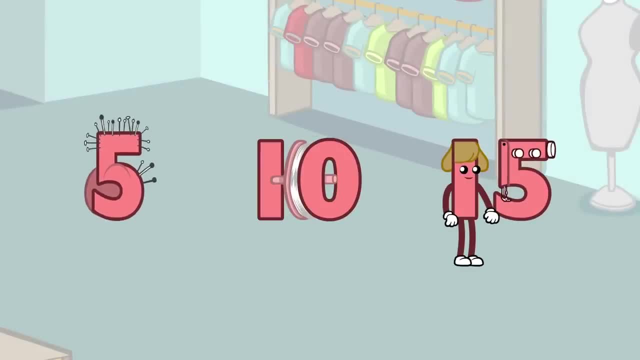 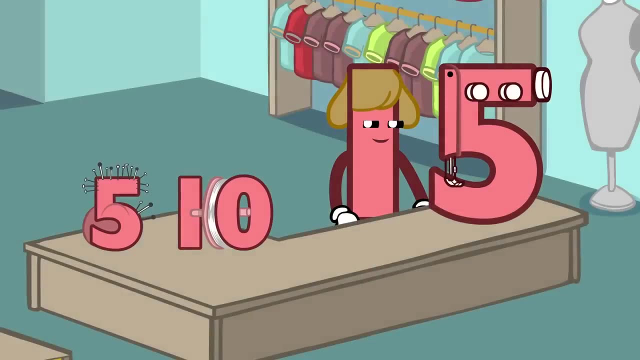 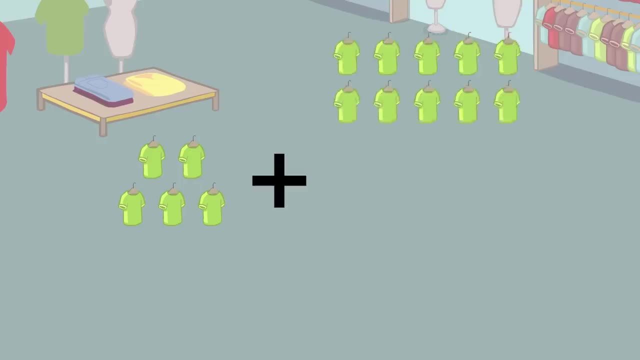 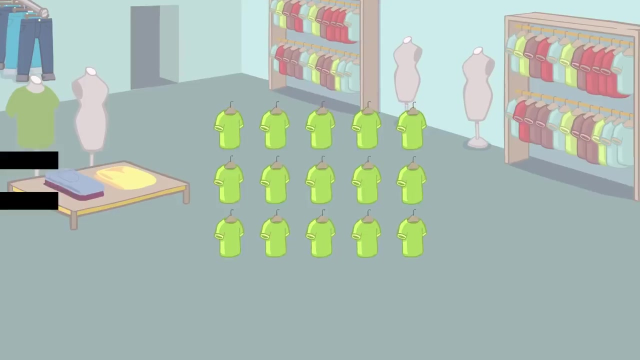 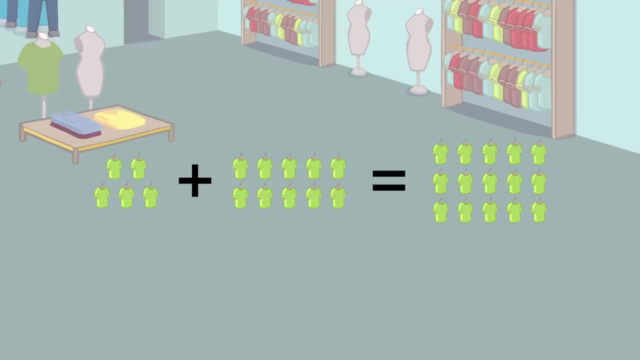 5 plus 10 equals 15.. 1,, 2,, 3,, 4,, 5,, 6,, 7,, 8,, 9,, 10,, 11,, 12,, 13,, 14, 15. 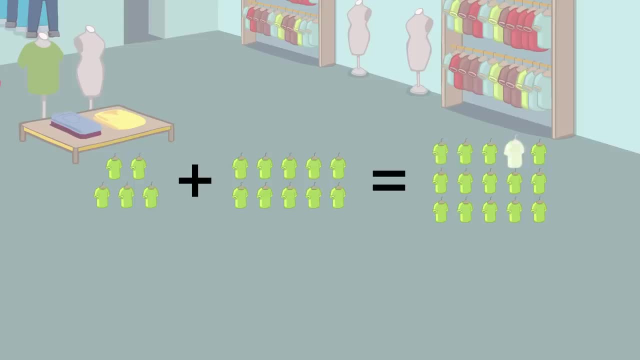 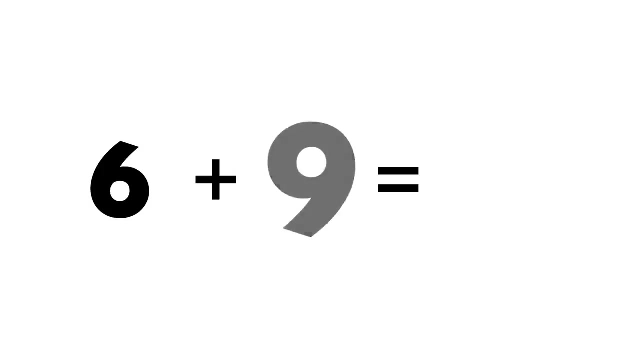 equals 1,, 2,, 3,, 4,, 5,, 6,, 7,, 8,, 9,, 10,, 11,, 12,, 13,, 14,, 15.. 6 plus 9 equals. 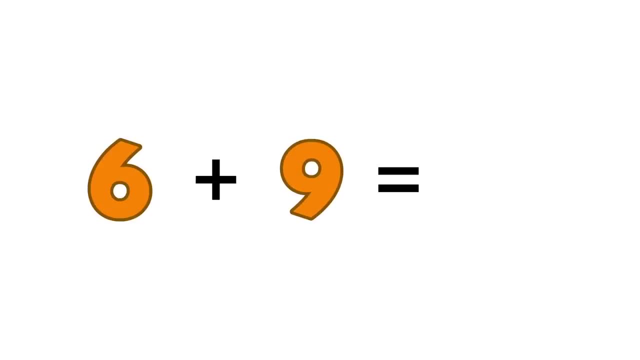 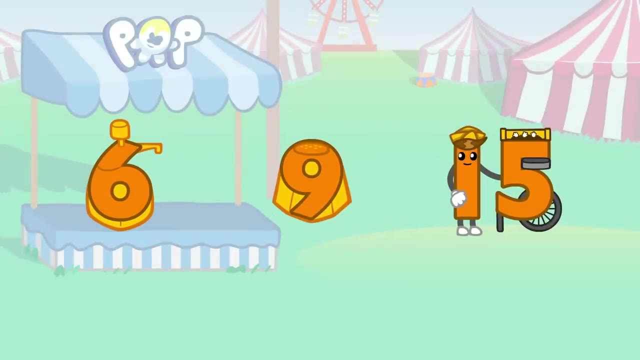 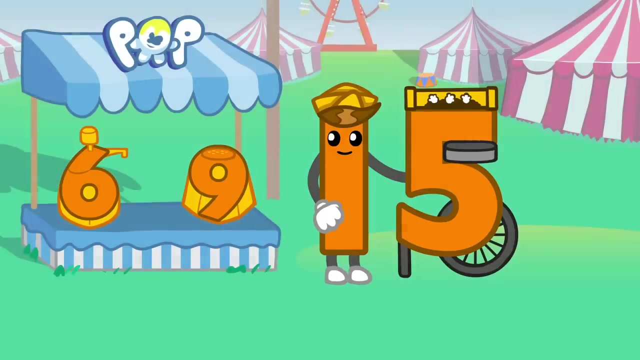 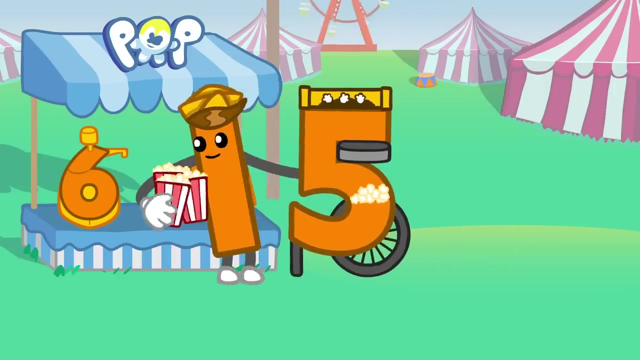 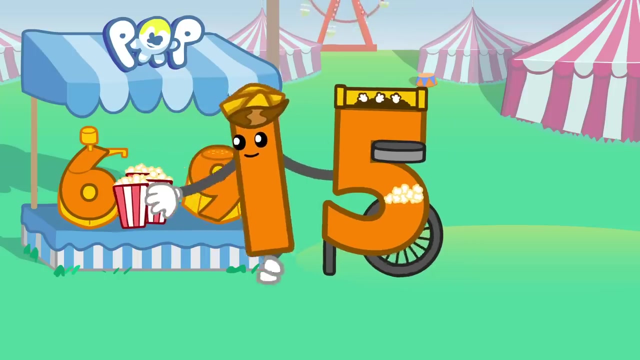 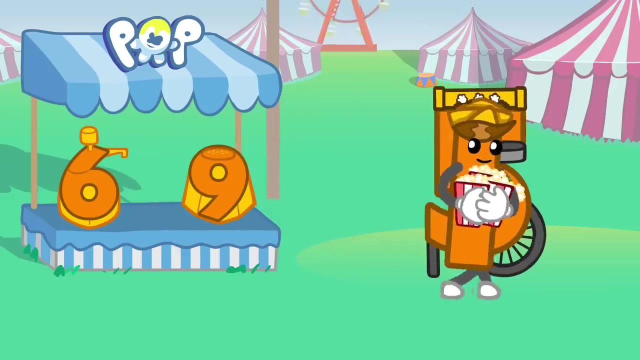 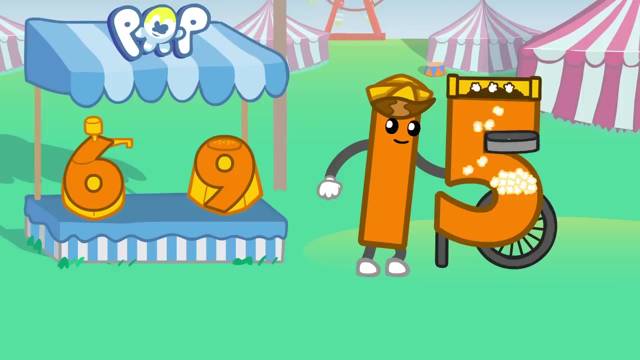 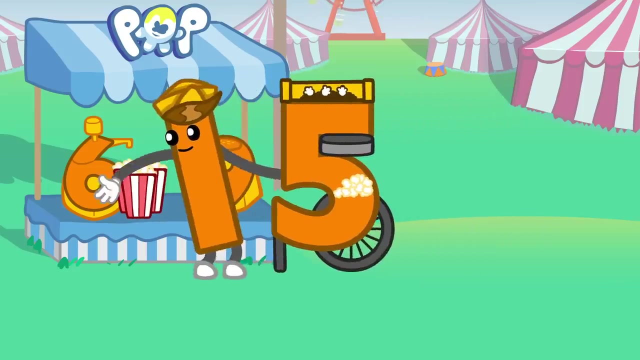 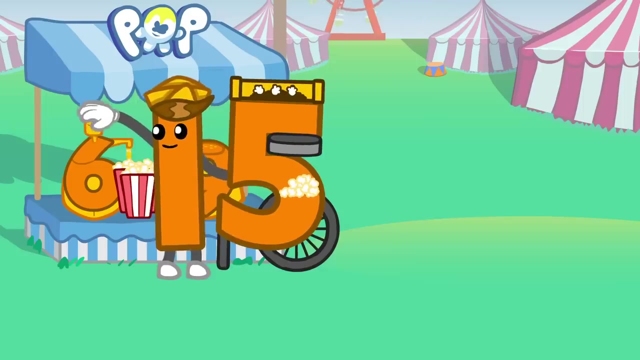 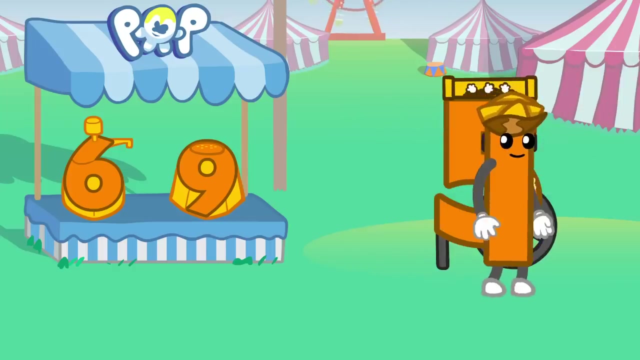 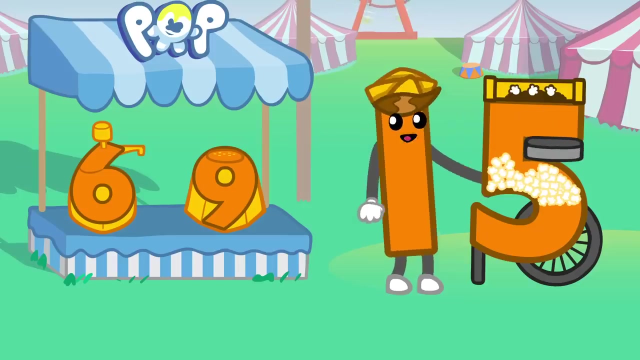 6 plus 9 equals 15!. 6 plus 9 equals 15!. 6 plus 9 equals 15?, 15? Mmm, Ah, Ah, Ah. 6 plus 9 equals 15.. 15.. 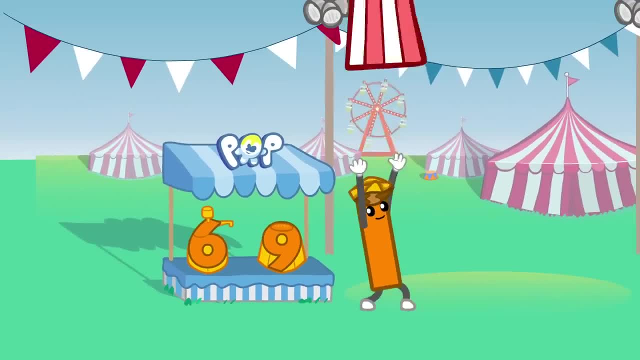 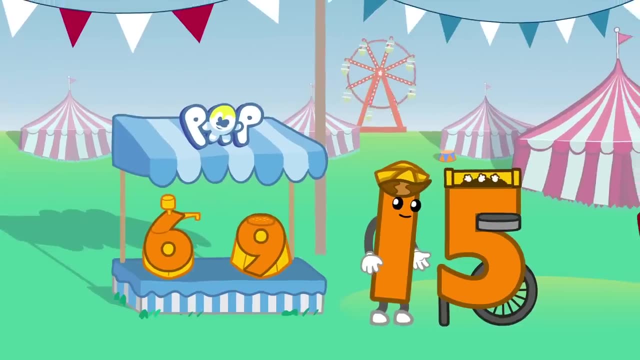 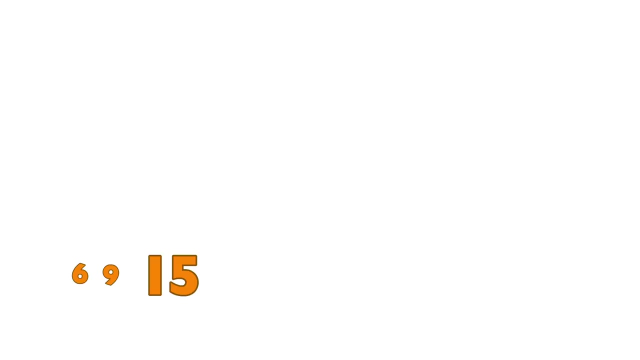 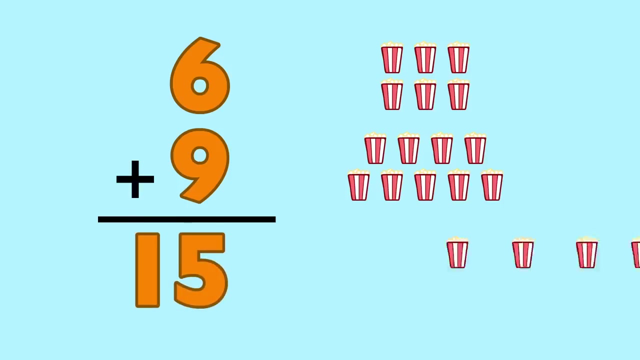 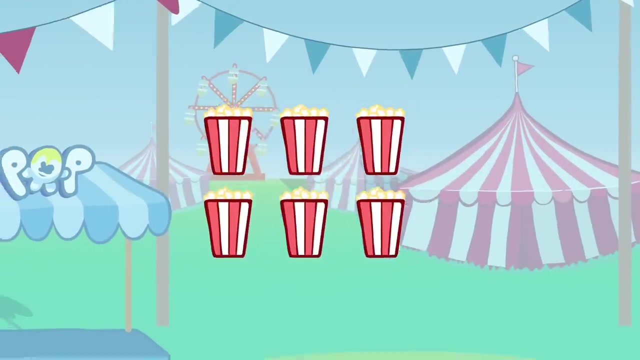 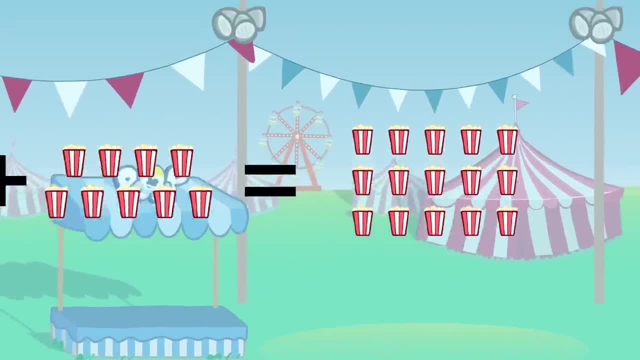 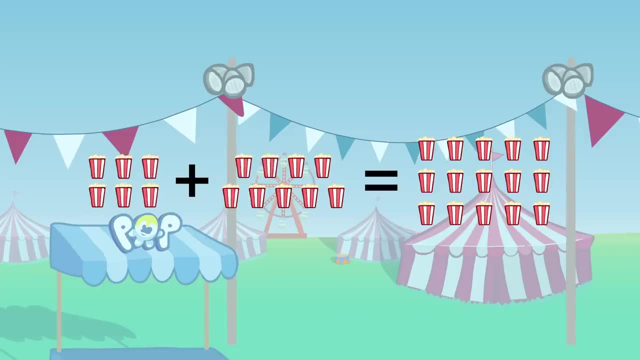 10 plus 9 equals 10.. 1,, 2,, 3,, 4,, 5,, 6,, 7,, 8,, 9,, 10,, 11,, 12,, 13,, 14, 15 equals 1,, 2,, 3,, 4,, 5,, 6,, 7,, 8,, 9,, 10,, 11,, 12,, 13,, 14, 15.. 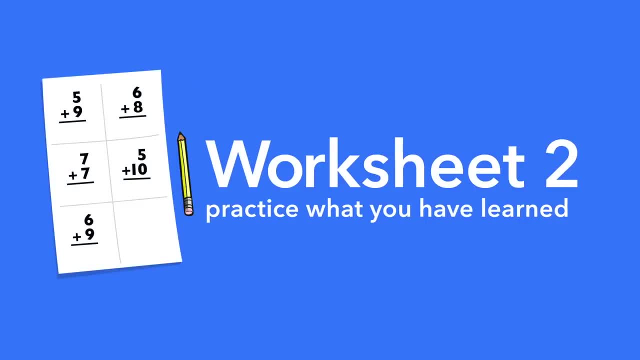 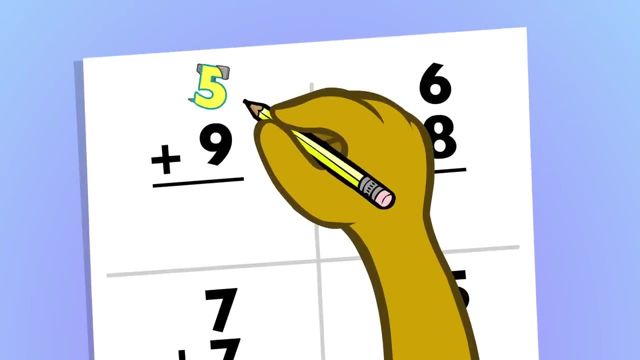 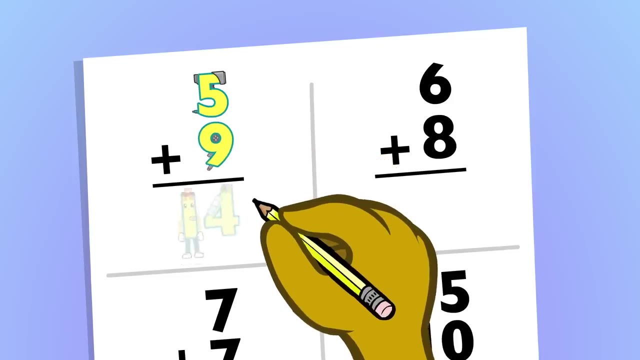 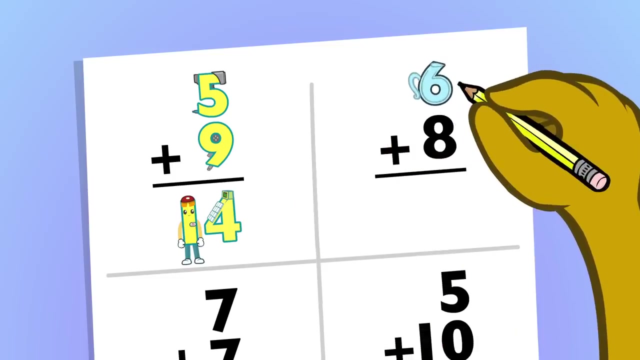 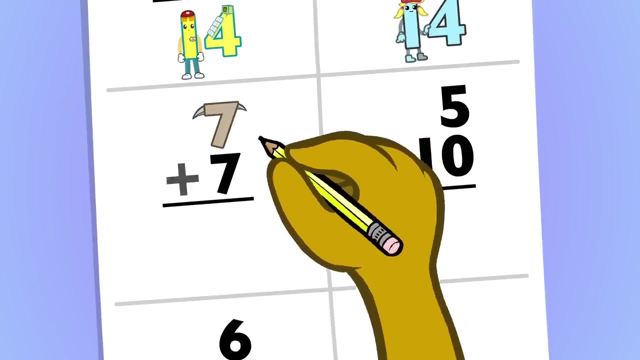 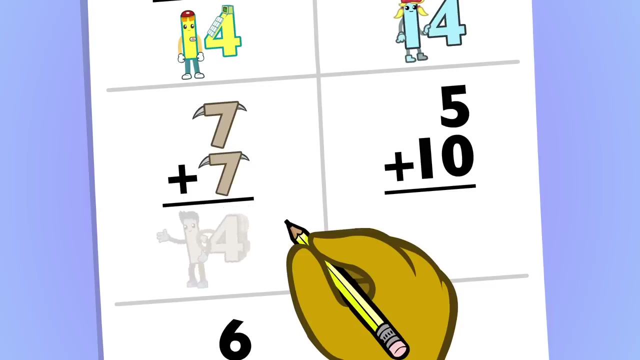 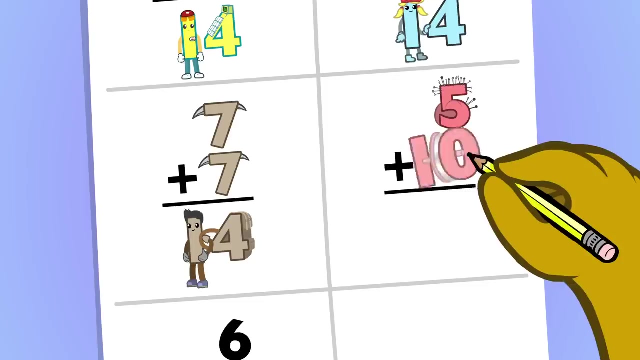 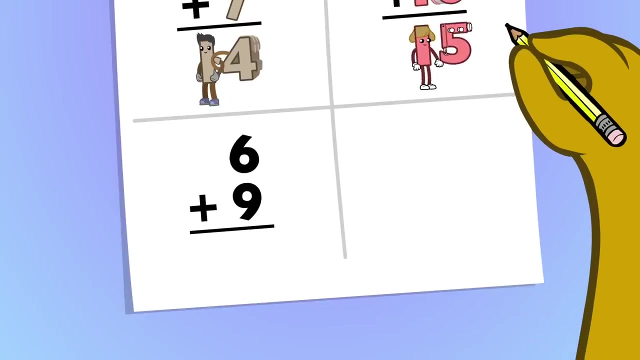 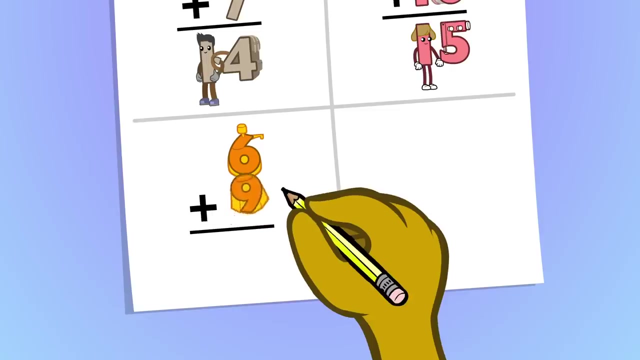 5 plus 9: equals 14. 6 plus 8: equals 14. 7 plus 7: equals 14. 5 plus 10: equals 15. 6 PASS, PASS, PASS 9, 9, PASS 9, 9, 9, 9, 9. 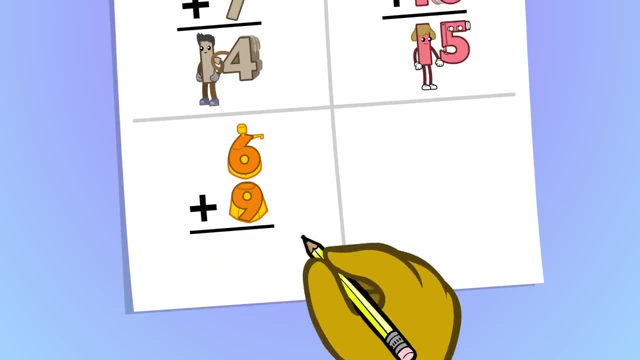 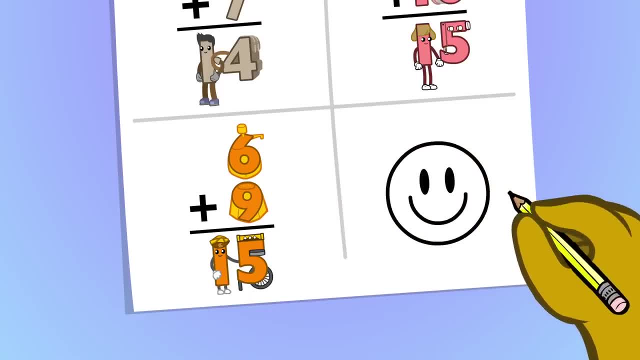 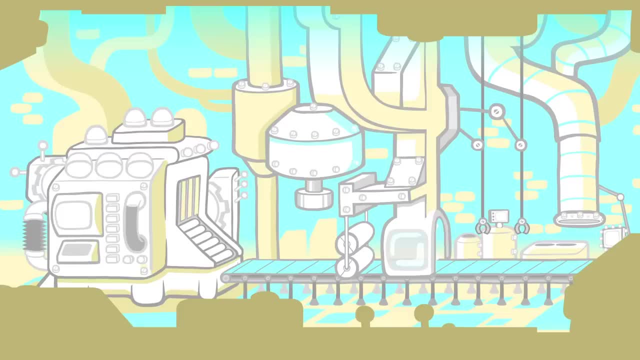 22, 23, 24, 25, 26, 26, 27, 27, 28, 29, 30, 31, 32, 32, 33, 32, 33, 33, 34, 34, 35, 36, 37, 38, 39, 40. 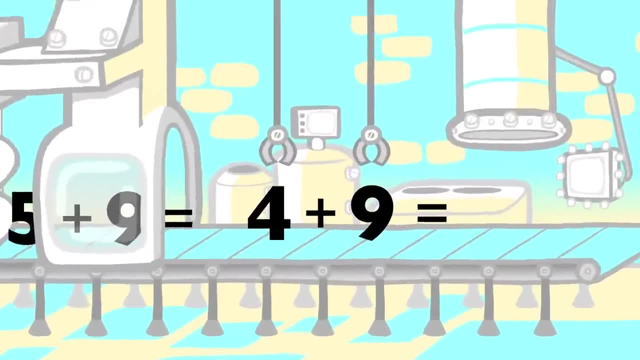 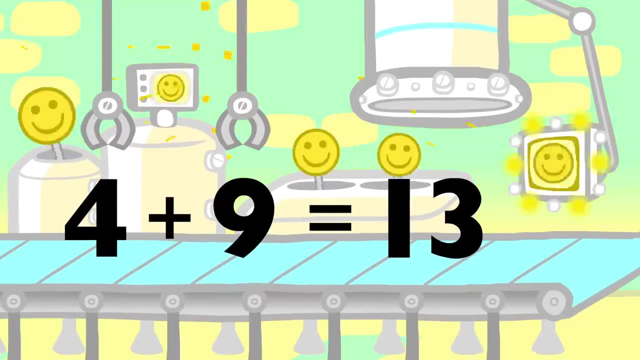 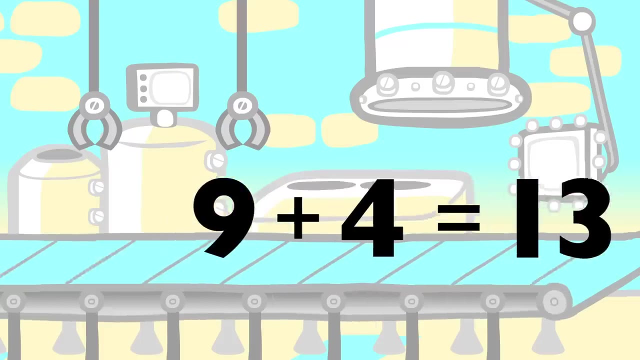 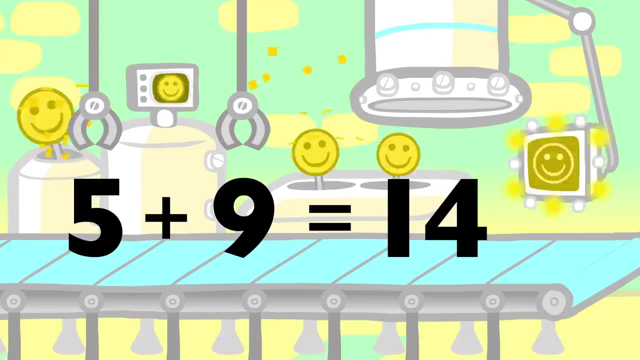 42, 43, 44, 45, 46, 47, 48, 49, 50, 51, 52, 53, 54, 55, 56, 57, 58, 59, 60, 61, 62, 63, 63, 64, 64, 64. 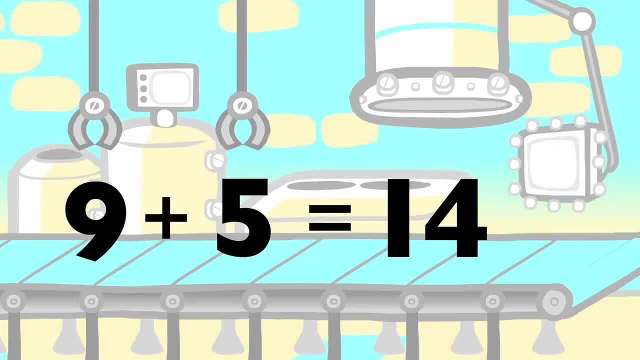 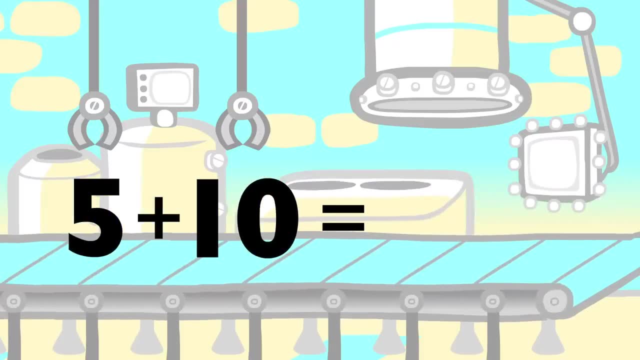 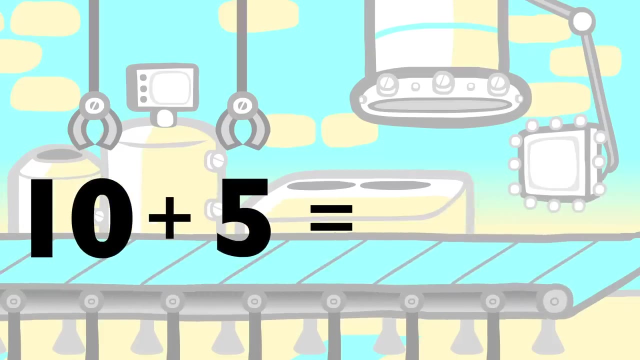 65, 66, 66, 67, 68, 69, 69, 70, 71, 72, 72, 73, 74, 75, 76, 77, 78, 79, 79, 80, 80, 81, 82, 83, 83, 84. 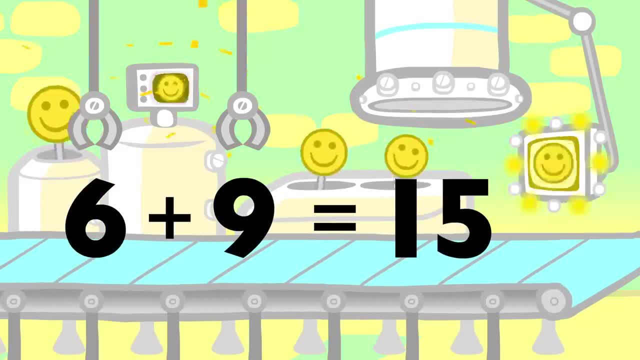 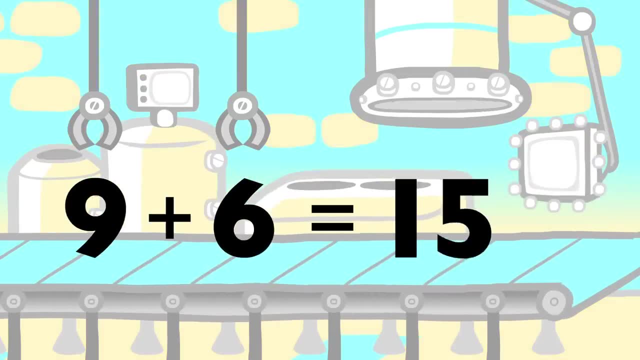 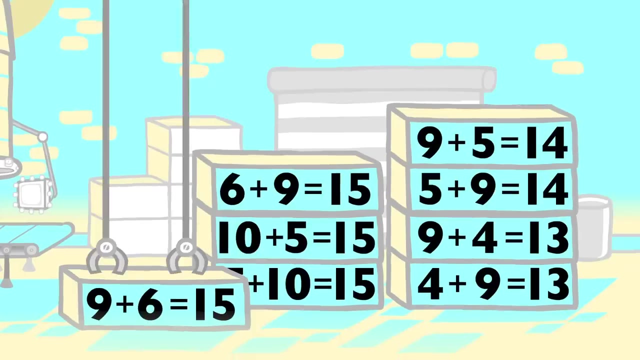 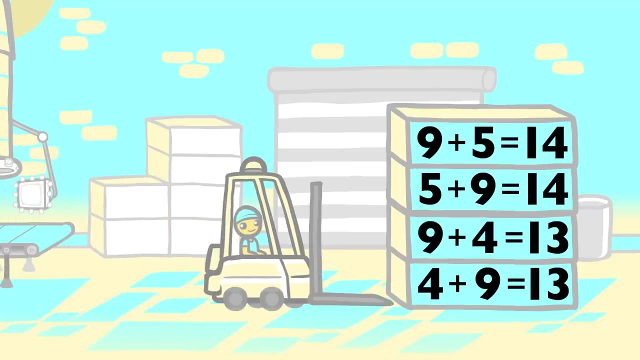 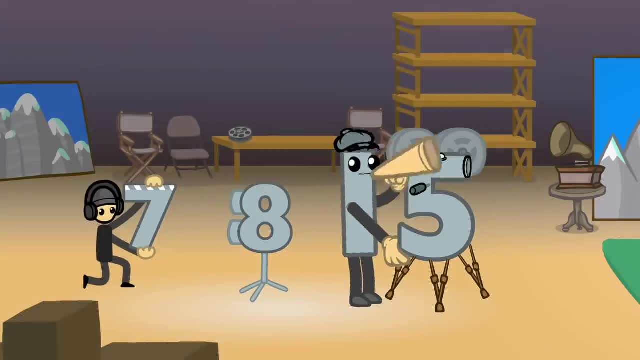 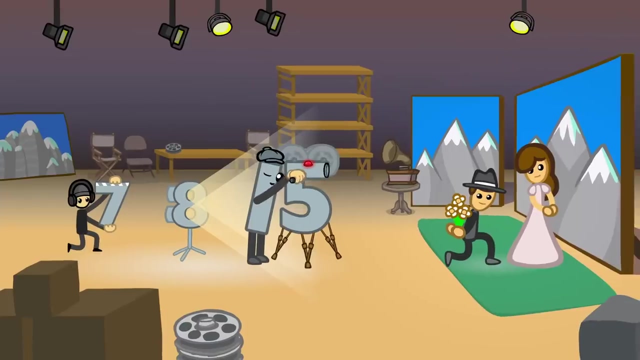 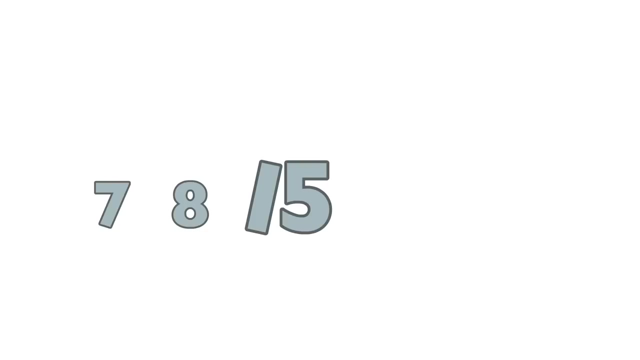 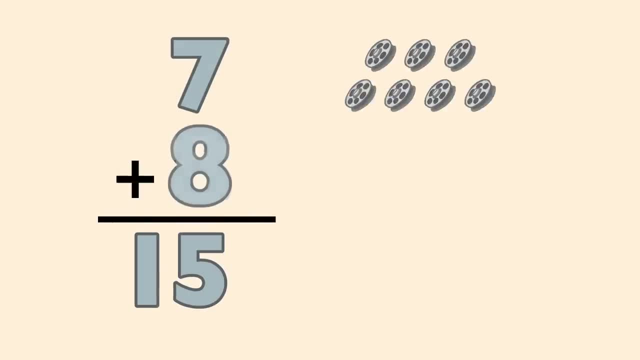 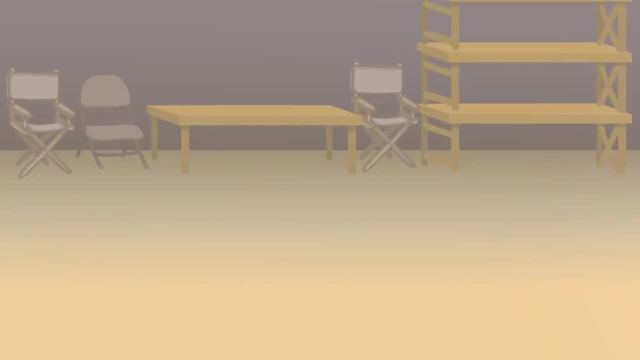 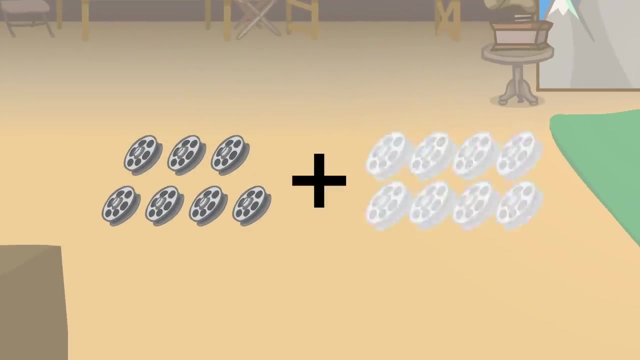 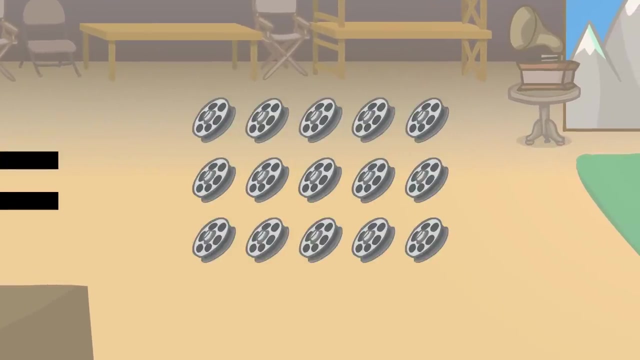 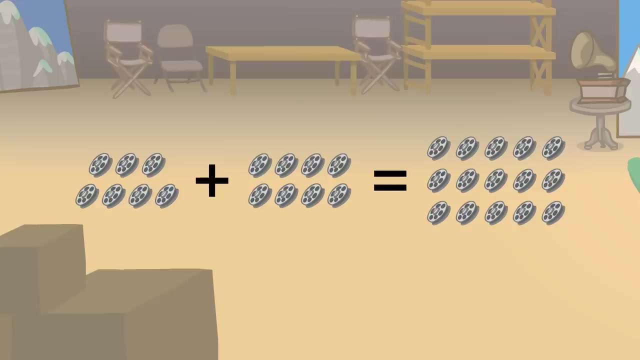 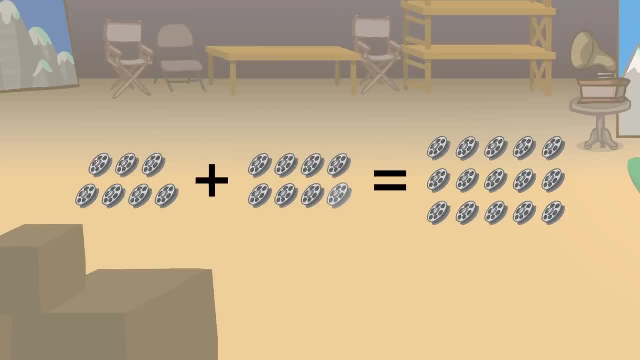 6 plus 10 equals zero. Is there jumbo: 1,, 2,, 3, 4,, 5,, 6,, 7,, 8,, 9,, 10,, 11,, 12,, 13,, 14,, 15, equals. 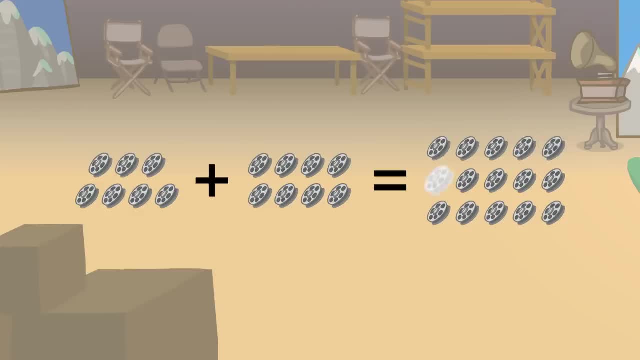 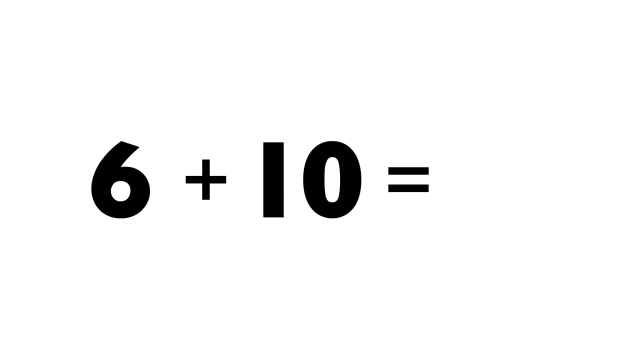 1,, 2,, 3, 4,, 5,, 6,, 7,, 8,, 9,, 10,, 11,, 12, 13,, 14, 15, 6 plus 10 equals Six plus ten equals sixteen. 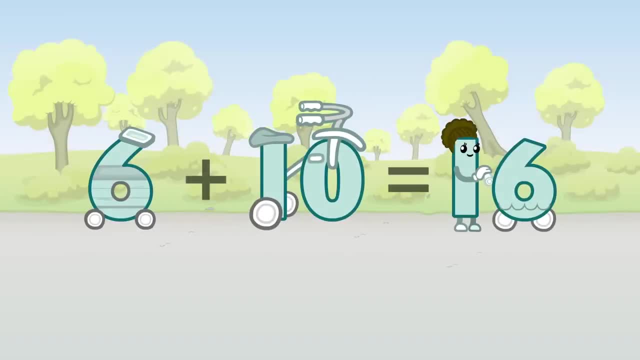 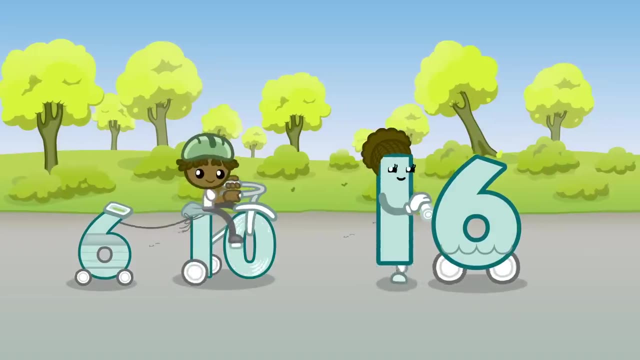 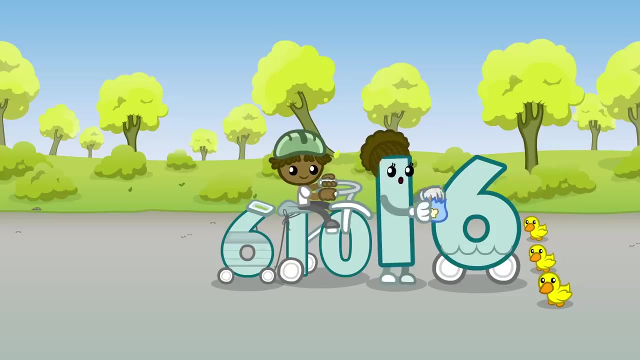 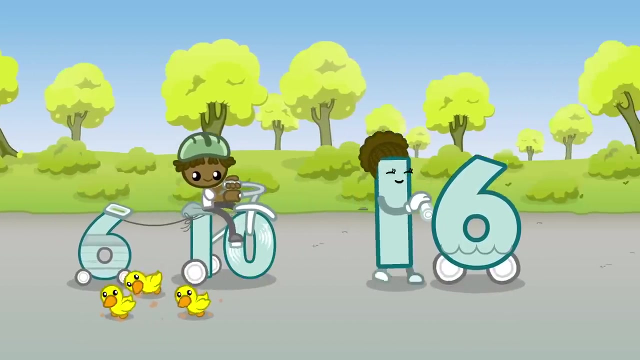 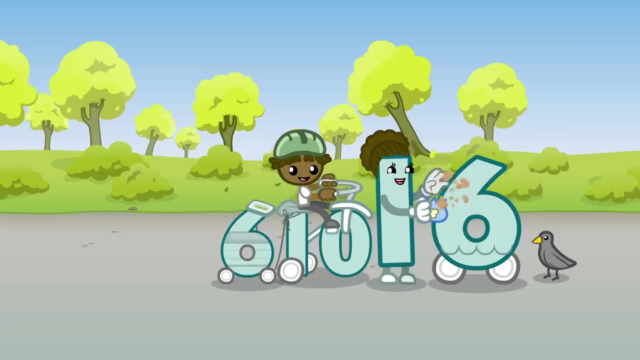 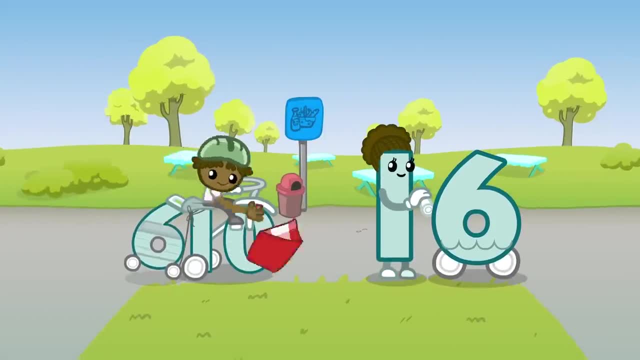 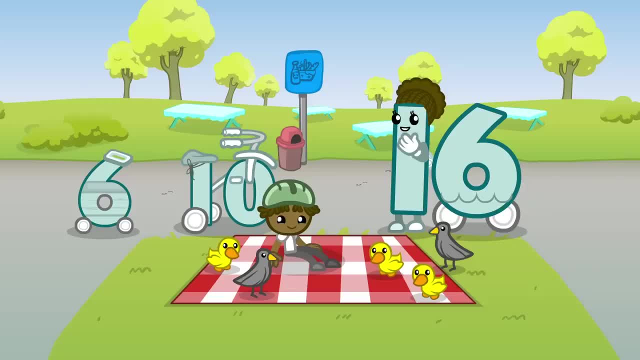 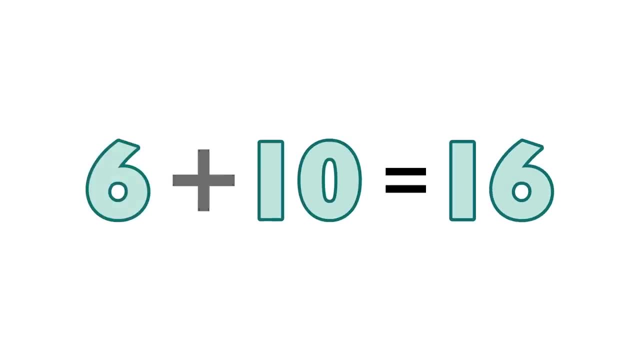 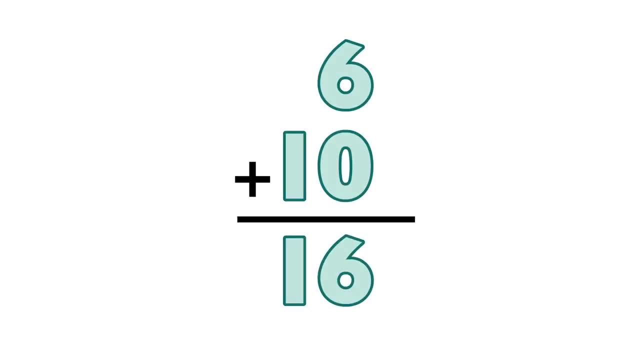 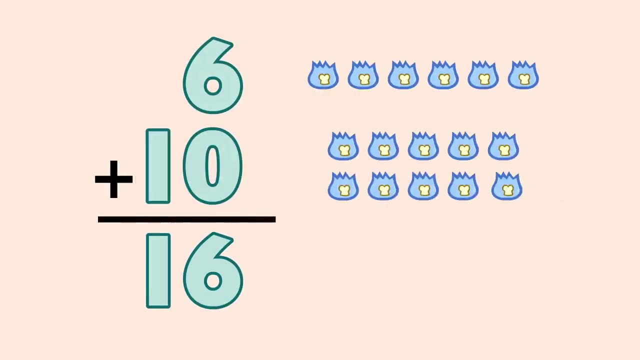 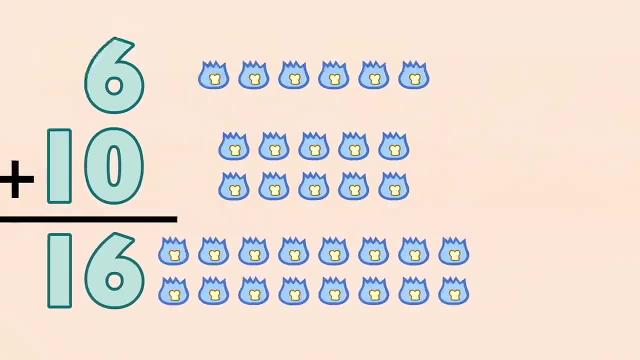 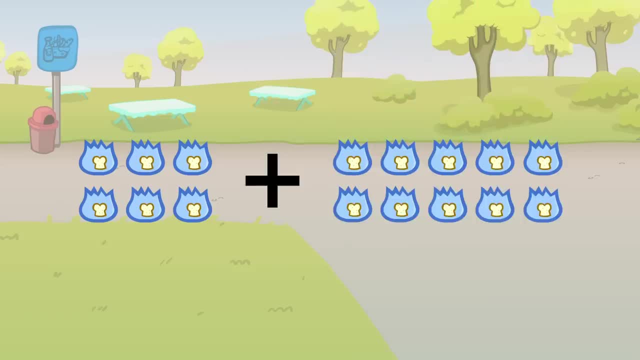 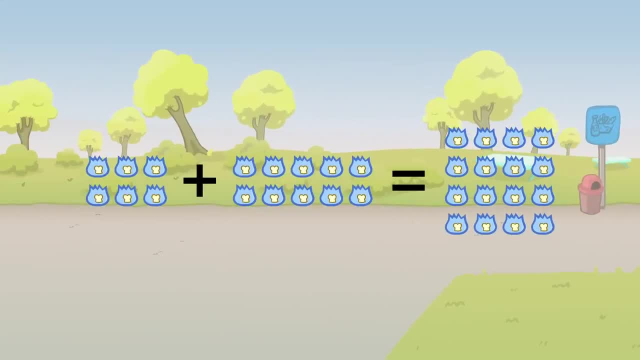 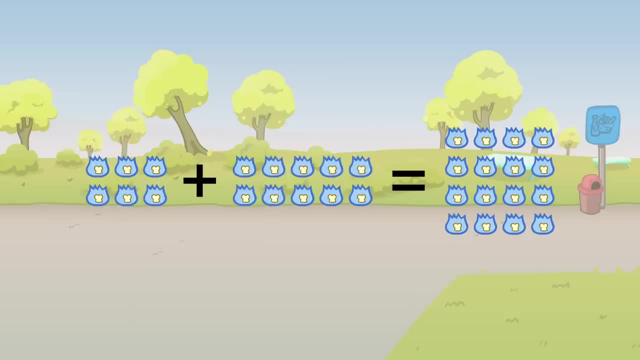 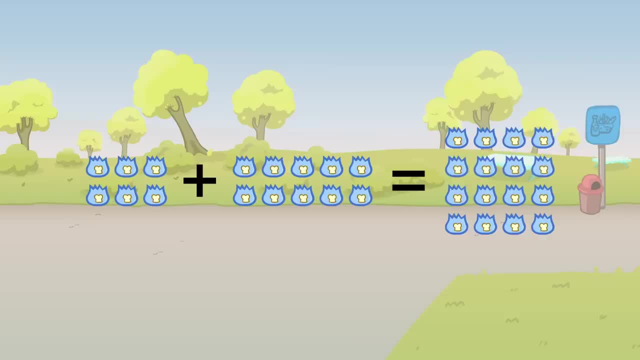 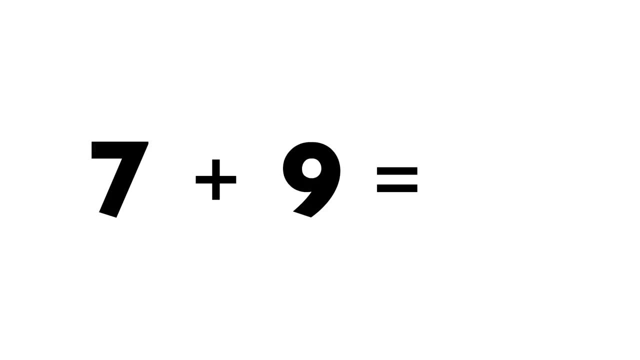 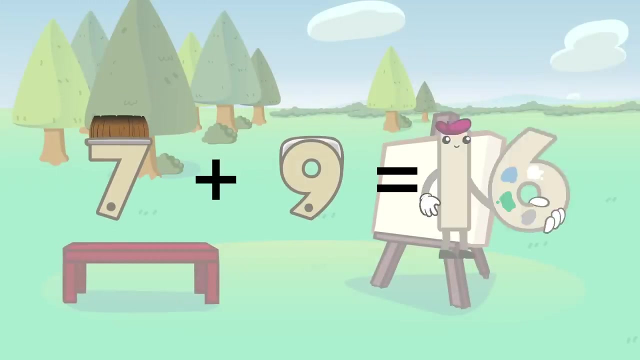 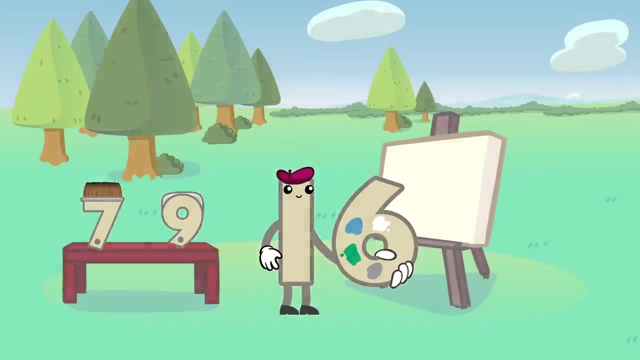 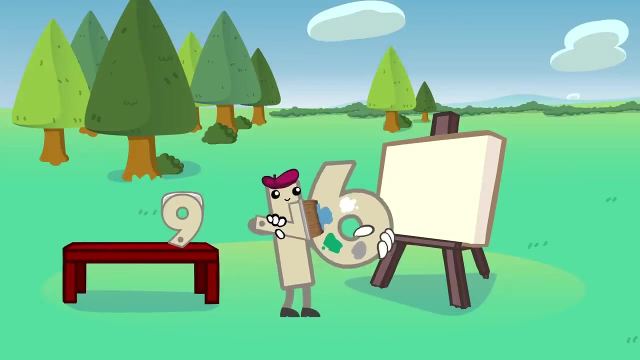 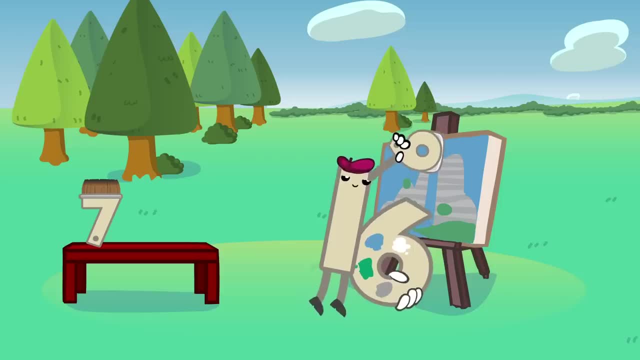 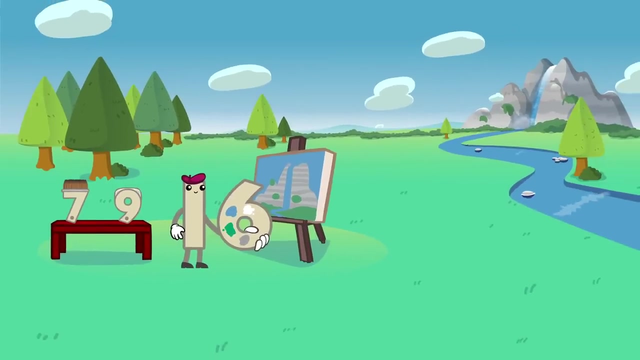 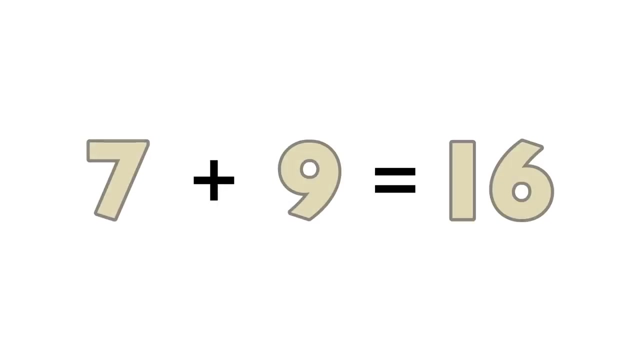 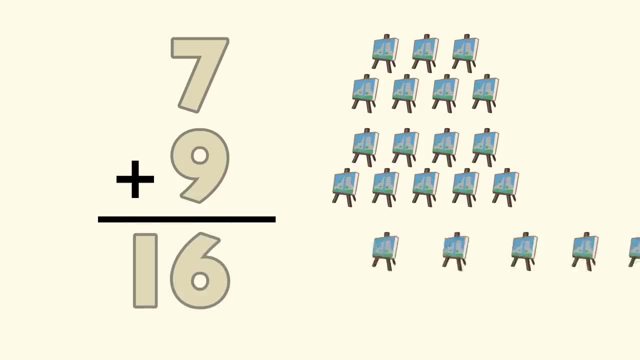 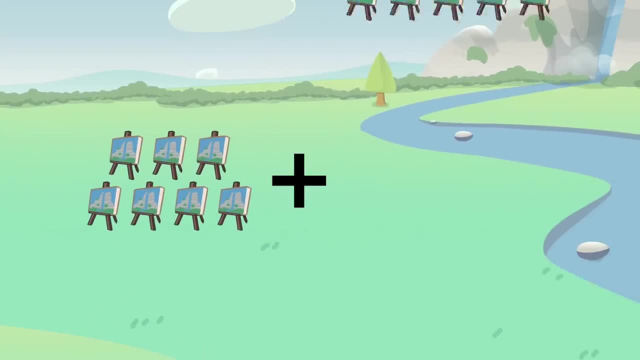 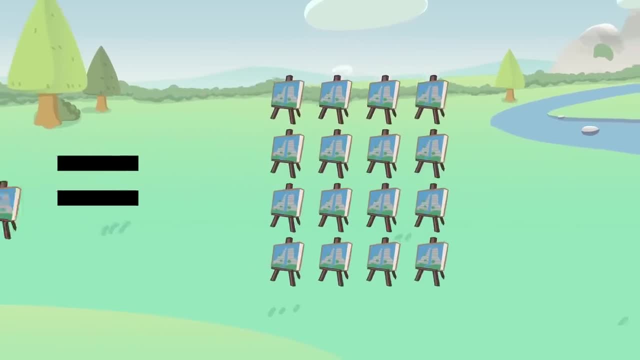 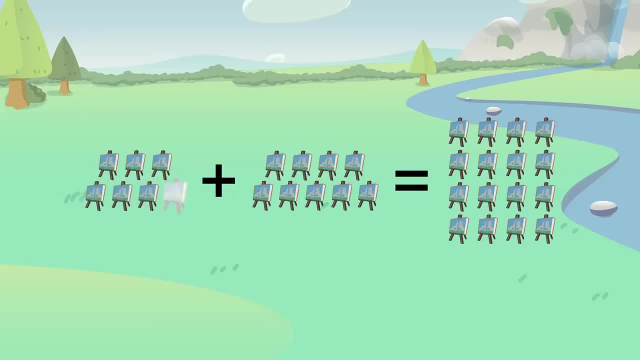 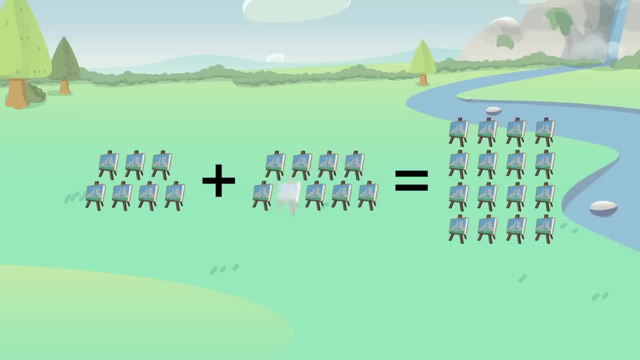 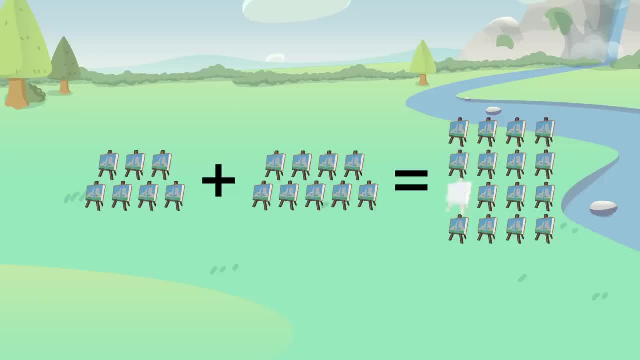 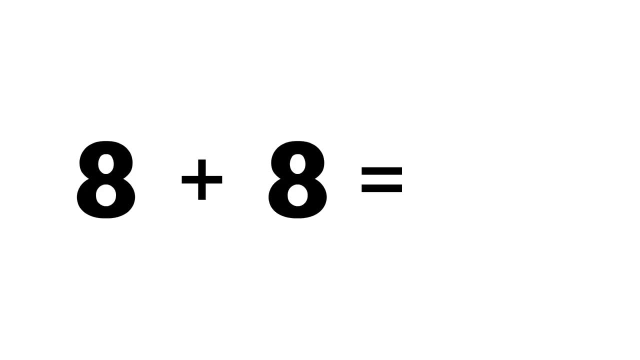 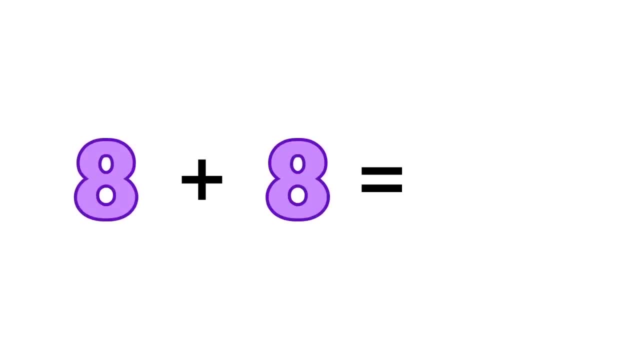 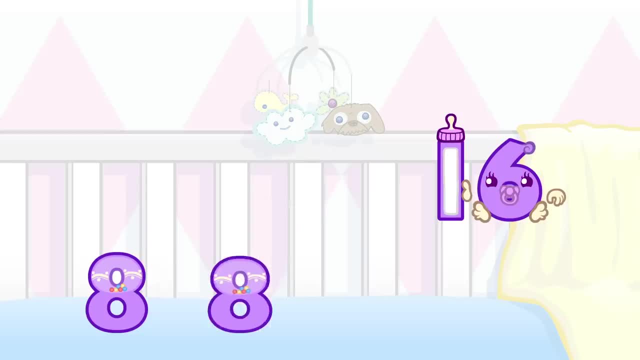 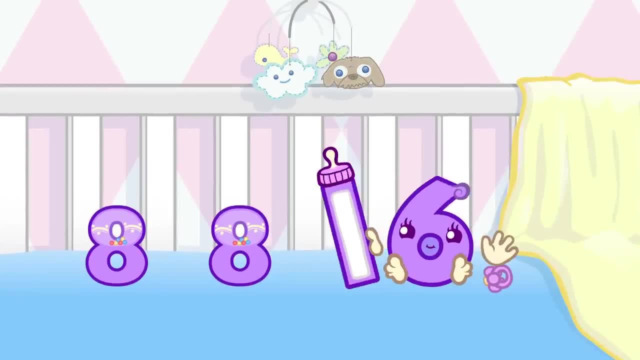 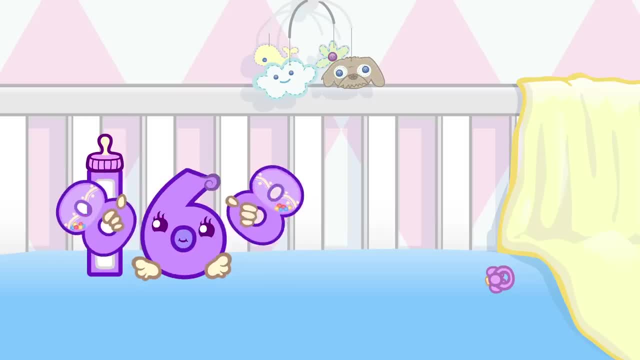 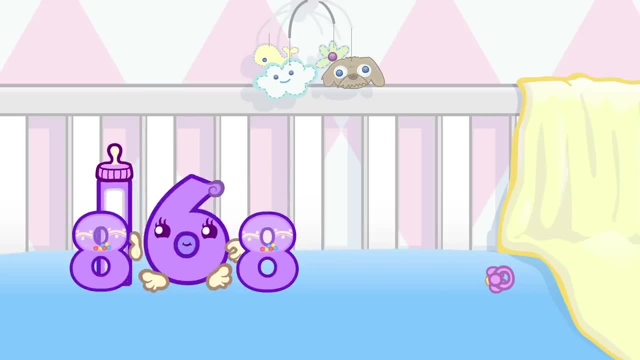 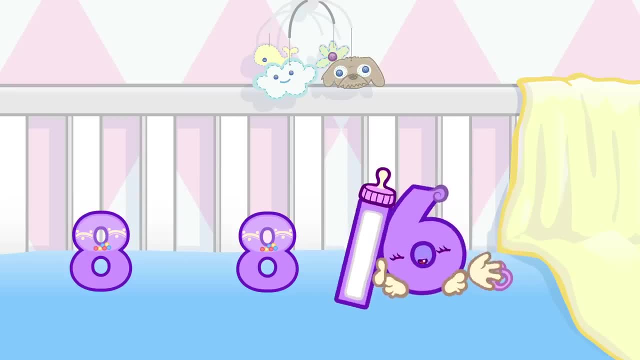 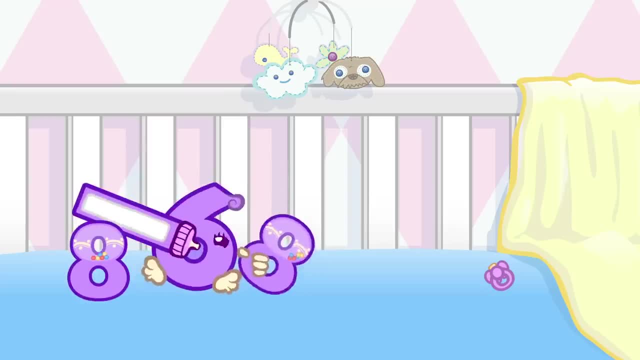 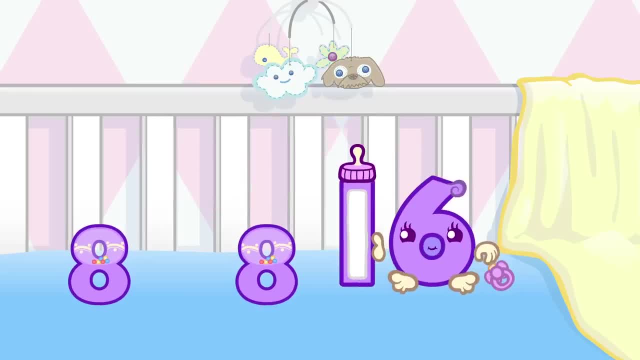 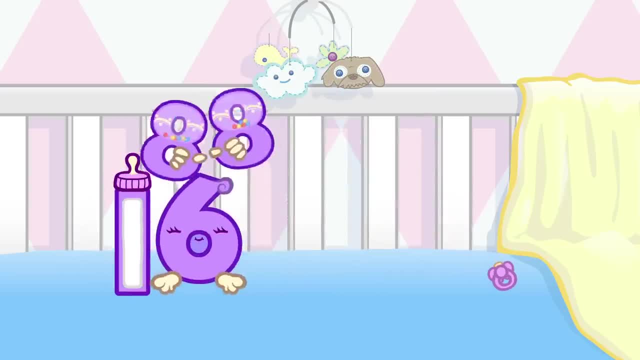 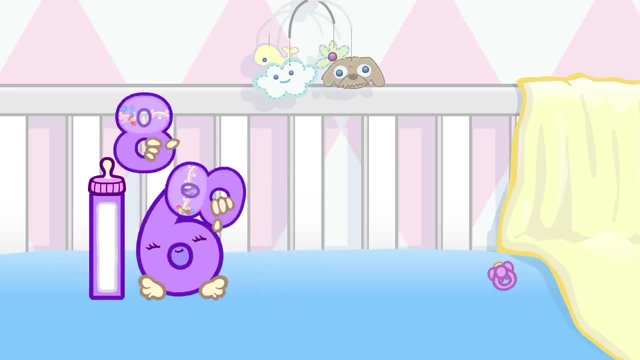 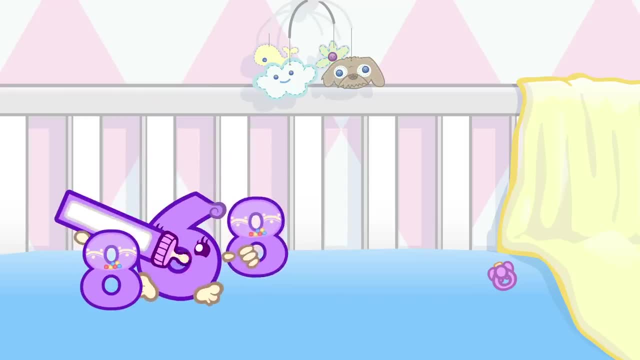 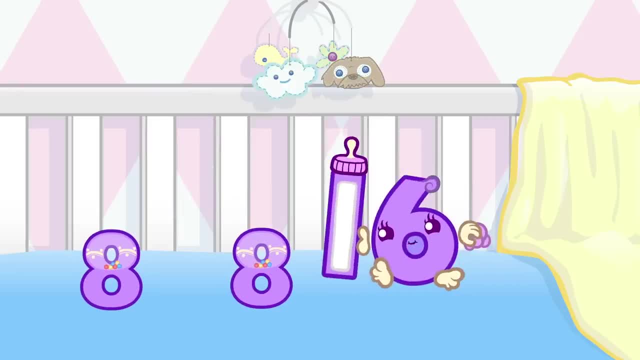 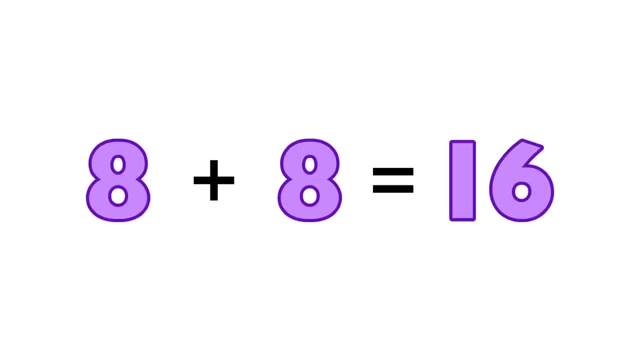 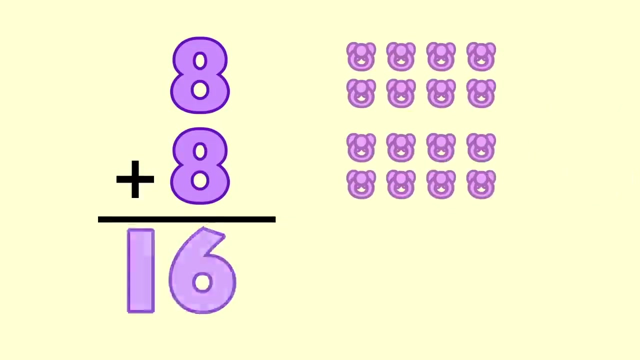 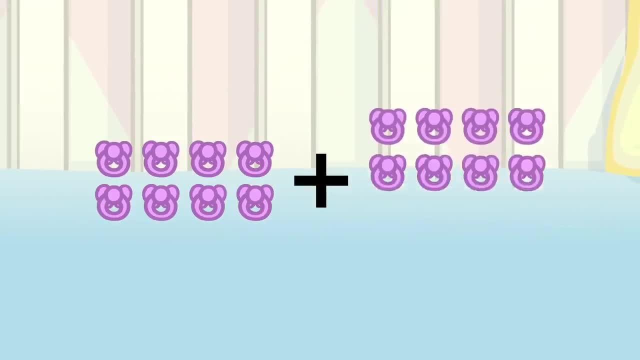 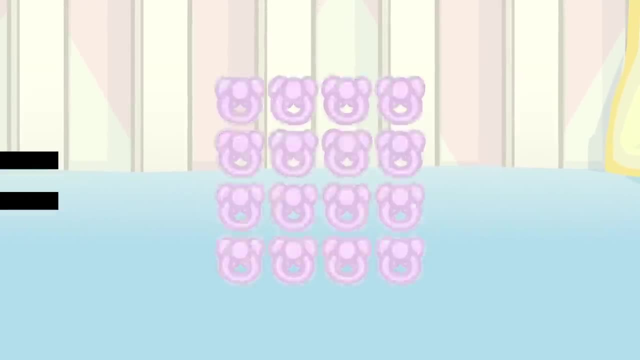 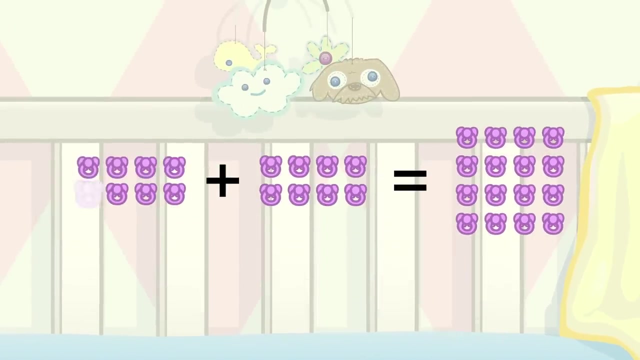 Eight plus eight equals sixteen: One, two, three, four, five, six, seven, eight, nine, ten, eleven, twelve, thirteen, fourteen, fifteen, sixteen equals one, two, three, four, five, six, seven, eight, nine, ten, eleven, twelve, thirteen, fourteen, fifteen, sixteen. 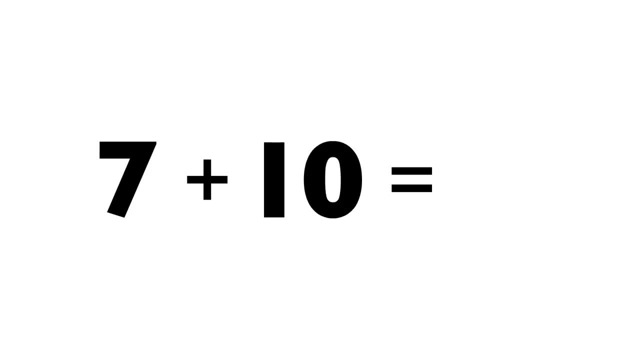 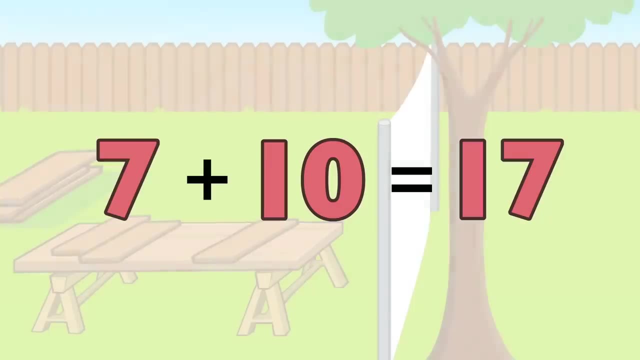 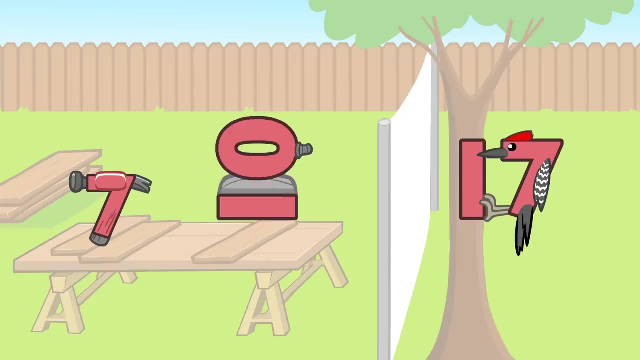 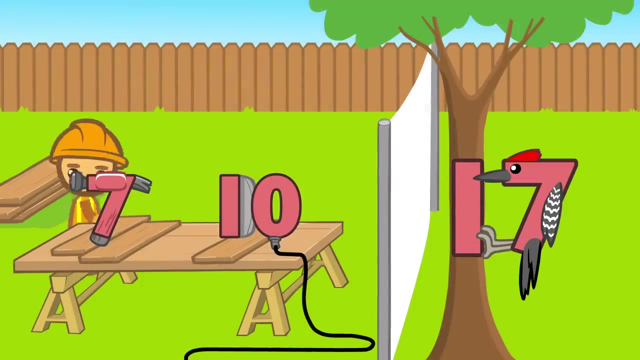 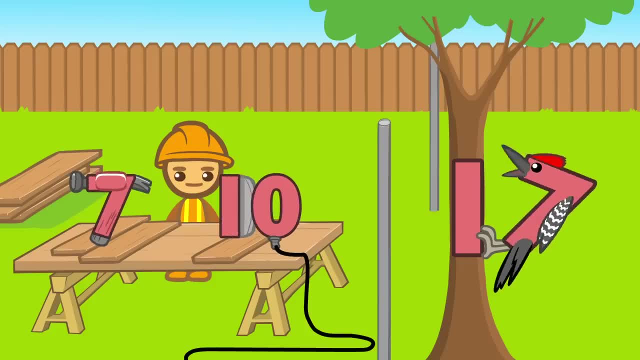 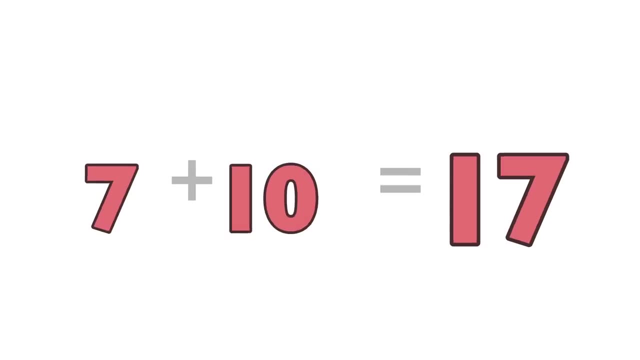 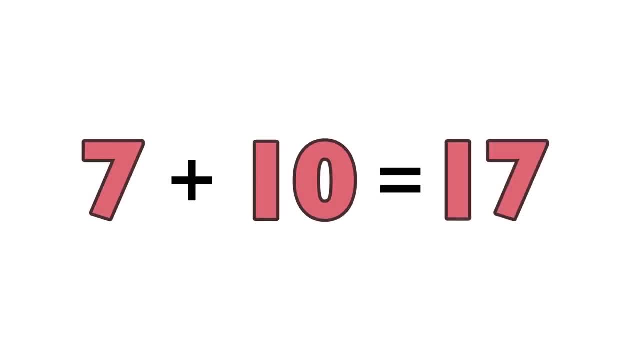 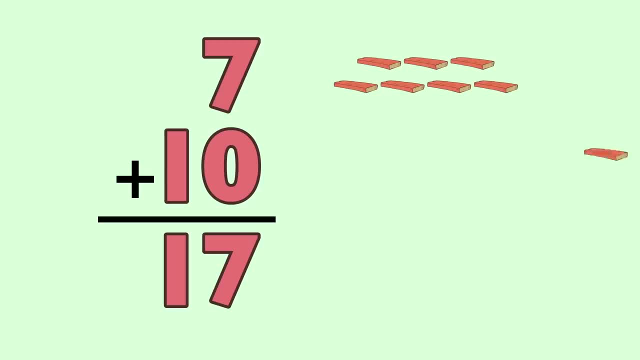 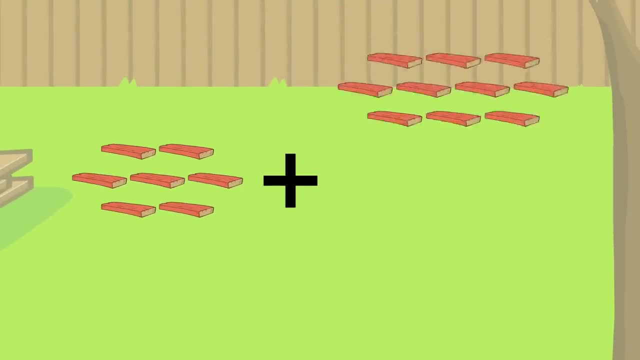 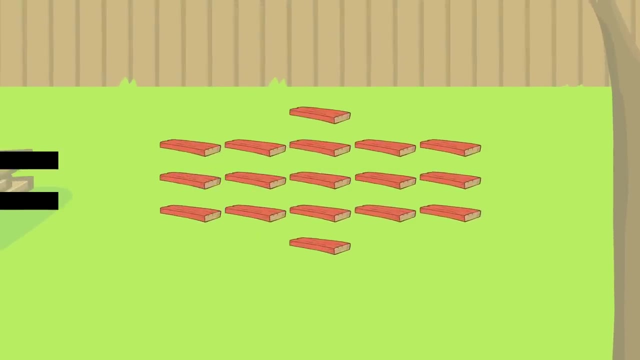 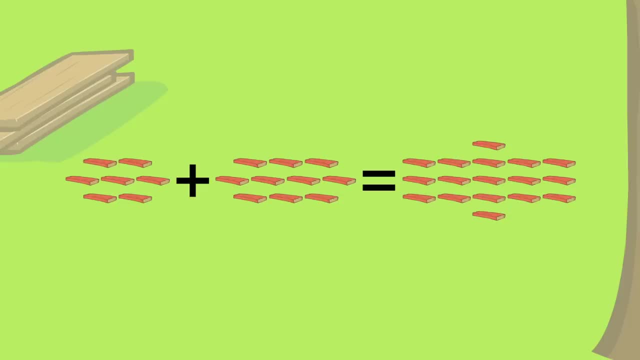 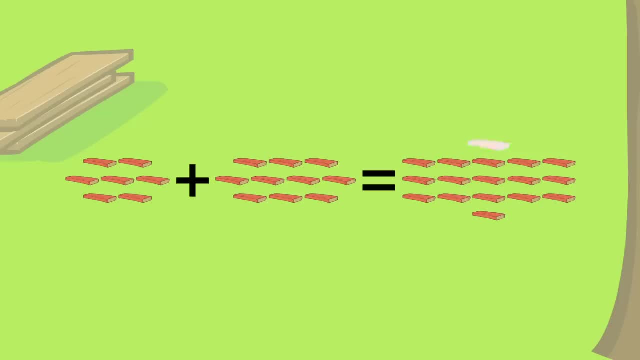 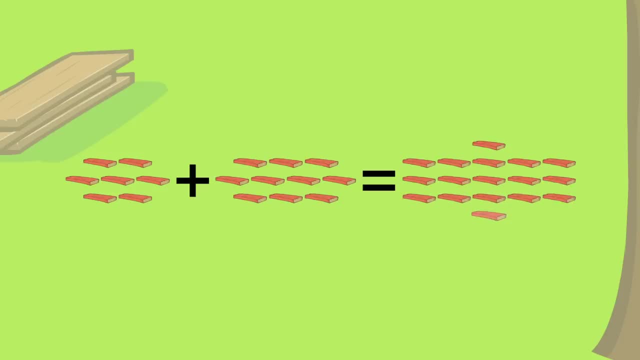 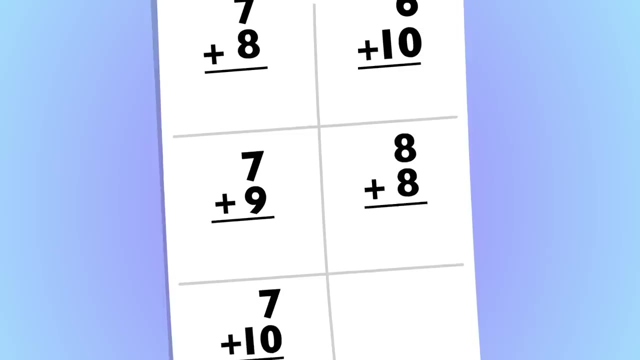 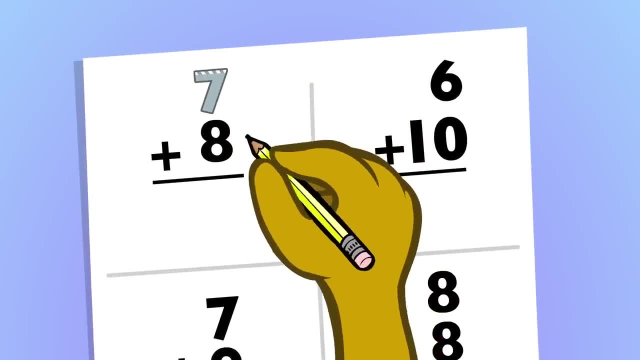 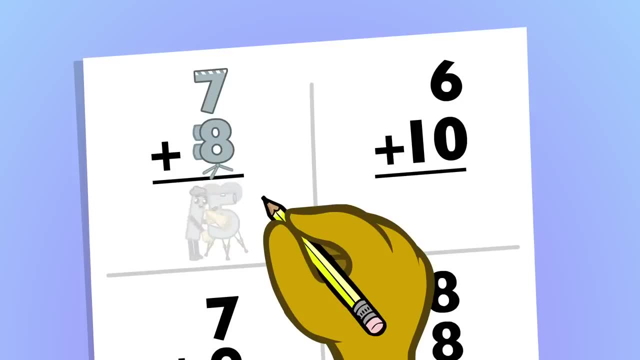 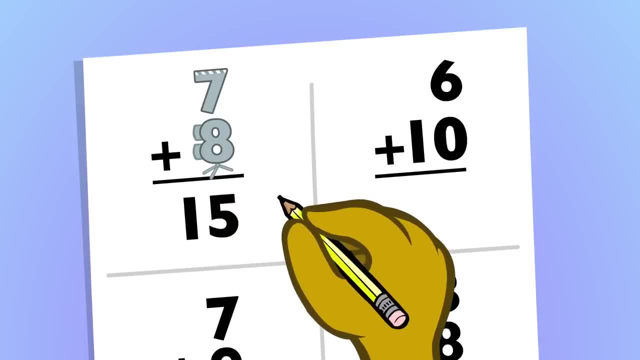 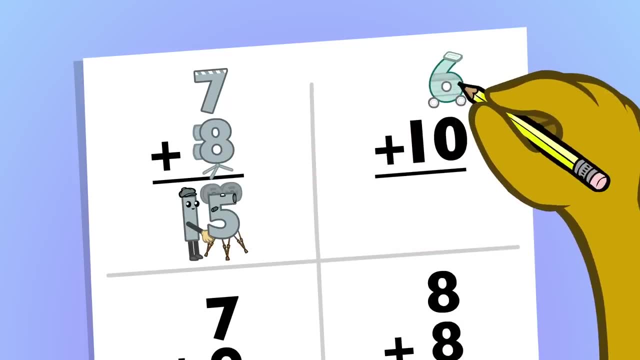 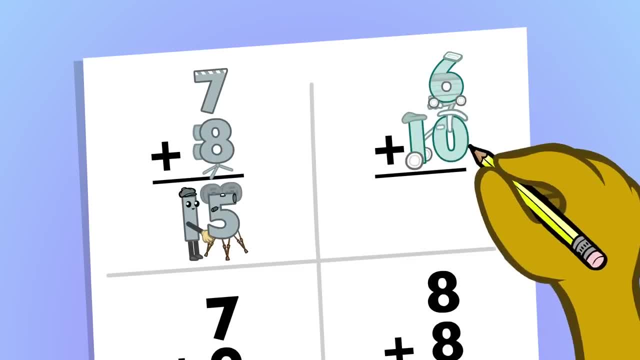 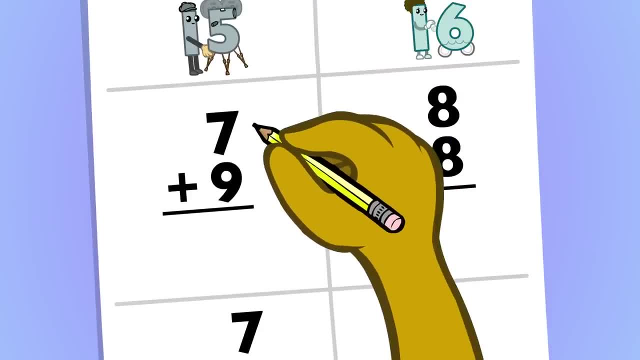 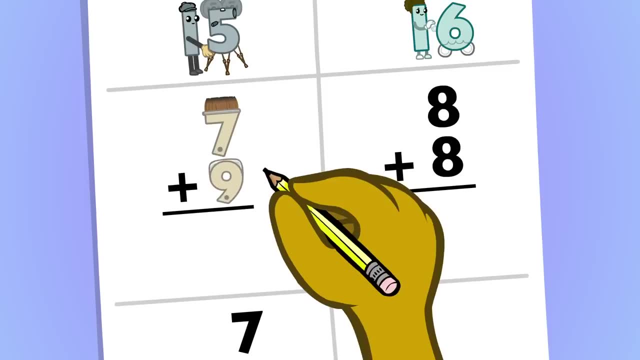 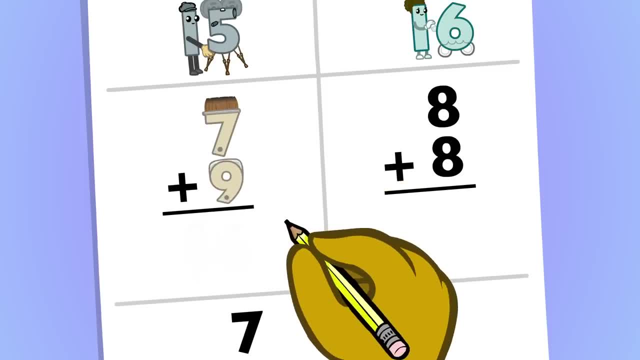 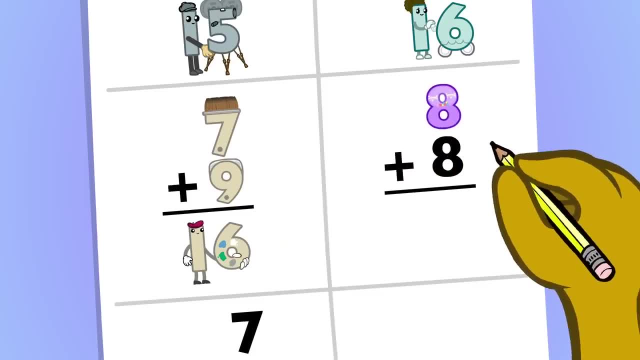 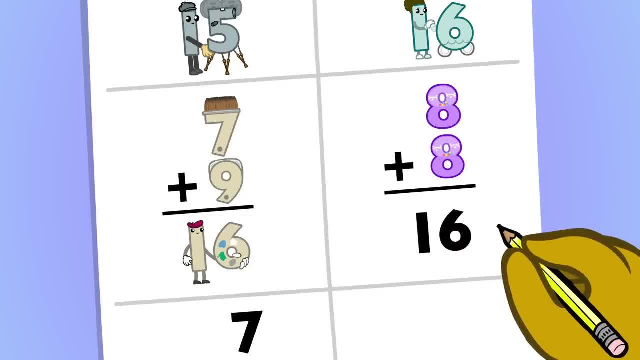 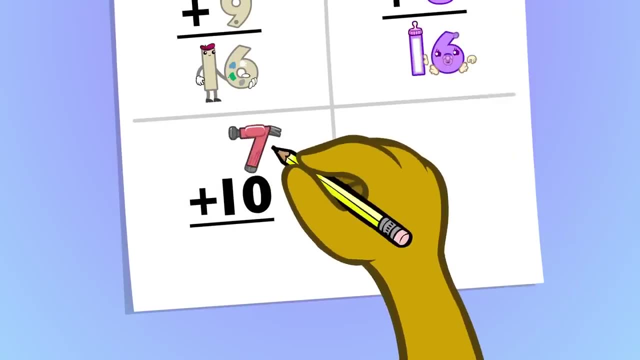 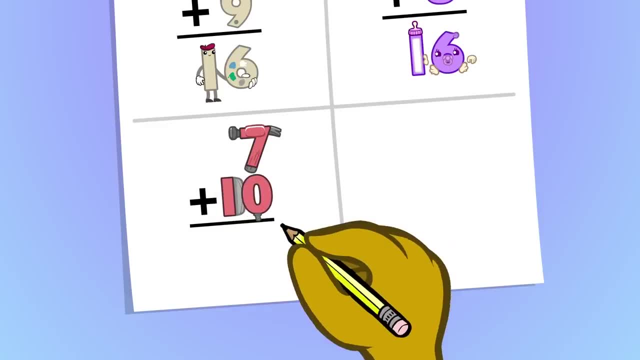 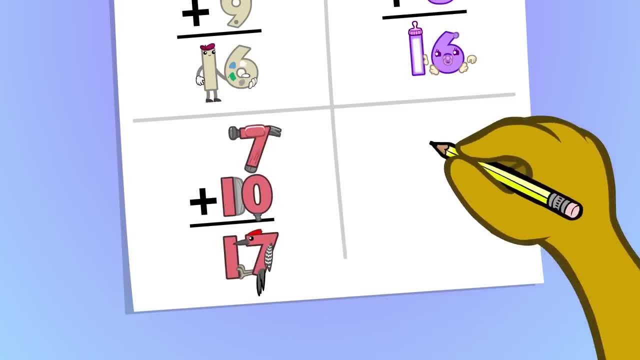 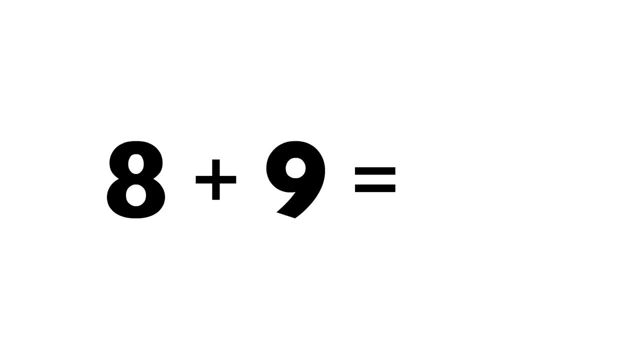 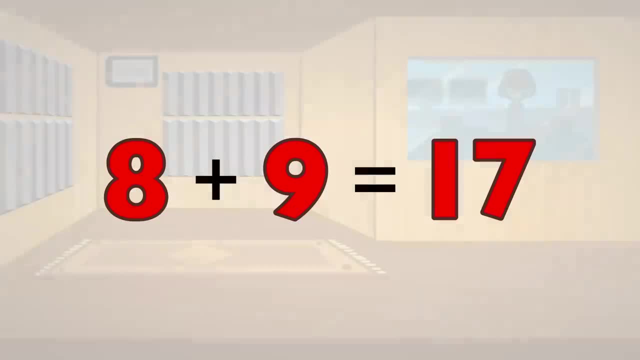 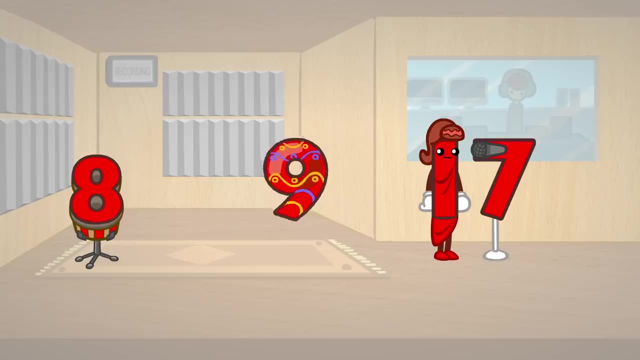 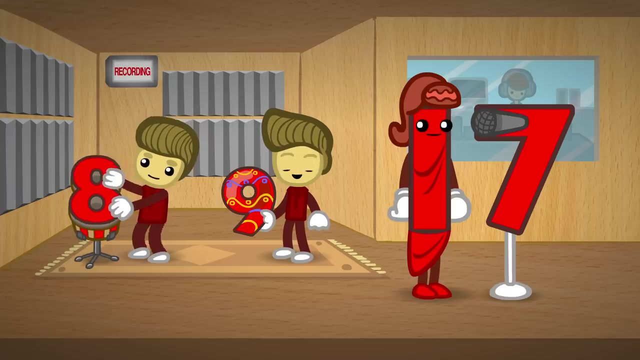 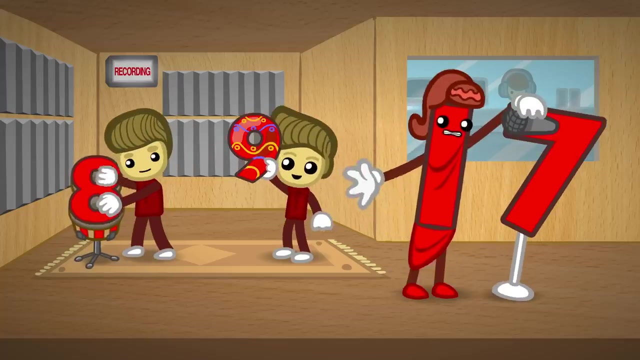 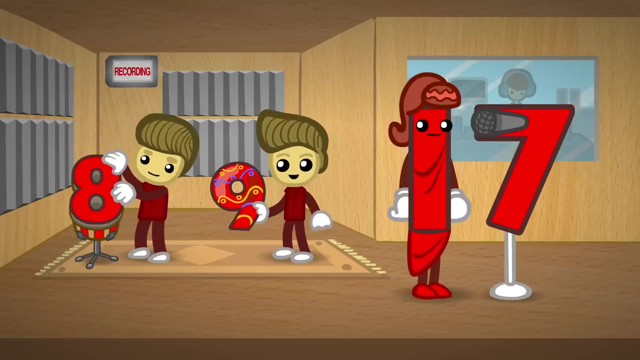 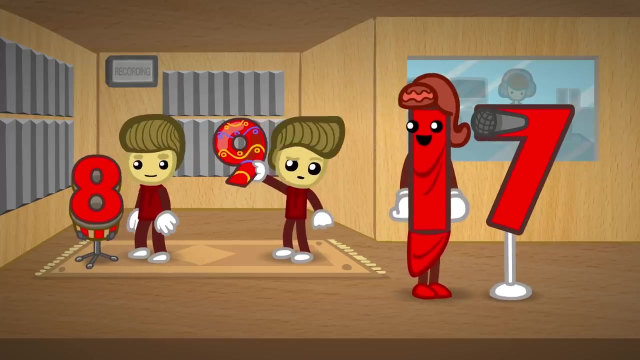 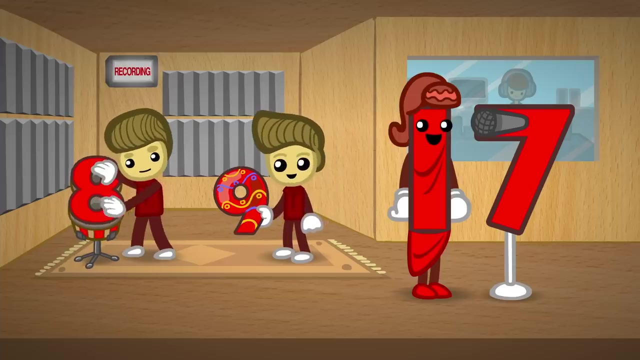 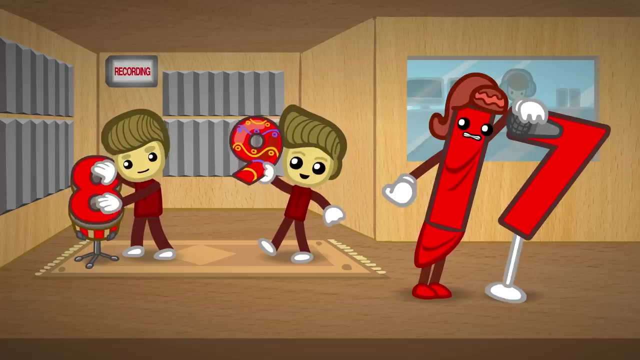 7 plus 10 equals 17.. SEVENTEEN EIGHT PLUS NINE EQUALS SEVENTEEN EIGHT PLUS NINE EQUALS. SEVENTEEN. 8 plus 9 equals 17. 8 plus 9 equals 17. 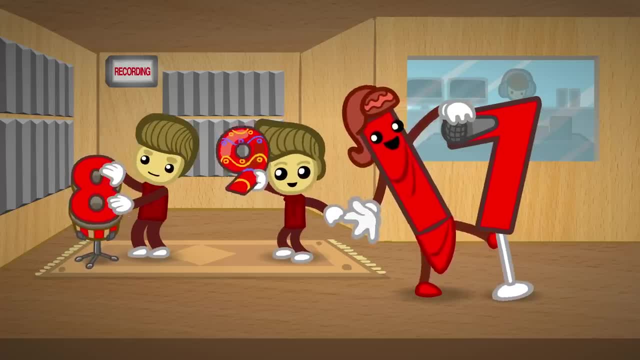 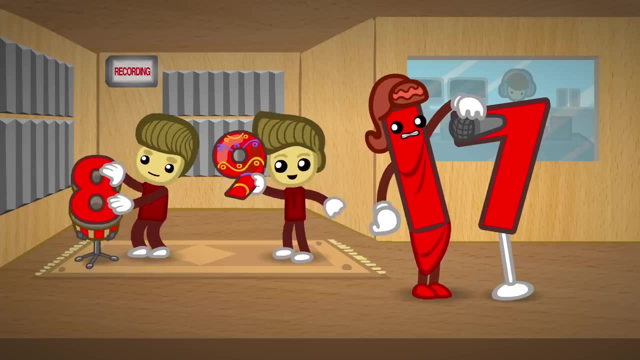 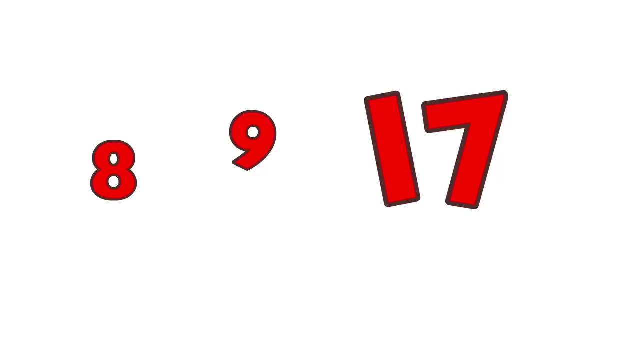 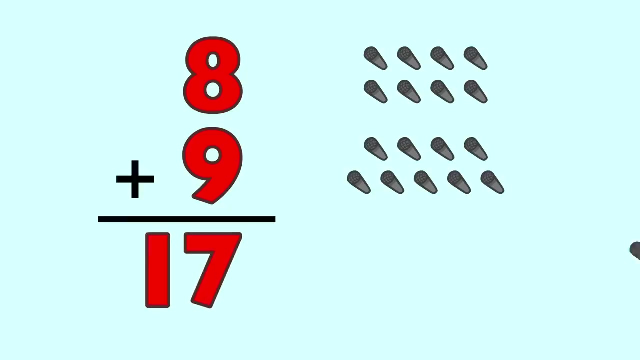 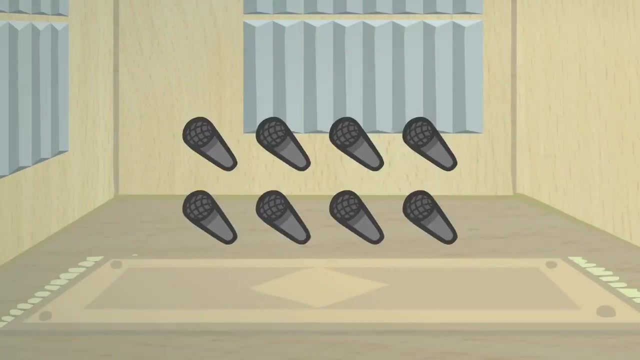 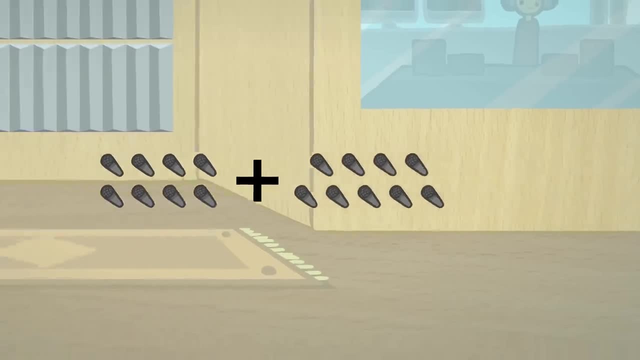 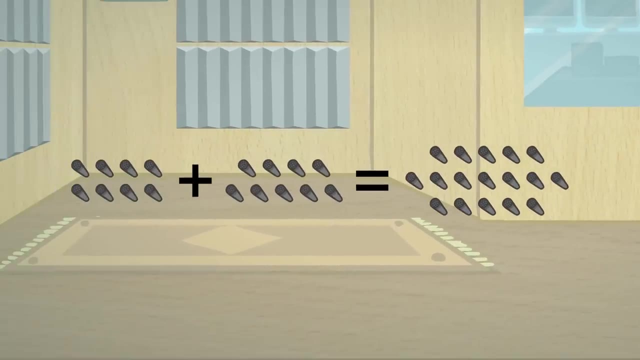 8 plus 9 equals 17: 1,, 2,, 3,, 4,, 5,, 6,, 7,, 8,, 9,, 10,, 11,, 12,, 13,, 14,, 15,, 16, 17. 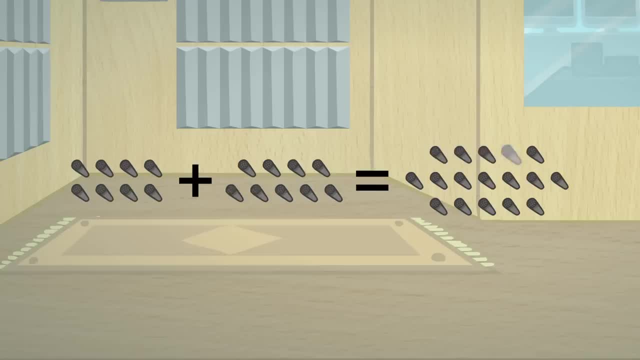 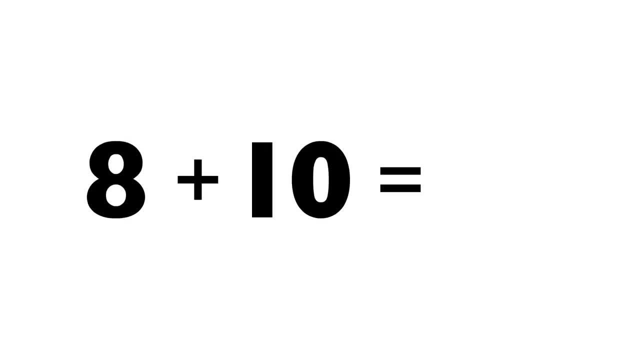 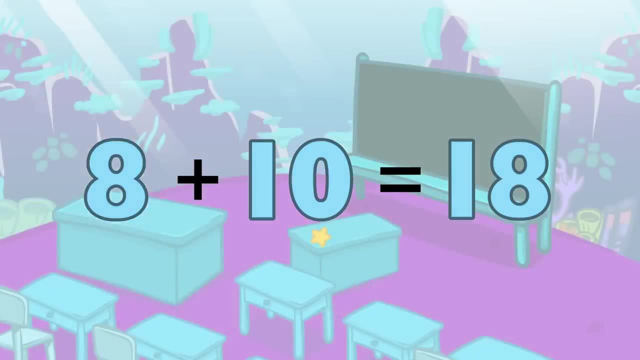 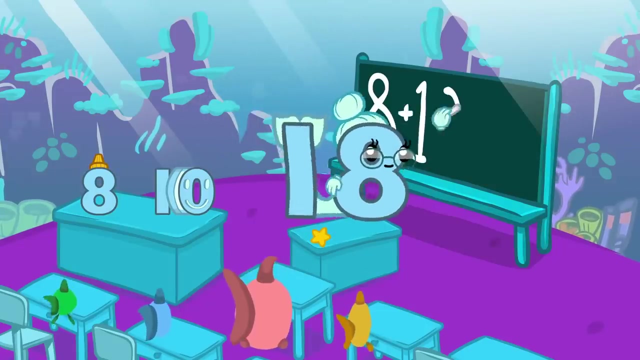 equals 10 plus 10, equals 8 plus 10, and 8 plus 10 equals 18, 8 plus 10. and 18, 8 plus 10 equals 10, equals 18 in in the in in in in in 9, 10. 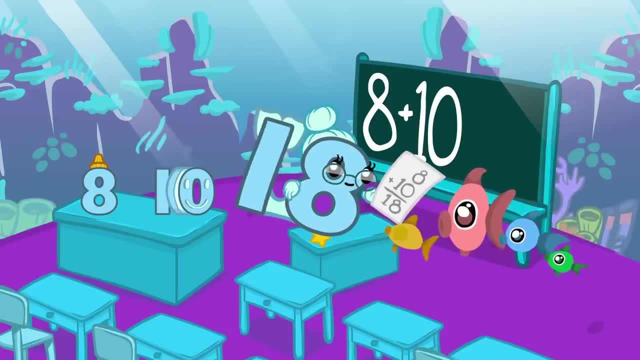 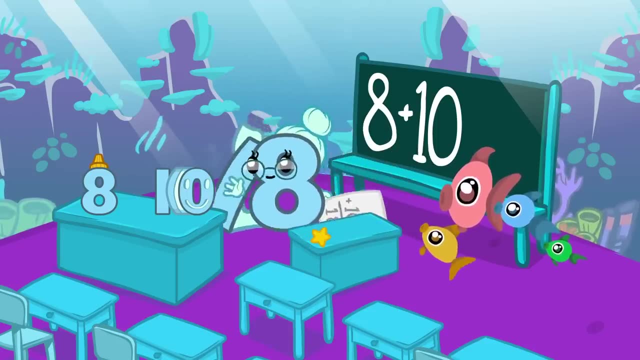 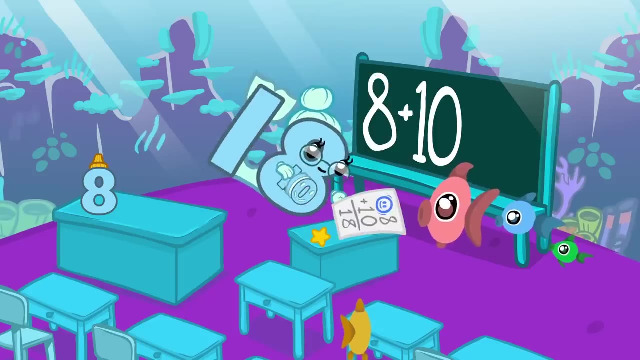 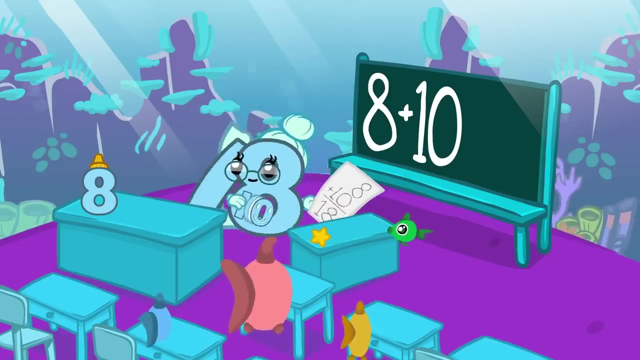 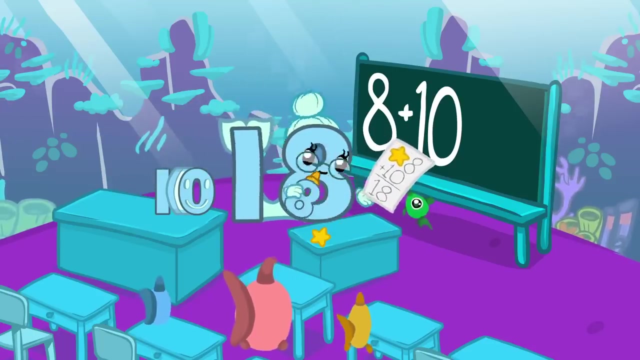 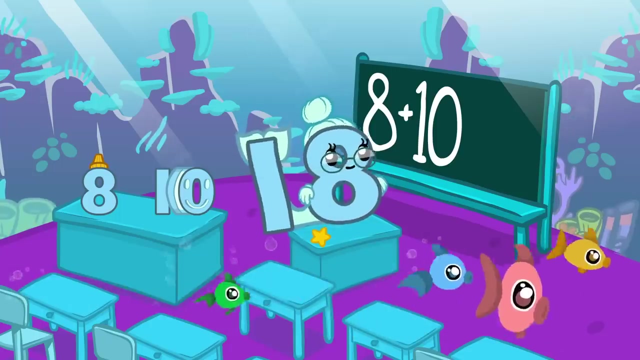 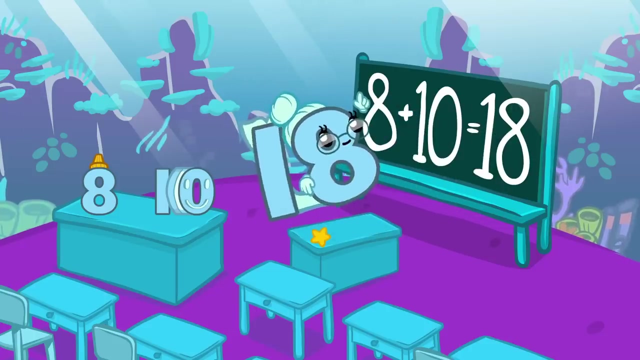 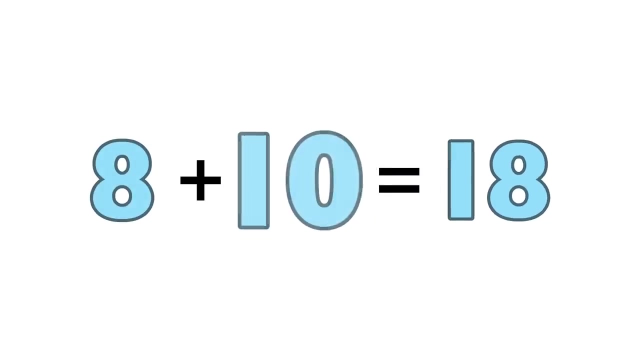 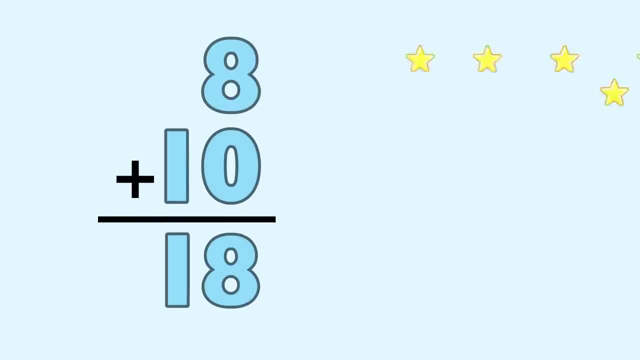 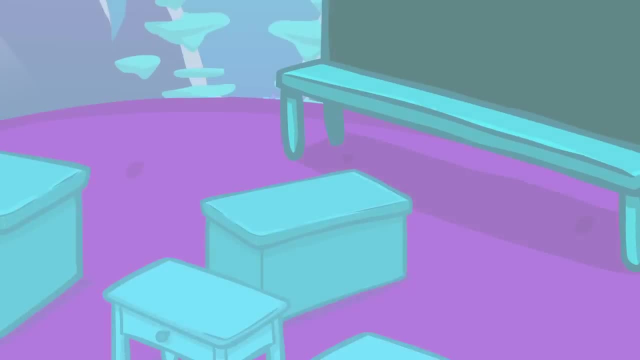 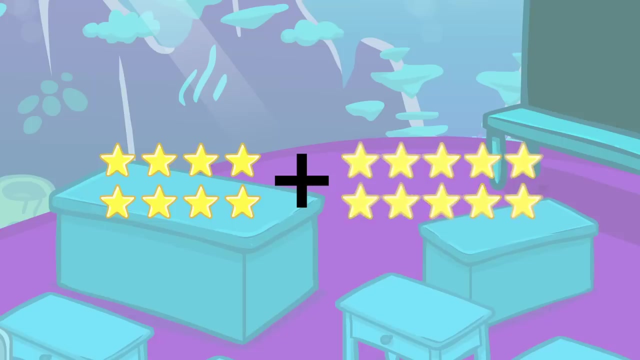 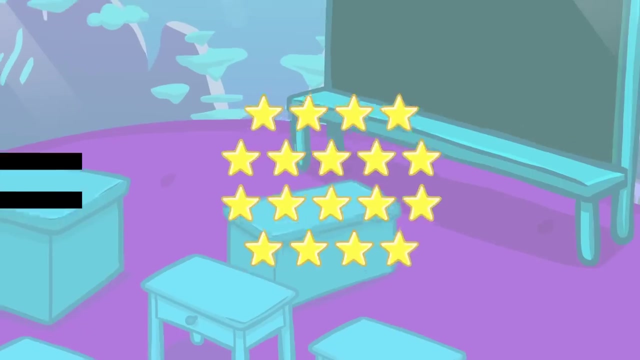 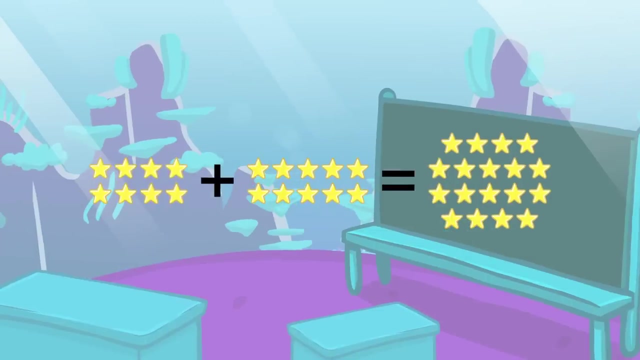 8 plus 10 equals 18.. 1,, 2,, 3,, 4,, 5,, 6,, 7,, 8,, 9,, 10,, 11,, 12,, 13,, 14,, 15,, 16,, 17, 18 equals 1,, 2,, 3,, 4,, 5,, 6,, 7,, 8,, 9,, 10,, 11,, 12,, 13,, 14,, 15,, 16,, 17,, 18.. 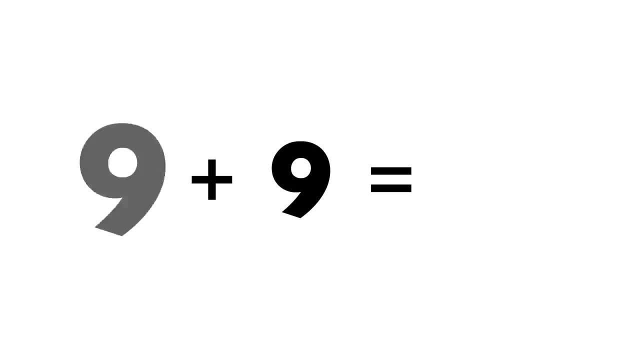 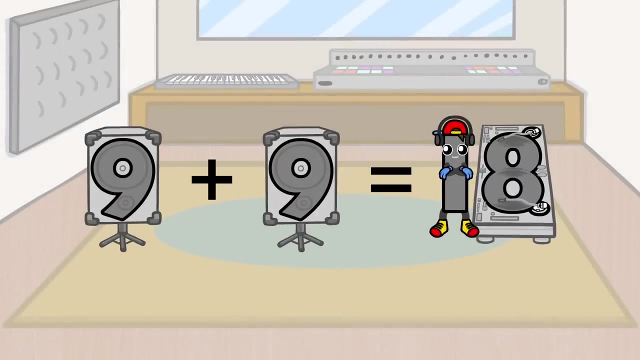 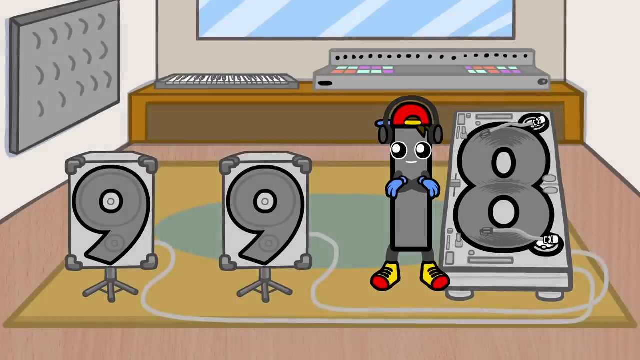 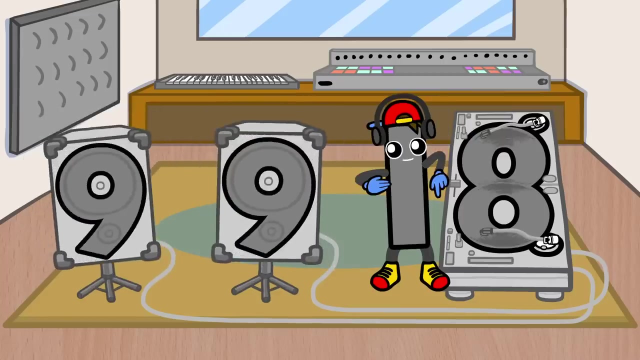 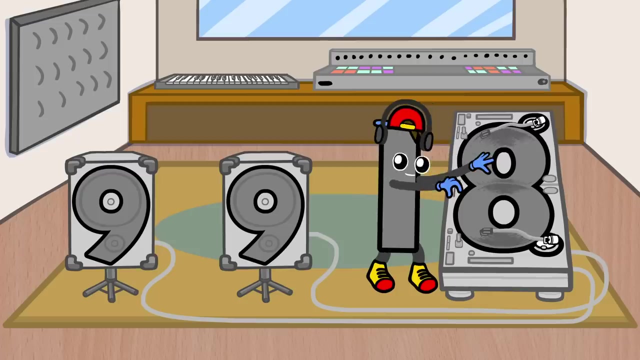 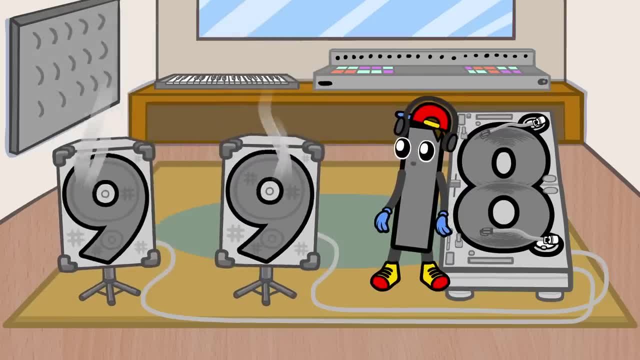 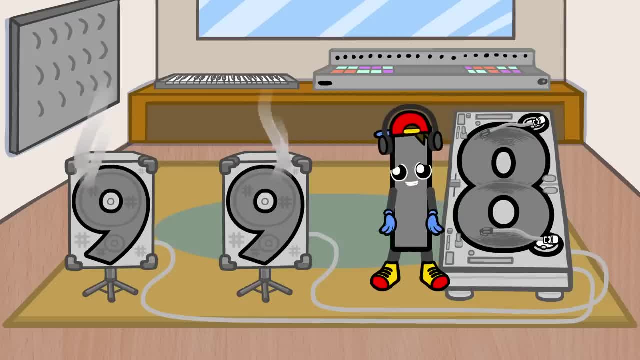 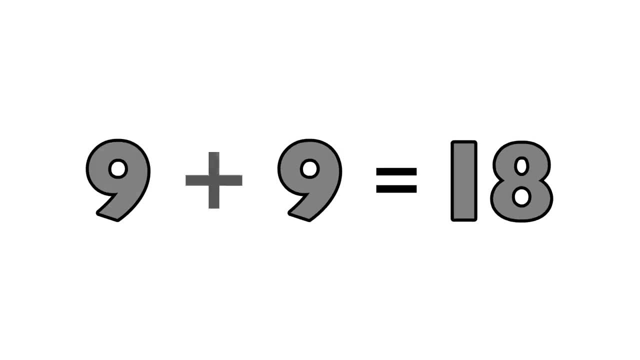 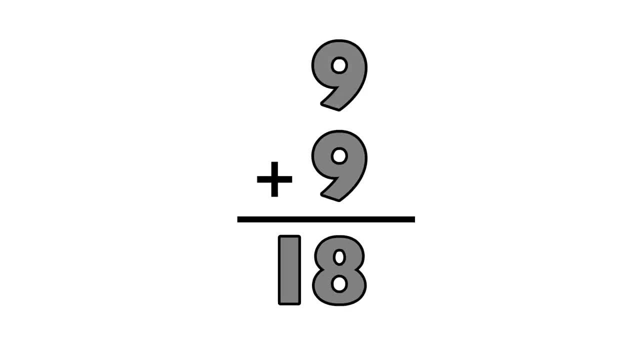 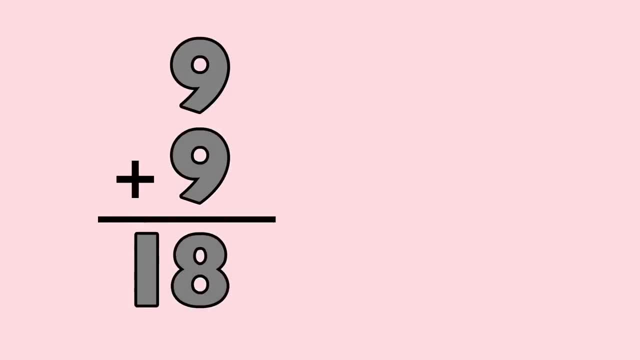 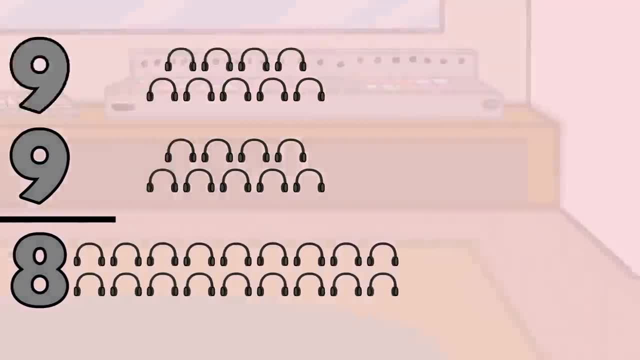 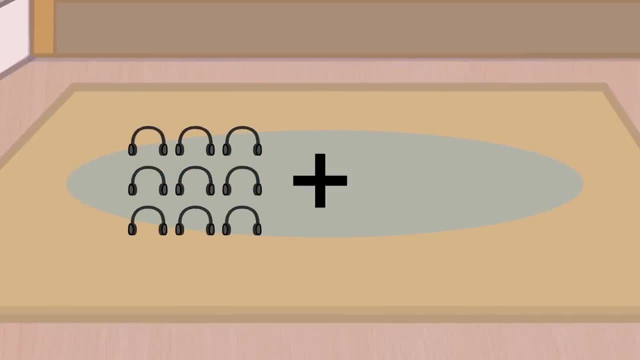 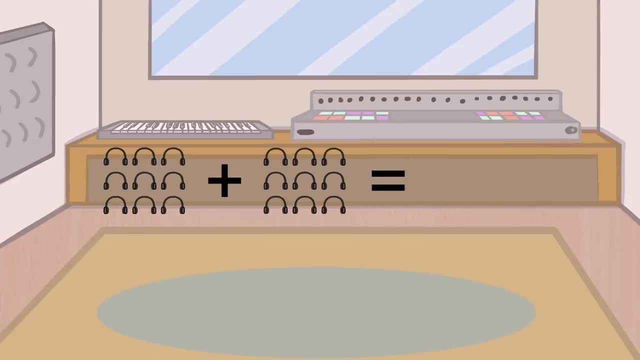 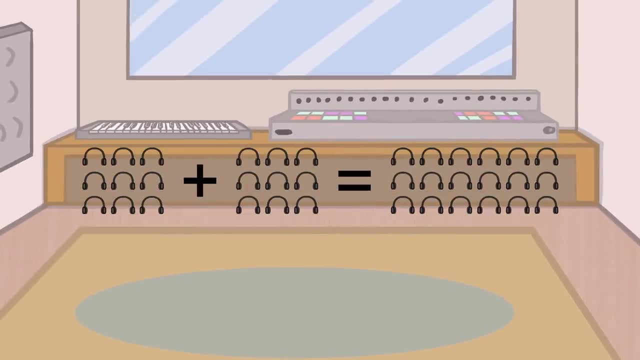 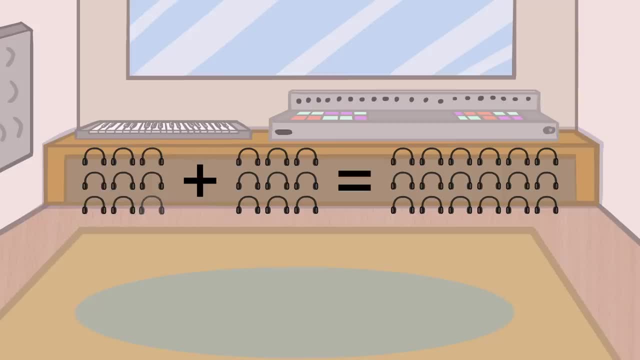 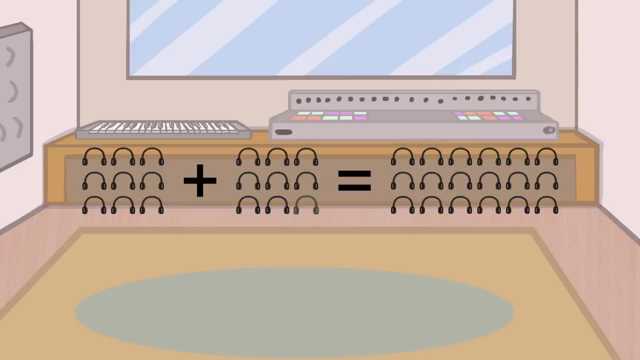 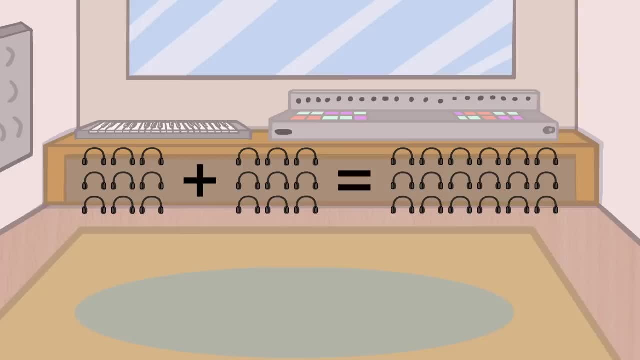 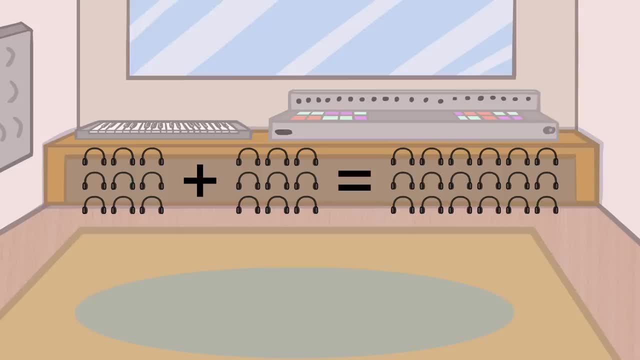 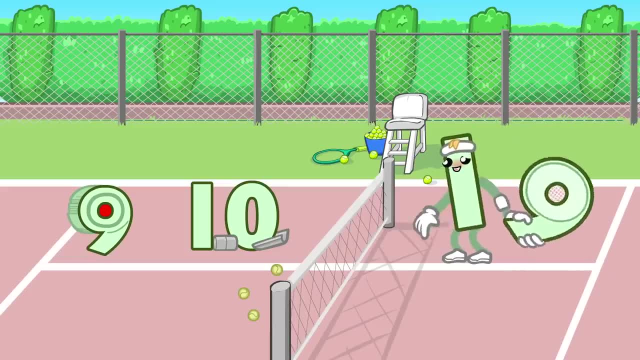 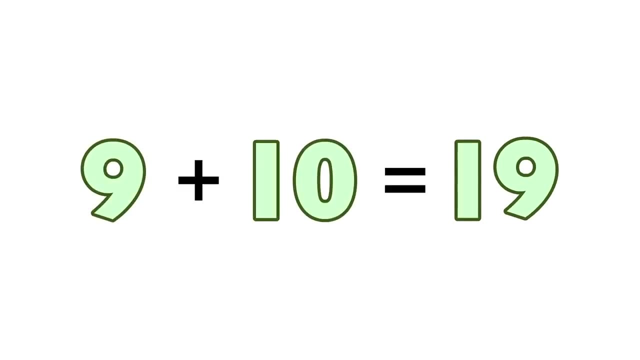 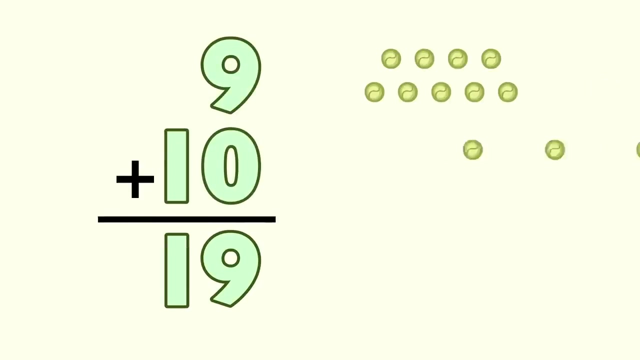 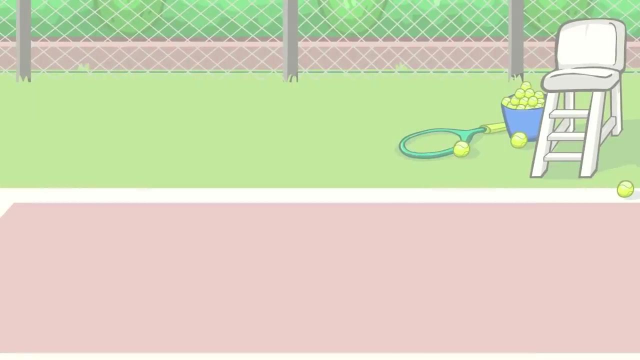 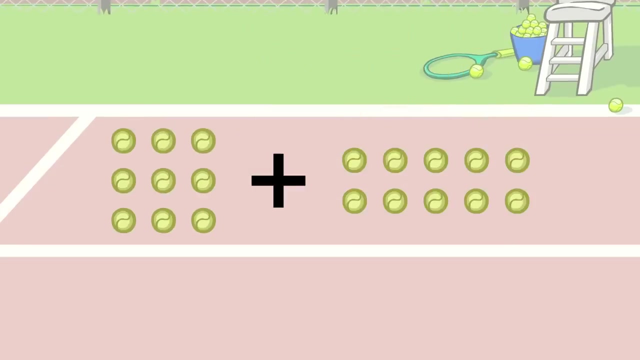 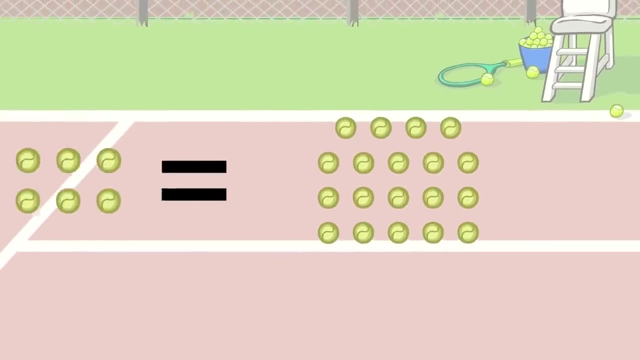 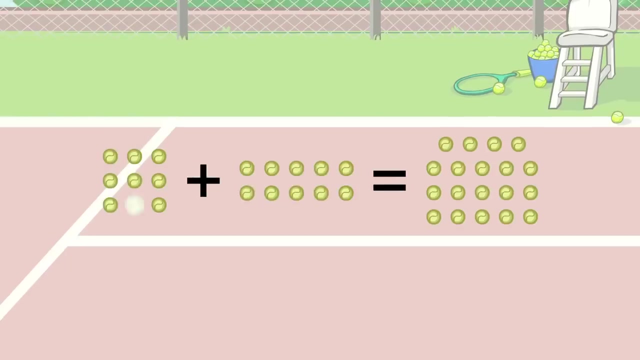 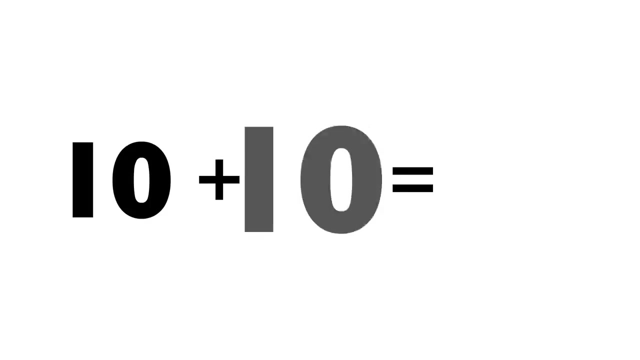 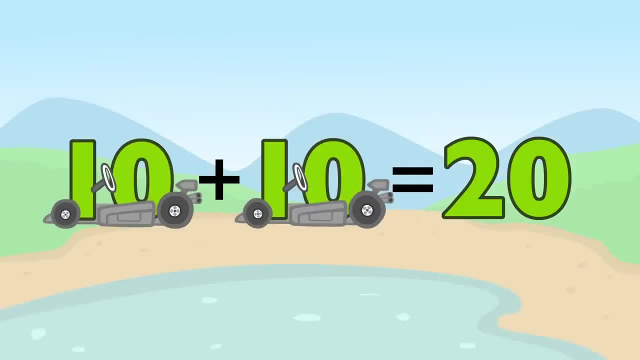 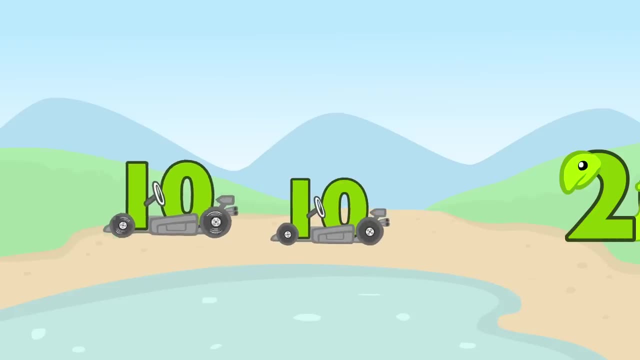 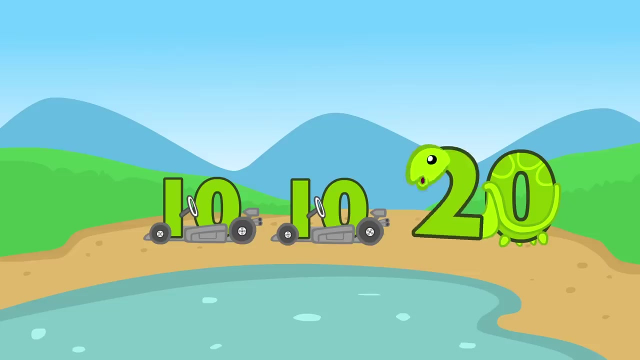 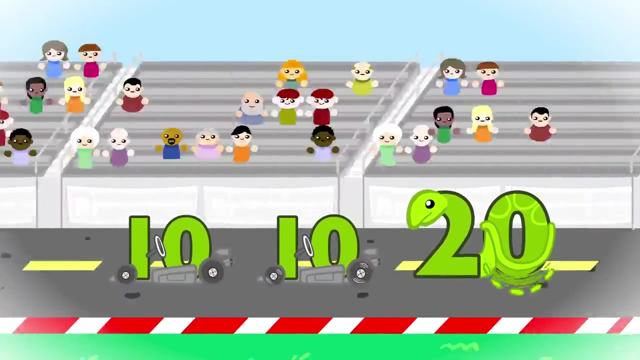 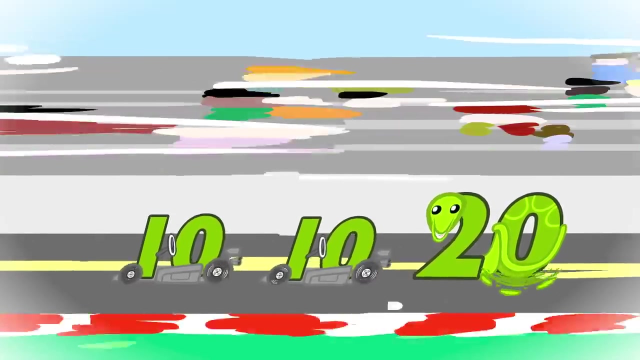 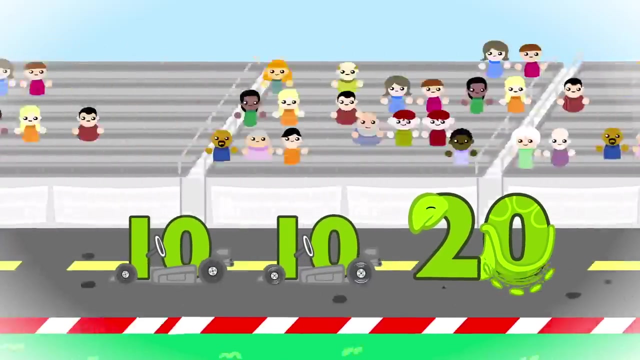 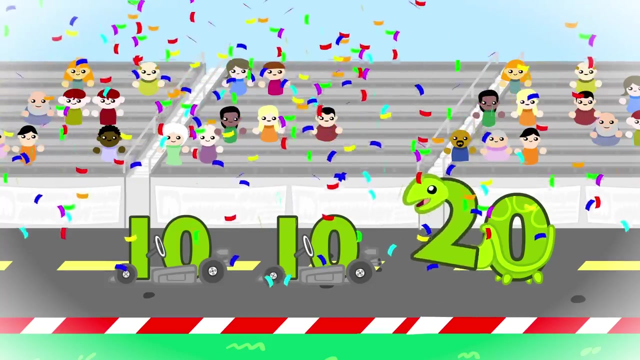 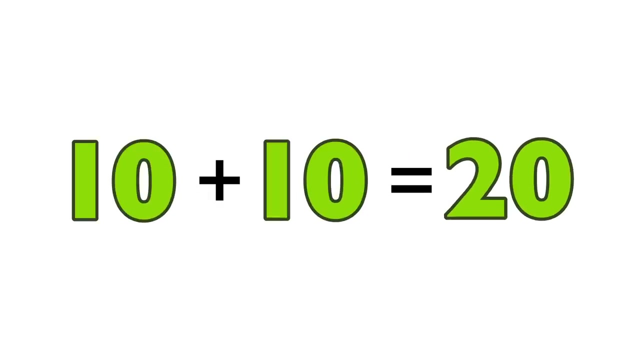 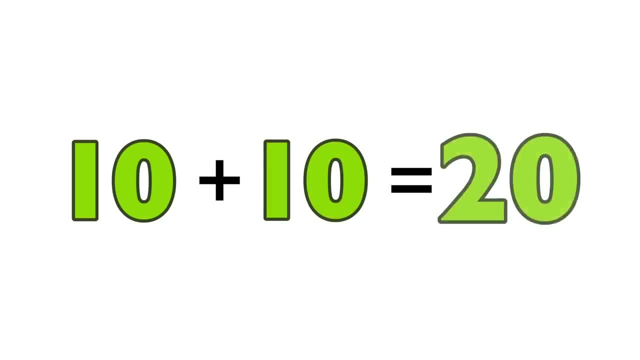 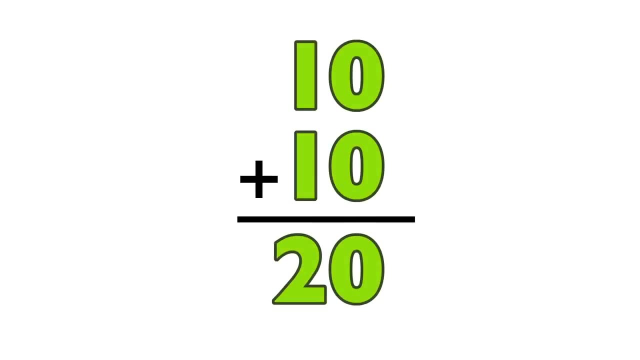 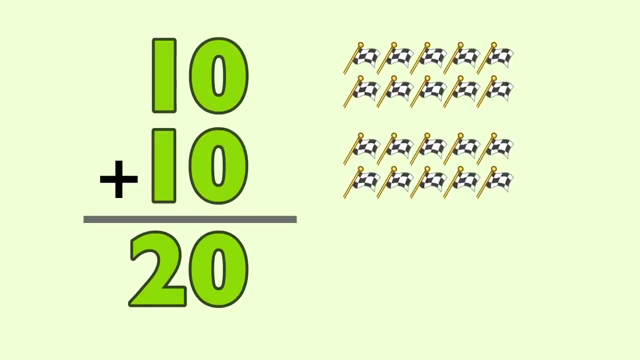 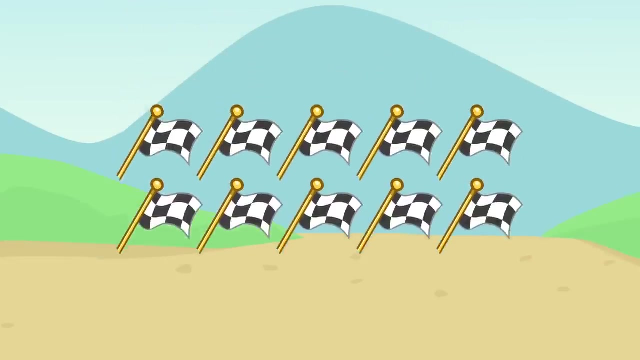 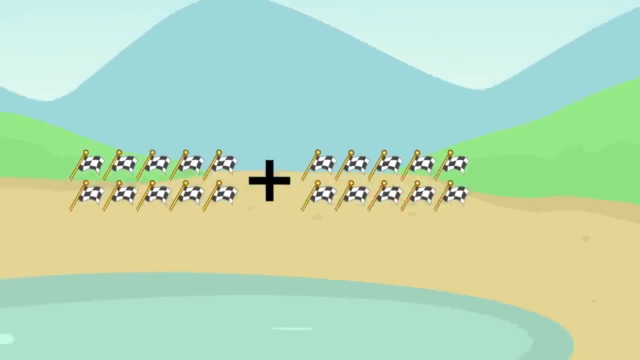 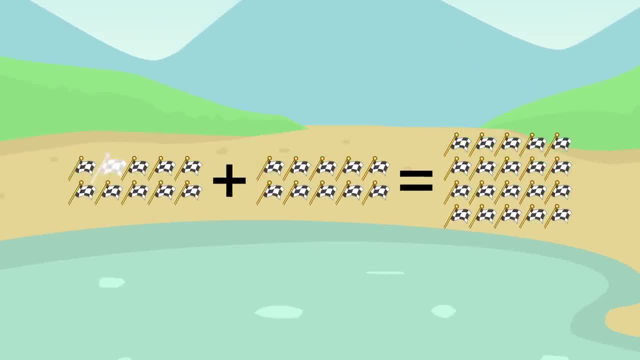 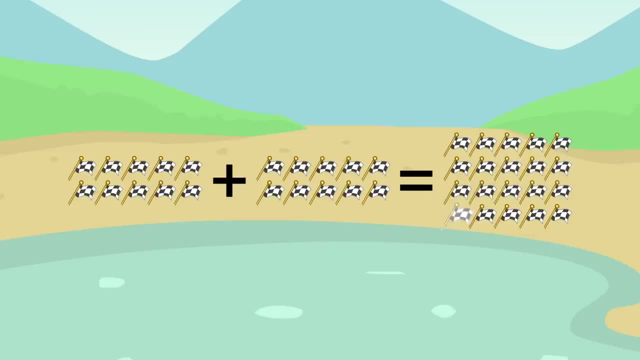 1,, 2,, 3,, 4,, 5,, 6,, 7,, 7,, 8,, 9,, 10,, 11,, 12,, 13,, 14,, 15,, 16,, 17,, 18,, 19,, 20.. 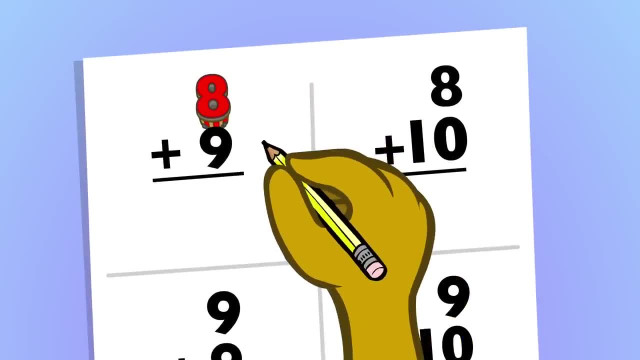 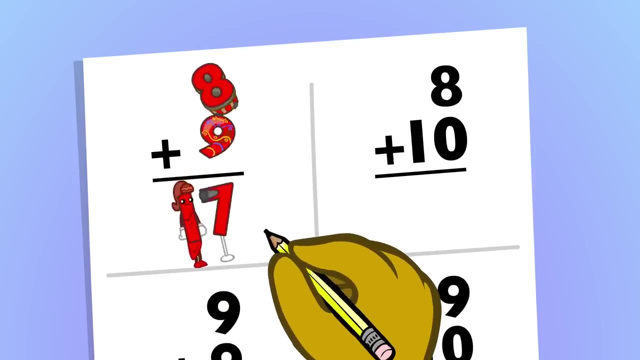 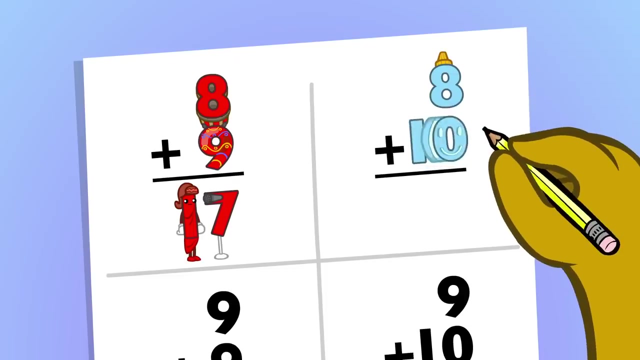 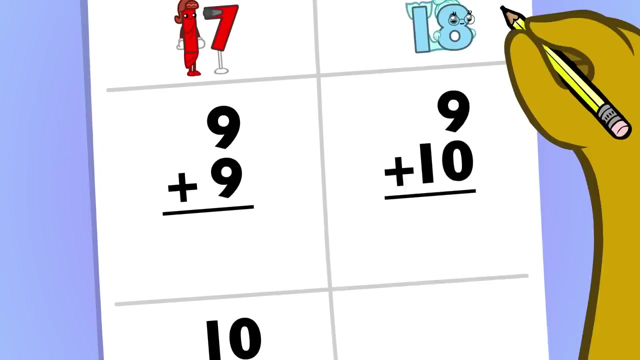 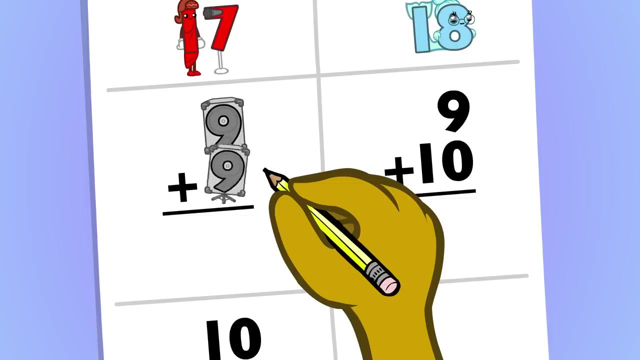 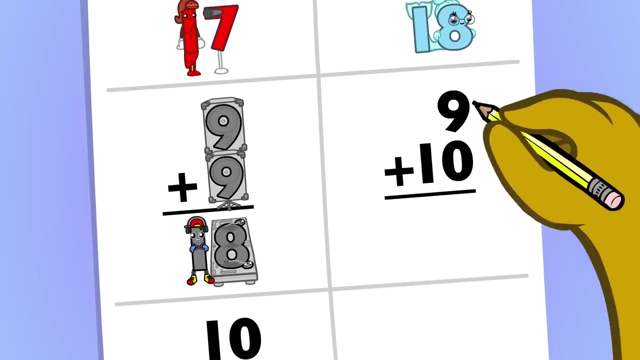 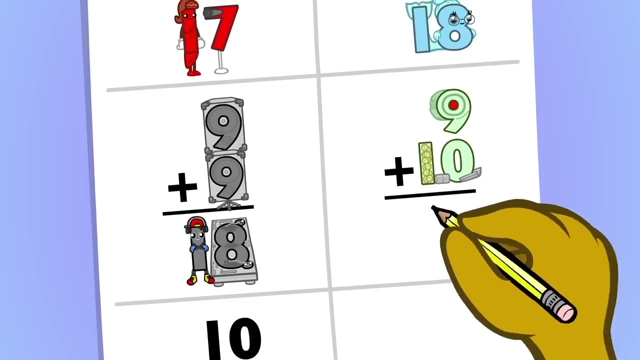 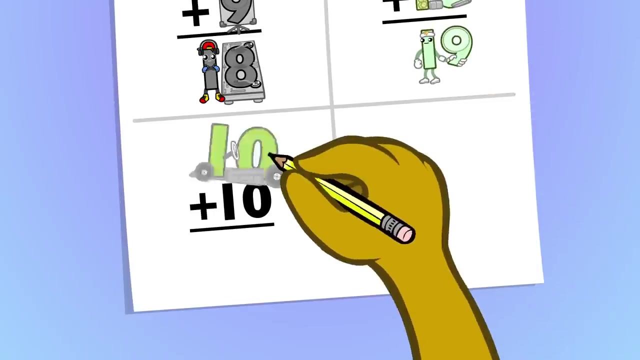 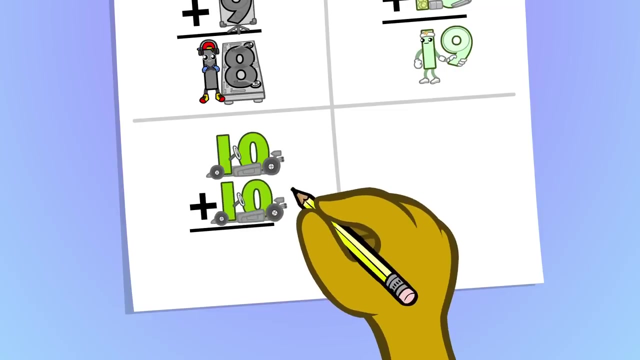 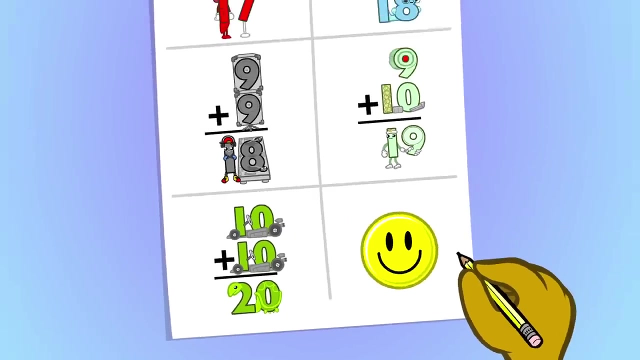 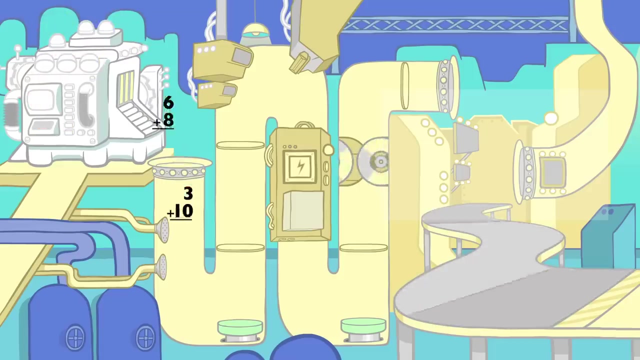 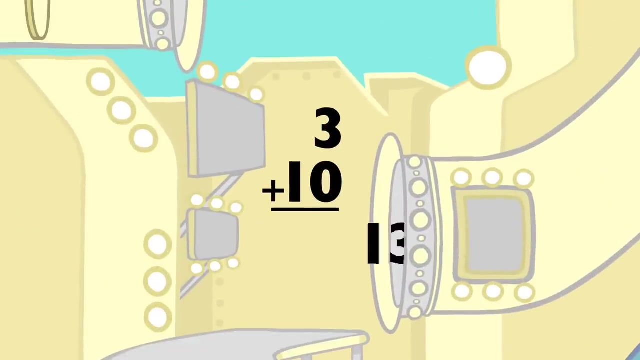 8 plus 9 equals Seventeen. eight plus ten equals eighteen. Nine plus nine equals eighteen. Eighteen nine plus ten equals eighteen. Nineteen ten plus ten equals nineteen. Ten plus ten equals nineteen. Twenty Three plus ten equals thirteen. 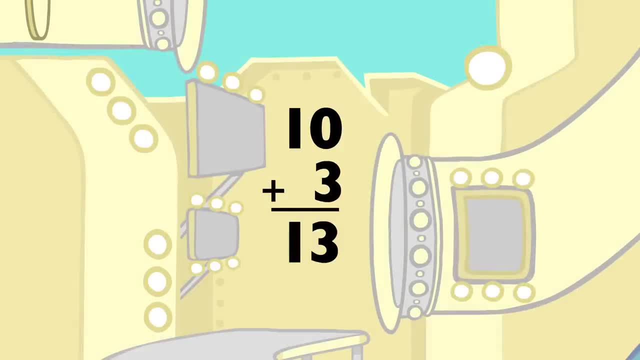 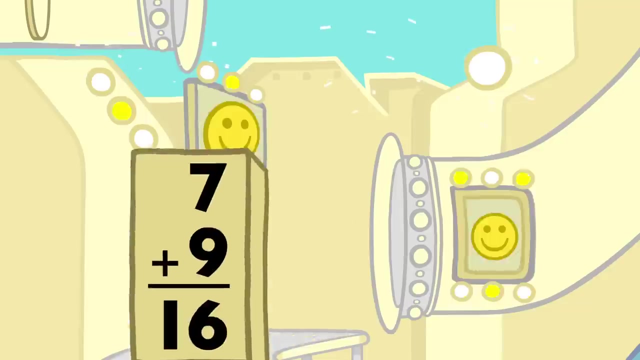 And ten plus three equals thirteen. Six plus eight equals fourteen. And eight plus six equals fourteen. Six plus nine equals fifteen. Nine plus six equals fifteen. Six plus ten equals sixteen. Ten plus six equals sixteen. Seven plus nine equals sixteen. Nine plus seven equals sixteen. 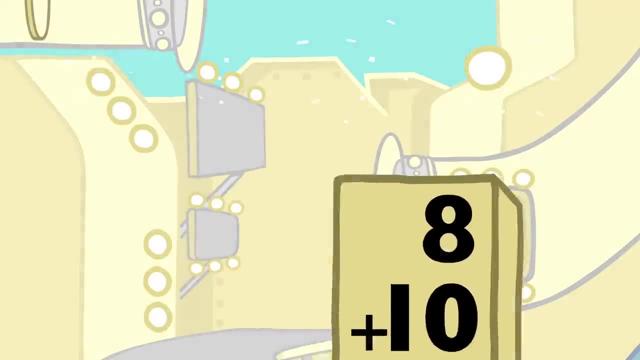 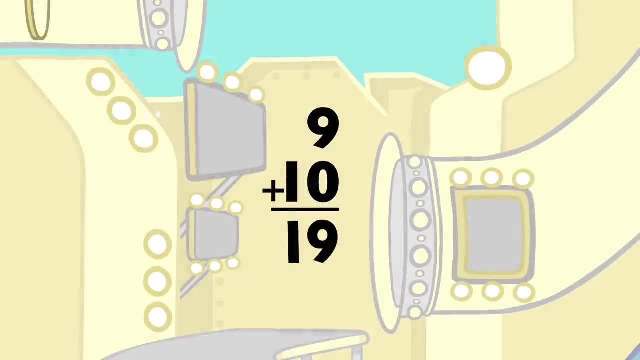 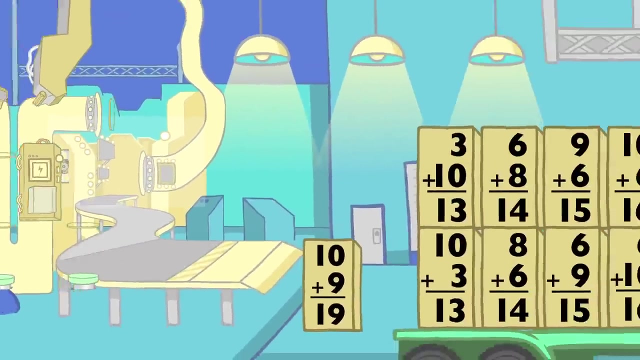 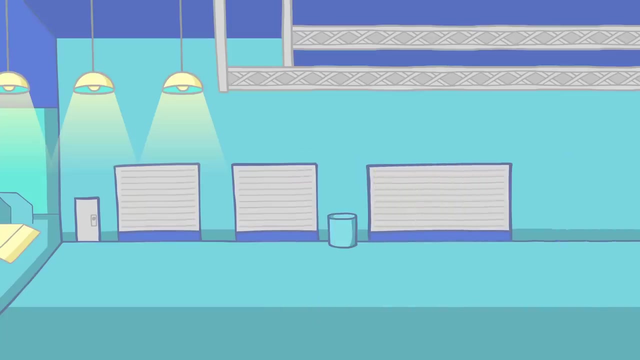 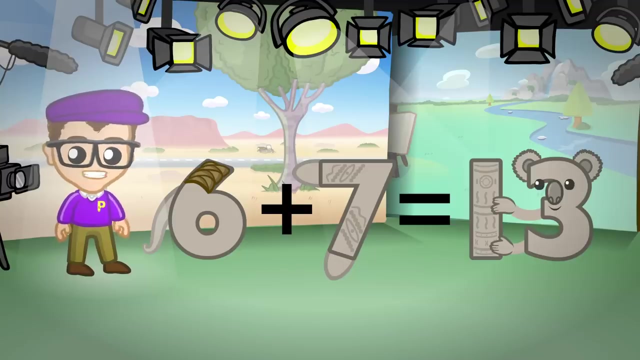 Eight plus ten equals eighteen. Ten plus eight equals eighteen. Nine plus ten equals nineteen, 19. 10 plus 9 equals 19. Now that you've learned the math facts, did you know you can use them for subtraction? It's easy. I'll show you how. 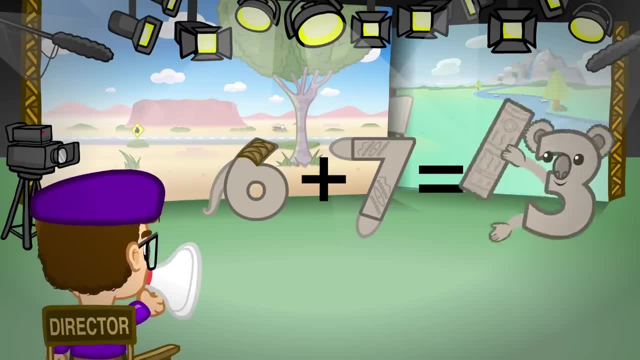 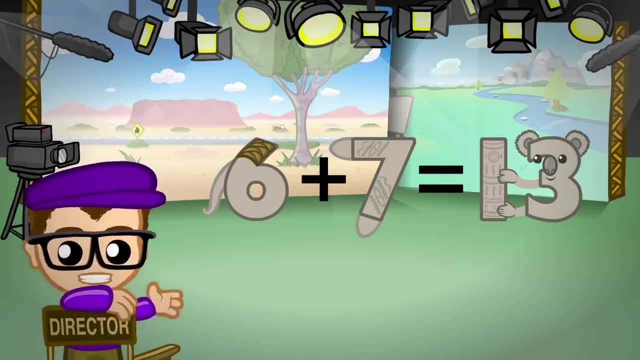 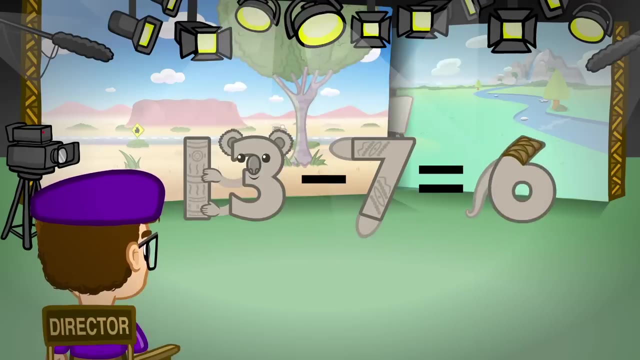 With the largest number. please step forward. great. Now we just move the largest number to the beginning And action: 13 minus 7 equals 6 And 13 minus 6 equals 7. Cut Next group. please would 7, 9 and 16 take the stage. 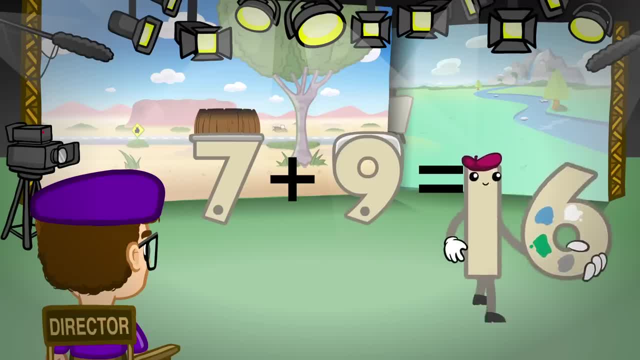 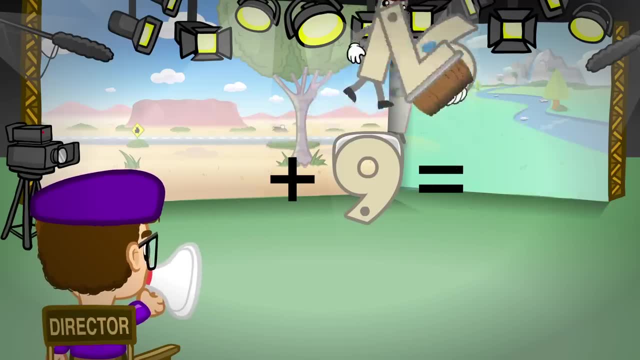 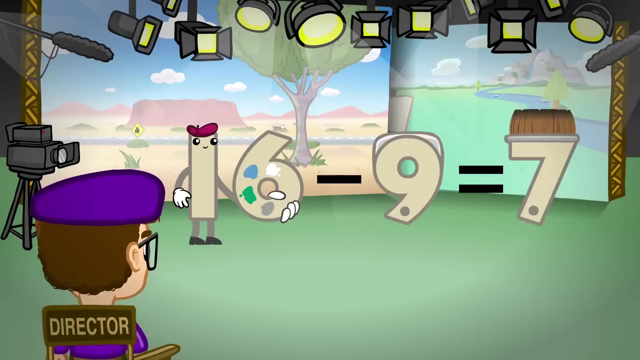 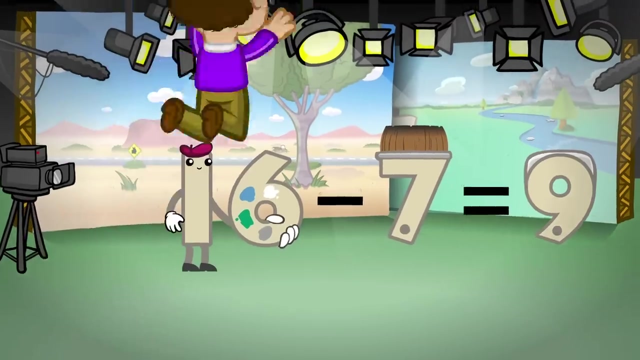 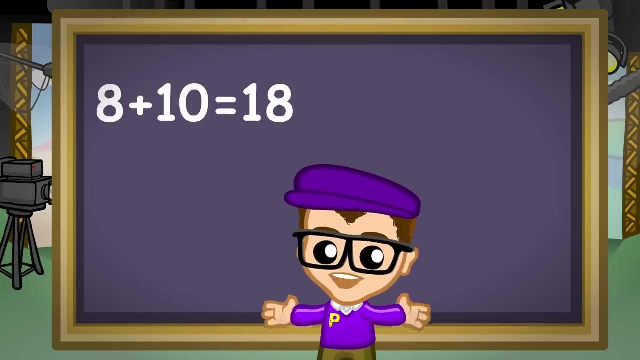 With the largest number. please step forward. Great, Okay, biggest number. please move to the beginning. 16 minus 9 equals 7, and 16 minus 7 equals 9. Now you try a few: 8 plus 10 equals 18. So 18 minus 10 equals. 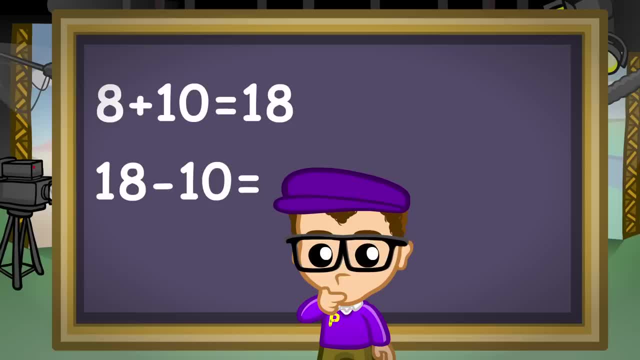 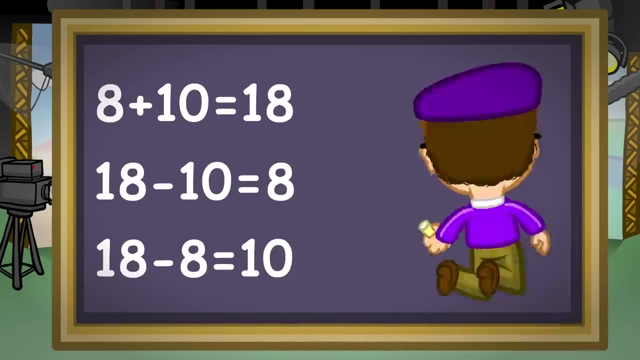 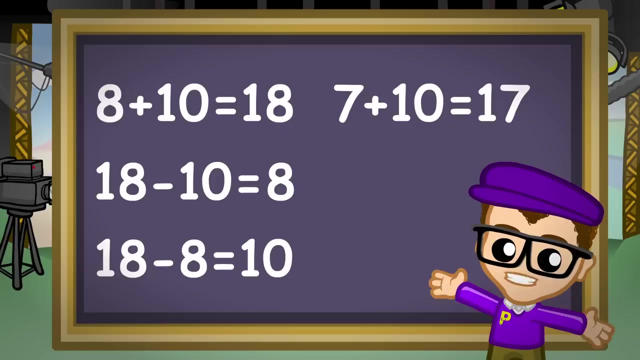 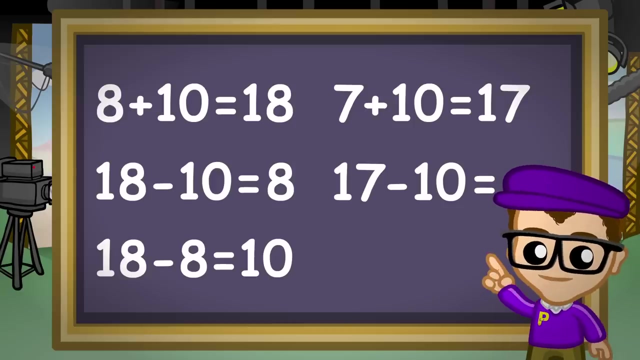 18 minus 10 equals 8, Right 8, And 18 minus 8 equals 10. That's right 10. Let's try another. 7 plus 10 equals 17. So 17 minus 10 equals 7 Right, And 17 minus 7 equals 10. 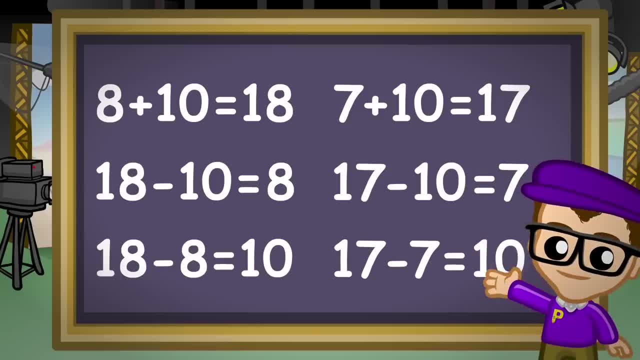 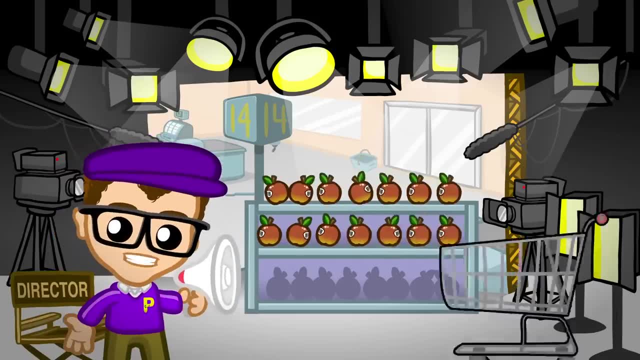 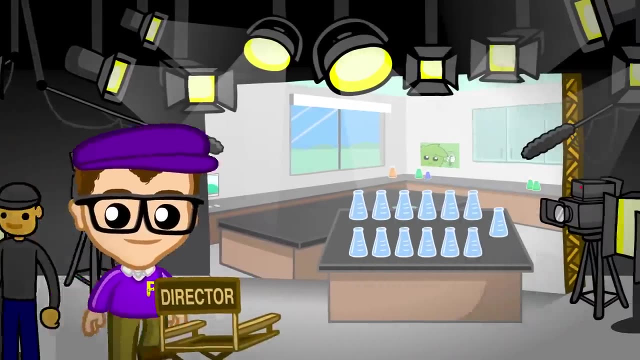 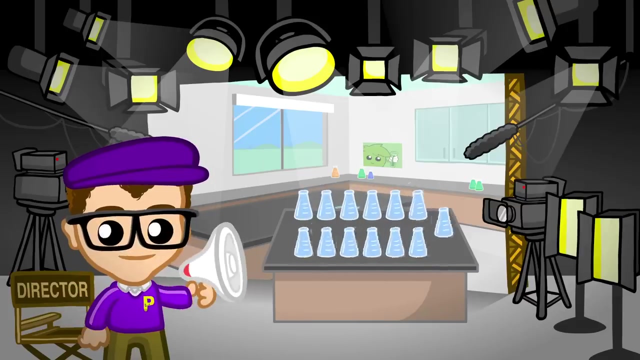 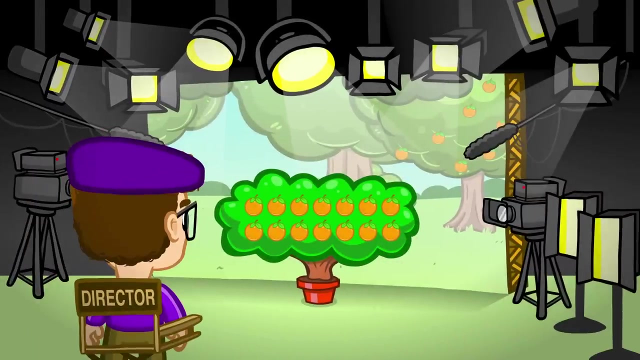 And 17 minus 7 equals 10. Right Right: 14 minus 9 equals 5. Right: 13 minus 7 equals 10, equals 19. 14 minus 10 equals 10, equals 15. 13 minus 8 equals 5 And 14 minus 9 equals 1. 11 minus 9 equals 9, equals 10. That's right. Then let us go to the next group: 13 minus 8 equals 8. 16 minus 10 equals 6. 15 minus 10 equals 5. 19 minus 9 equals 10. 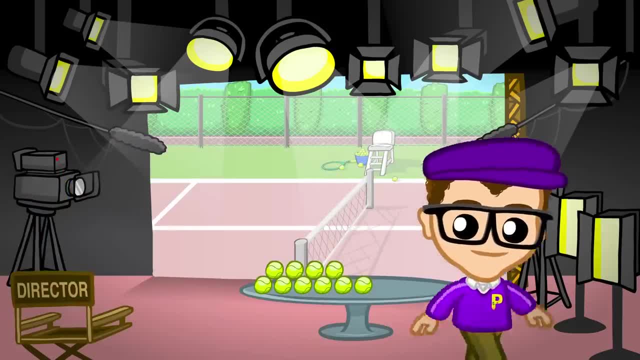 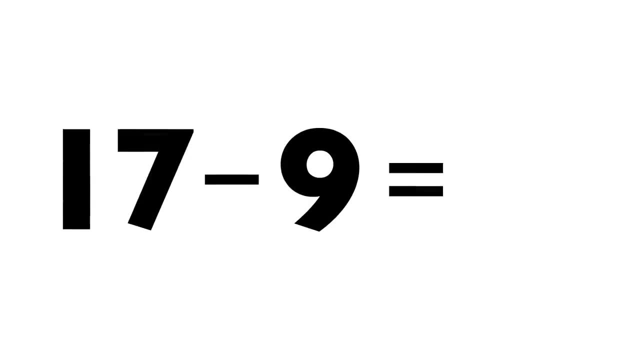 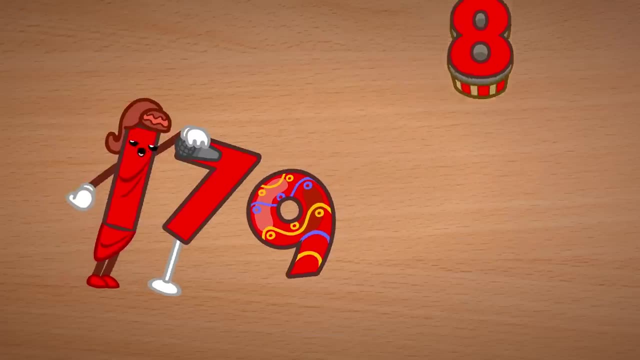 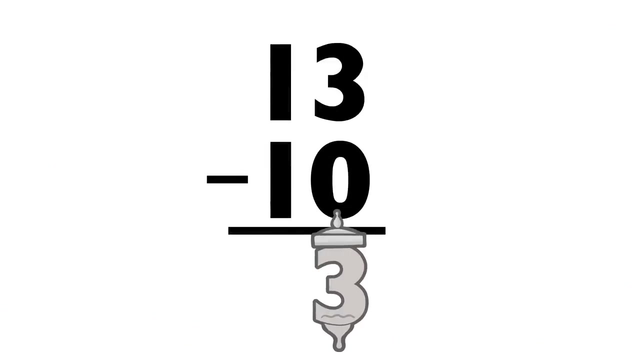 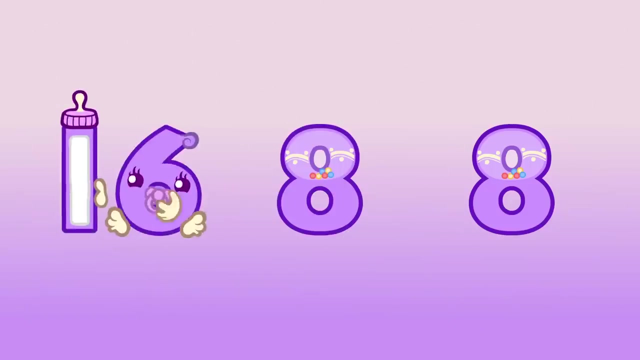 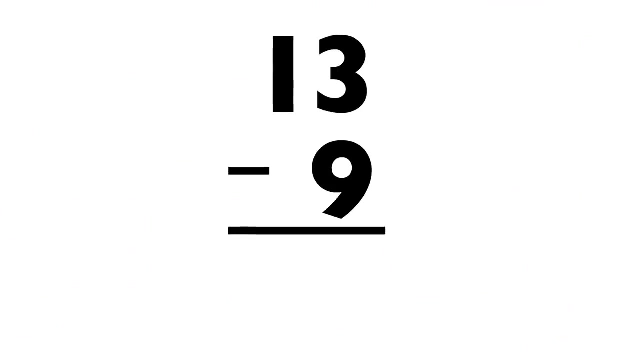 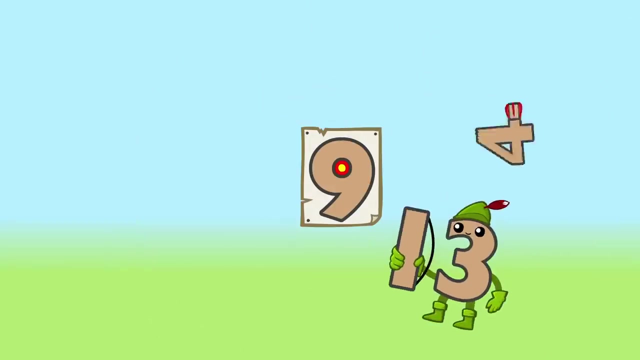 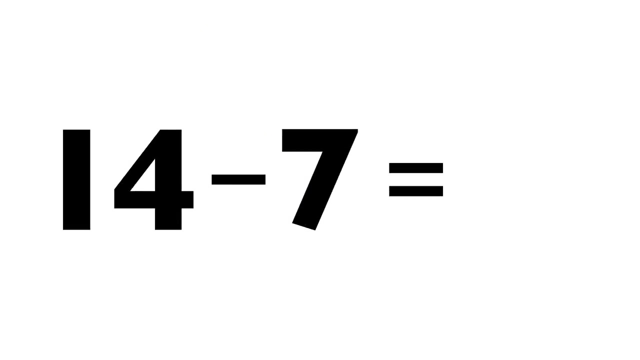 17 minus 9 equals 8. 13 minus 9 equals 8. 13 minus 9 equals 8 Minus 10: equals 3. 16 minus 8 equals 8. 13 minus 9: equals 4. 14 minus 7: equals 7. 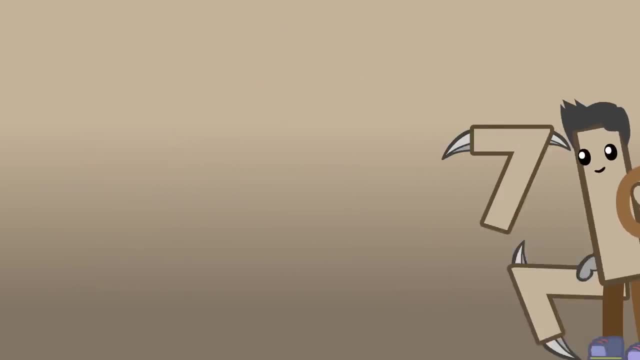 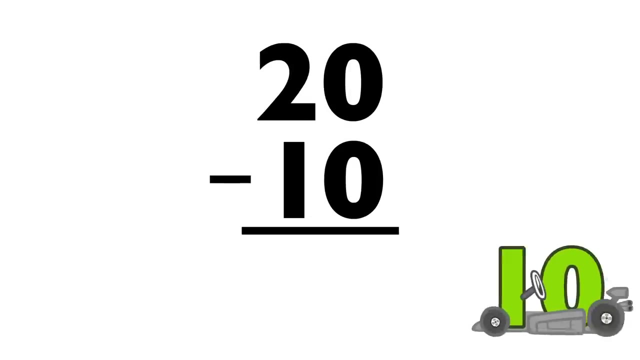 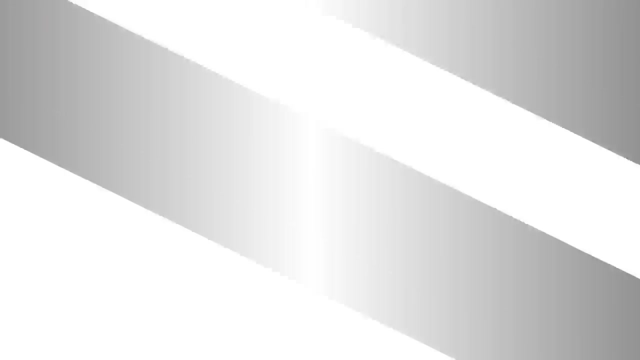 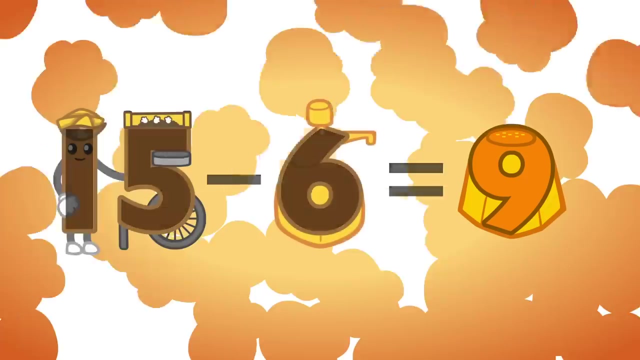 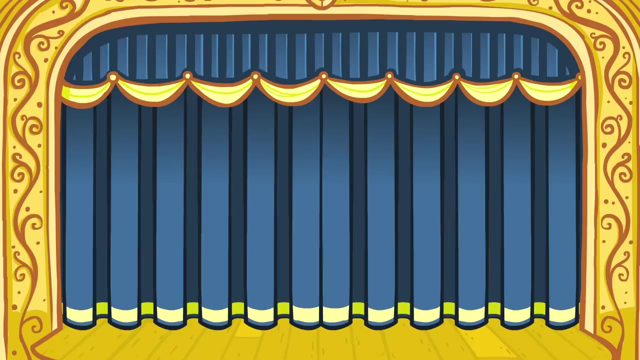 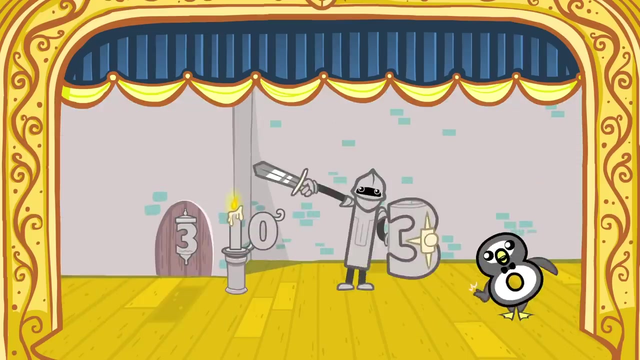 20 minus 10 equals 10. 15 minus 9 equals 10. 19 minus 6 equals 9. Ladies and gentlemen, please give a round of applause to Meet the Math Facts: 3 plus 10 equals 13. 4 plus 9 equals 13. 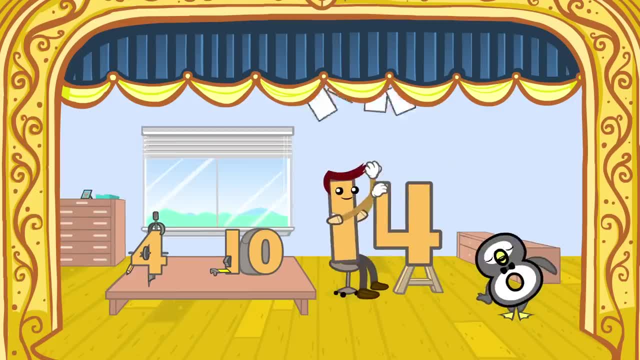 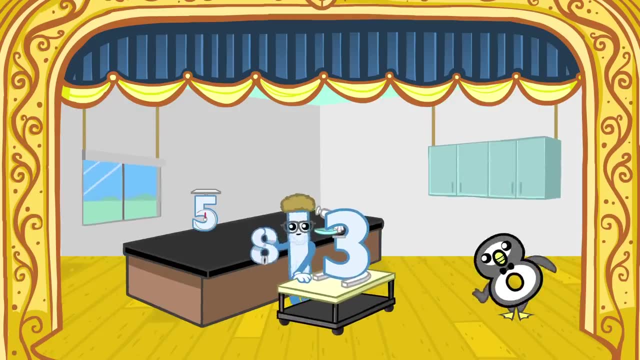 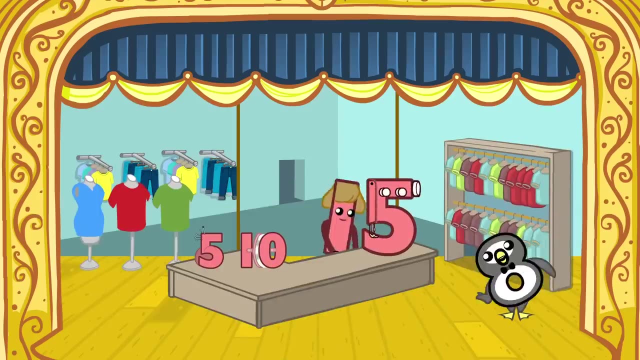 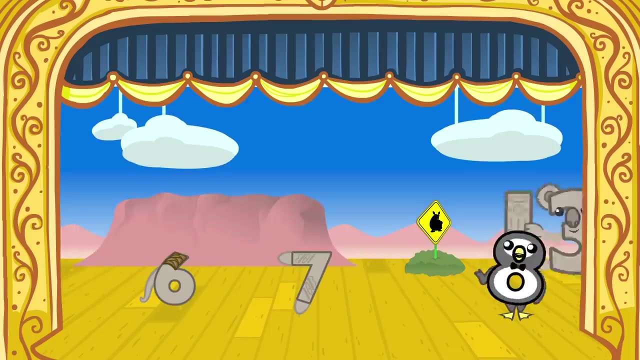 4 plus 10 equals 14. 5 plus 8 equals 13. 5 plus 9 equals 14. 5 plus 10 equals 15. 6 plus 7 equals 13. 6 plus 8 equals 14. 4 plus 10 equals 14. 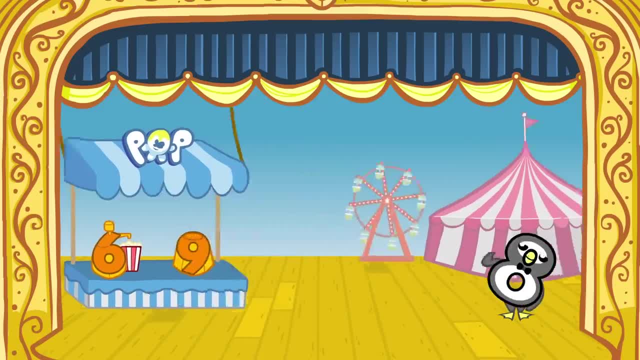 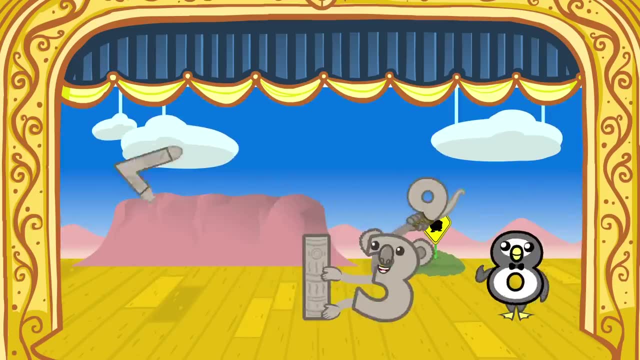 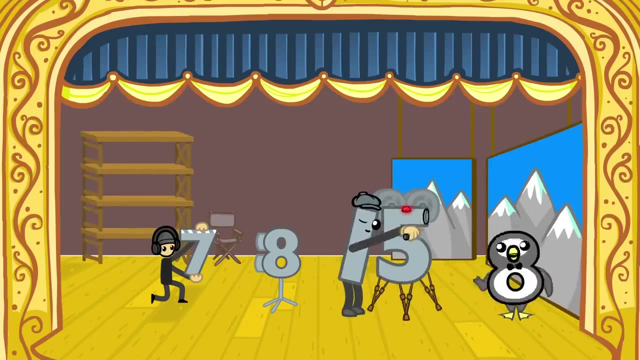 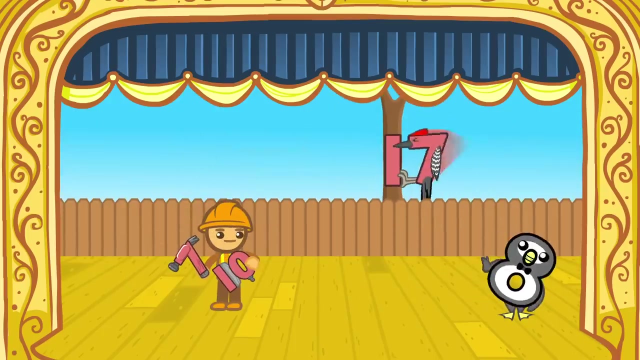 6 plus 9 equals 15,. 6 plus 10 equals 16,. 7 plus 6 equals 13,. 7 plus 7 equals 14,. 7 plus 8 equals 15,. 7 plus 9 equals 16,. 7 plus 10 equals 17.. 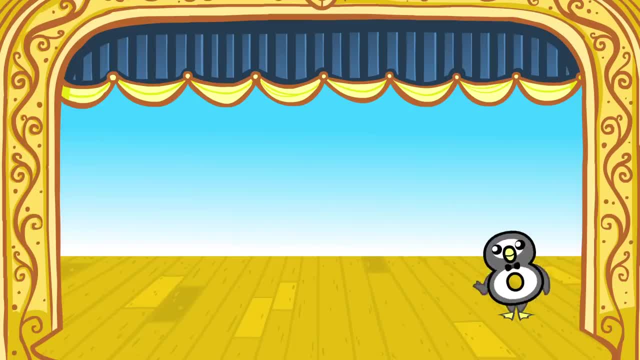 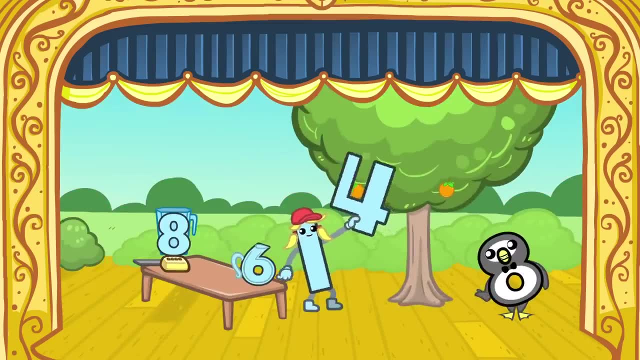 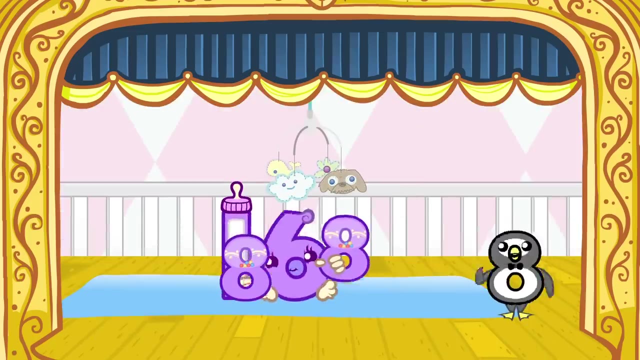 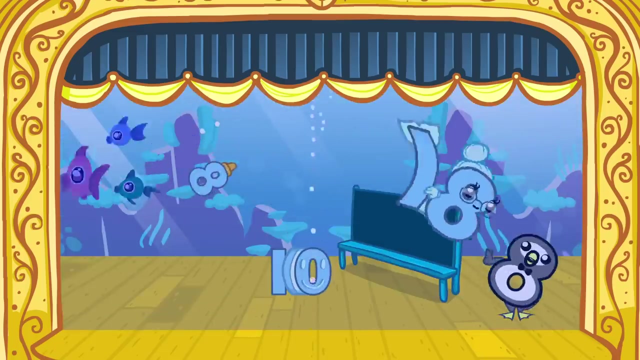 8 plus 5 equals 13,. 8 plus 6 equals 14,. 8 plus 7 equals 15,. 8 plus 8 equals 16,. 8 plus 9 equals 17,. 8 plus 10 equals 18,. 9 plus 4 equals 13.. 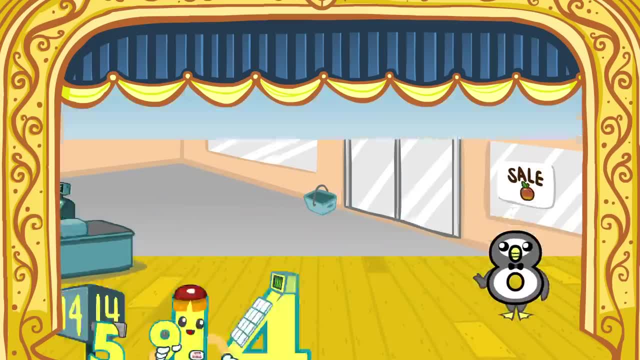 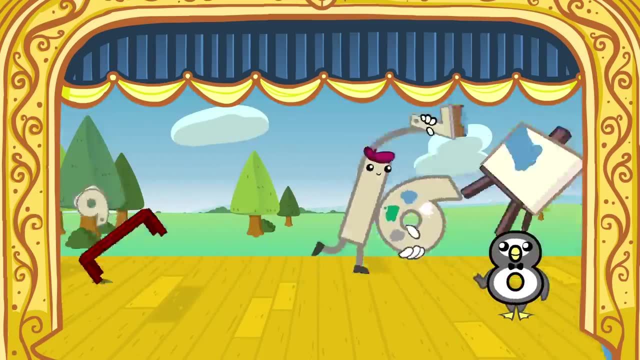 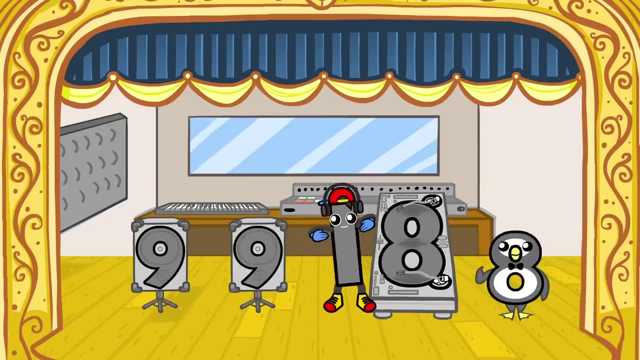 9 plus 5 equals 14,. 9 plus 6 equals 15,. 9 plus 7 equals 16,. 9 plus 8 equals 17,. 9 plus 9 equals 18,. 9 plus 10 equals 19,.